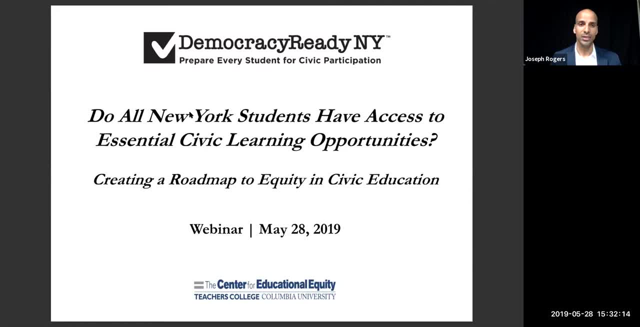 and exciting conversation- certainly a timely one- on whether New York students- all New York students- have access to the civic learning opportunities that they need and to which they're going to be able to access. So I'm going to start with Joe Rogers. 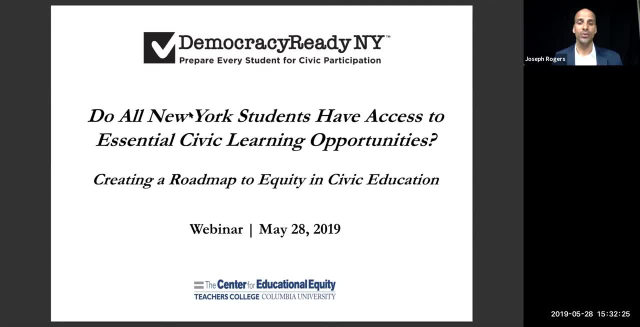 I'm going to give you some background information on the constitutional right to civic preparation. You're going to hear from a few stakeholders selected by coalition member organizations and they're going to tell you a little bit about what the findings from this recent report that the Center for Educational Equity wrote, based on a pilot study, mean to them. 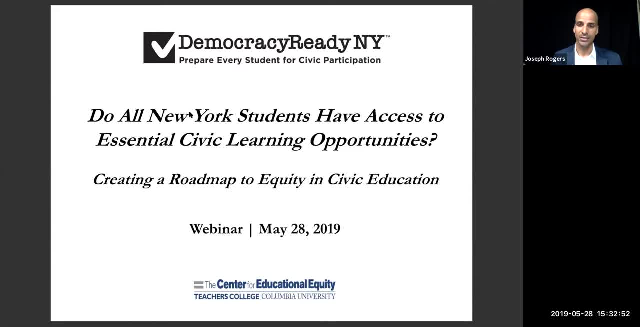 as students, as parents and as students. So I'm going to start with Joe Rogers. So Joe Rogers started with us. a first: You're going to hear from a few stakeholders selected by coalition member organizations. You're going to hear from a few stakeholders selected by coalition member organizations. 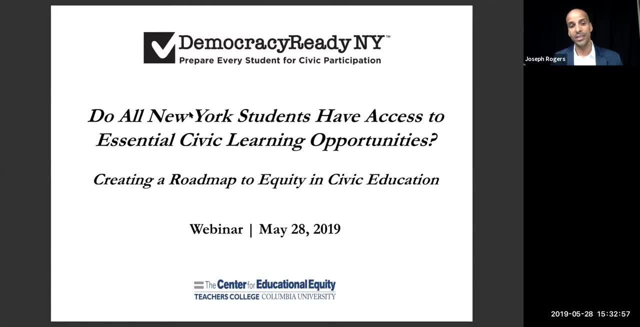 as youth development organization representatives, as teachers and as school board association representatives. So that's just to give you a sense of where we're headed. After you hear from our featured education stakeholders, we're going to then open up the conversation, And we hope that. 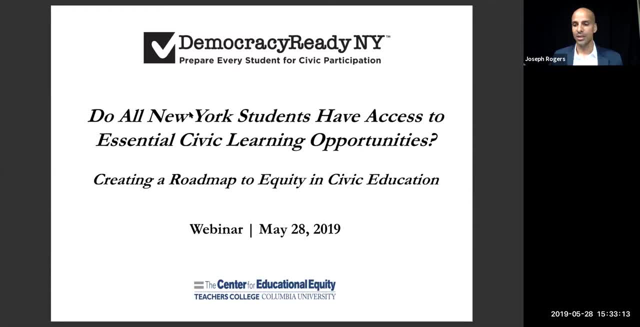 you will engage and add your thoughts and questions toward guiding the Democracy Ready New York Coalition's work in the coming months and years toward ensuring that all students will have the opportunity to participate in the work that they're doing. So, Joe, you're going to start off with Joe Rogers. 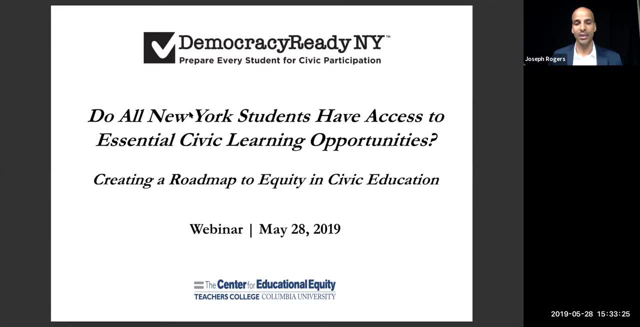 Thank you, receive the full range of civic learning opportunities that they need in order to participate in and shape our democracy. So we're going to then transition to our next slide. Okay, I've mentioned this is the Center for Educational Equity, Again, CEE, as you may know. 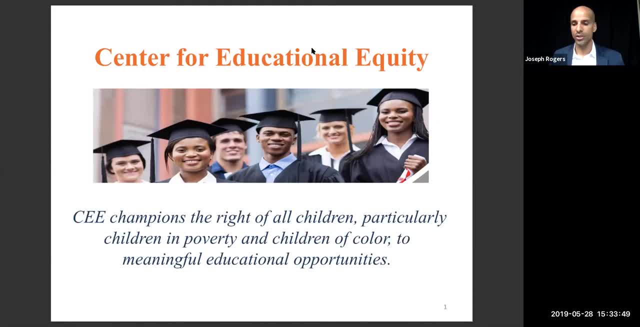 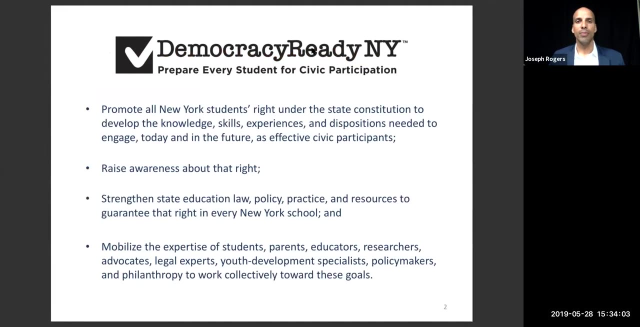 is a research and policy organization based at Teachers College, Columbia University, that works to ensure that the rights- the educational rights- of all students are honored and that students receive the meaningful, high-quality educational opportunities that they need in order to be successful. A little bit more about the Democracy Ready. 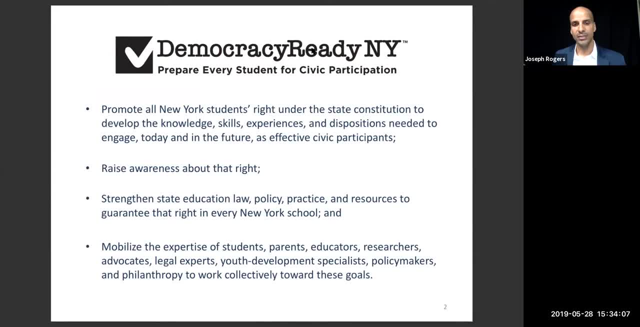 New York Coalition. Again, I mentioned that the stakeholders at the table who are guiding and driving the coalition's work fall into one of three buckets, and those are: school funding slash, educational equity, education advocacy groups, including the Center for Educational Equity. the Center for Educational Equity. 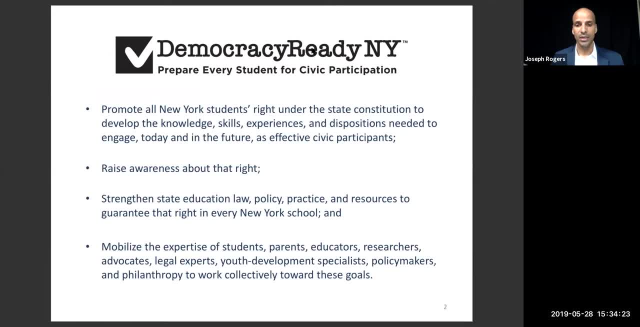 and the Center for Educational Equity, the Center for Educational Equity, the Center for Educational Equity, including several statewide organizations. You also have civic educators, and these include both school-based educators- these include education specialists and particularly social studies specialists- as well as non-profit organizations, many of whom partner with schools. 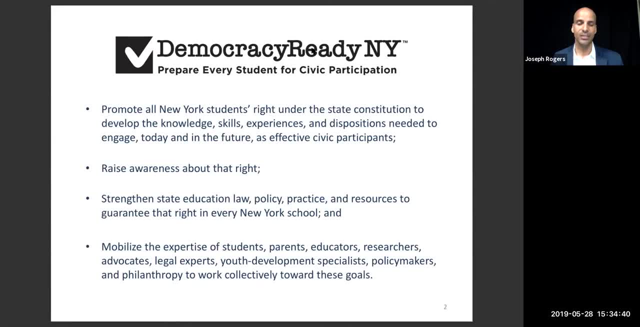 to provide civic education or civic learning services and supports. And, last but not least, you have good government groups- I'll call them- and those are groups that are trying to to provide civic education or civic learning services and supports. And those are groups that are trying to. 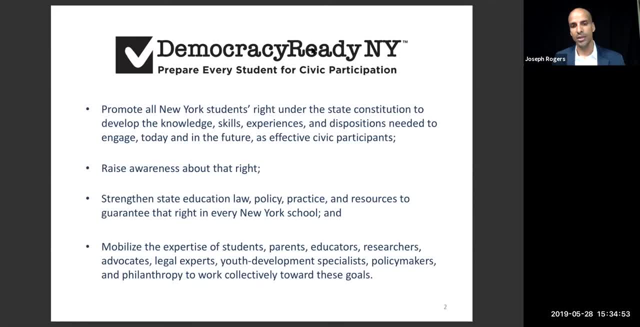 voters are well-informed about the options. they're staying abreast of candidates, political candidates and, ultimately, that those who are able in our state go to the polls. But, of course, civic participation, civic engagement doesn't stop with voting and we want to make sure that all 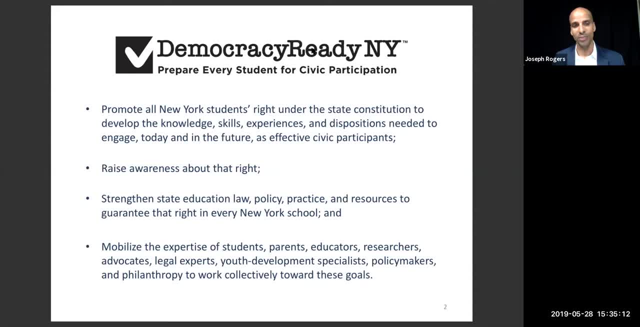 civic participants, all members of the New York family or New York community are able to participate in our democracy, whether that's at the local level, the state level or community level- I should have mentioned- or beyond, at the federal level, Some would say globally as well. 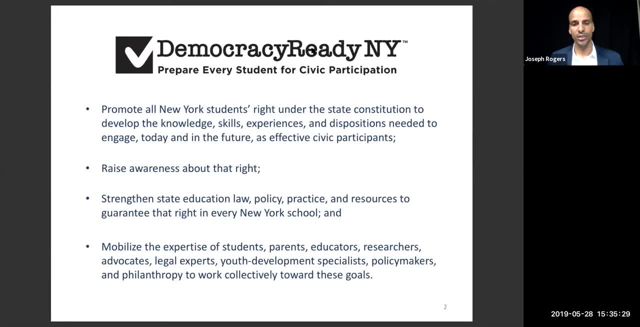 So just very quickly about the Democracy Ready New York Coalition. what you see on your screen now are the four elements, or four components of the coalition's mission, and those are, very simply, to promote all students' right under the Constitution to be prepared for civic participation. We'll say 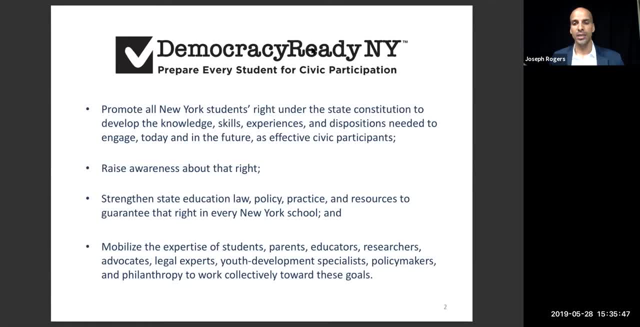 a little bit more about what the Constitution guarantees in a moment. The coalition is also raising awareness about that right. I'm sure many of you out there are unfamiliar with this specific constitutional guarantee to our children that they be prepared for civic participation. So we want to make sure all New 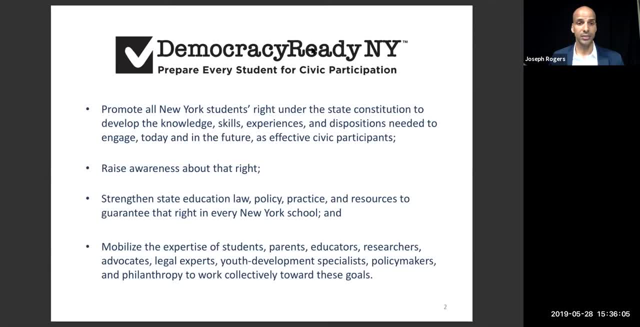 Yorkers are aware of what the Constitution guarantees. We want to strengthen state policy, strengthen the laws of policy, practice and resources that allow our schools to be effective in serving our children in civic learning, civic teaching and learning. So we're developing policy proposals and recommendations to help guide our state. 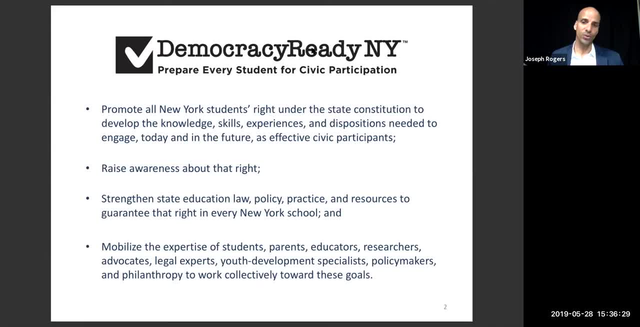 And then, finally, we're mobilizing the expertise of a wide range of stakeholders, And, you see, we list students there. first, because the coalition has made a very strong commitment to ensuring that those New York stakeholders who are most affected are young people and, ultimately, their families, as 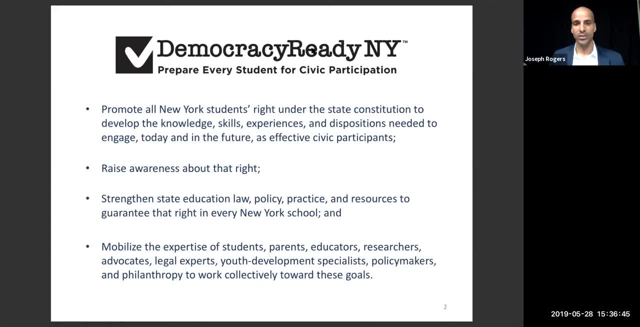 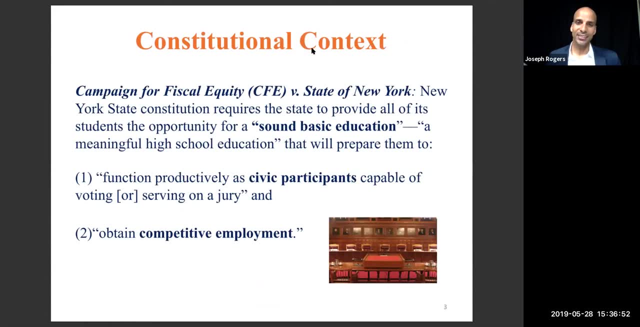 well are at the table, But we also include, as you can see, educators, researchers, advocates, legal experts and other key stakeholders. So back to the constitutional context, Some of you are familiar with CFV, or the Campaign for Fiscal Equity versus the State of New York lawsuit. That was a suit that was waged from 1993 to 2006.. So it 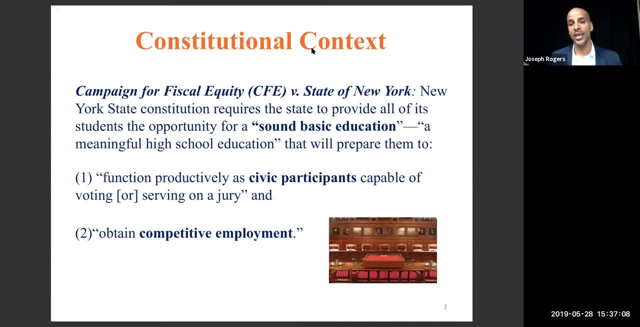 was a 13-year legal battle that was fought with and on behalf of families in New York who realized that their children- and in some cases the children themselves- realized they weren't receiving even the basic opportunities that they needed in order to make a living, And so we're. going to talk a little bit about that in just a moment, But before we do that, I want to thank our panelists. I'm going to turn it over to Michael Rebell from the Center for Educational Equity, the Executive Director of the Center for Educational Equity Centre for the National Center for Educational 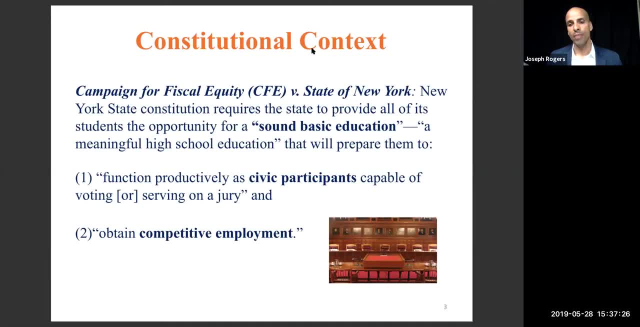 Equity and the Center for Educational Equity and the Center for Educational Equity and Michael Rebell. Michael Rebell, we are so grateful to have you here on this panel, We are so grateful to have you as the Director of the Center for Educational Equity in New York and we are so grateful to be. 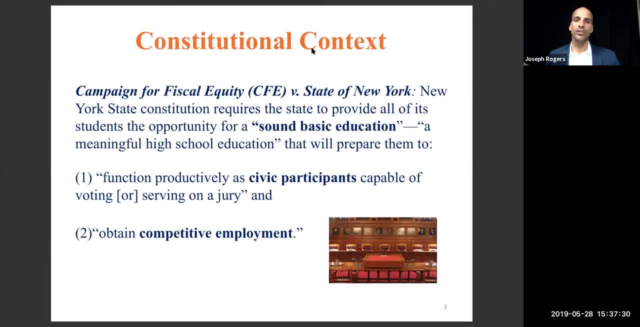 able to meet state standards and, ultimately, to be successful in life As a result of that momentous lawsuit, which was led by the Center for Educational Equity's Executive Director, Michael Rebell. at that point, a couple of really important takeaways or achievements were emerged from that case. So 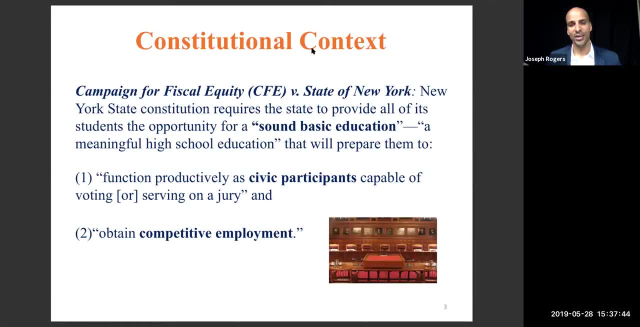 those are the two that are most relevant. certainly, they're both relevant to our conversation, but the the one that's most relevant is: it clarified, it declared that the courts, the highest court, the Court of Appeals, declared that young people in New York State, in every school, every part, 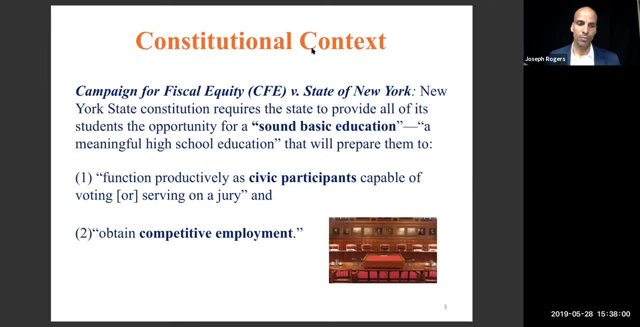 of the state. they have a right to preparation to become productive civic participants. And this certainly isn't an exhaustive list of examples of civic participation, but you can see there that voting and serving in a jury are two of the fundamental roles in our society, and 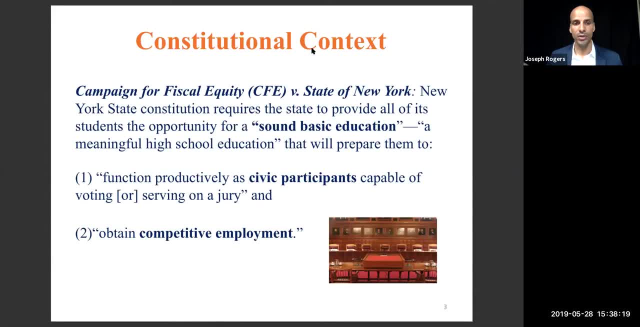 in our state that young people must be prepared to fulfill The other bucket of rights if you will pertain to preparation for competitive employment, which essentially means preparation to get a good job, one that allows you to support your family yourself and to play an active role. 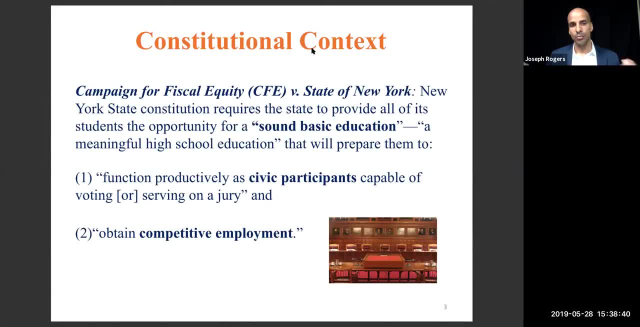 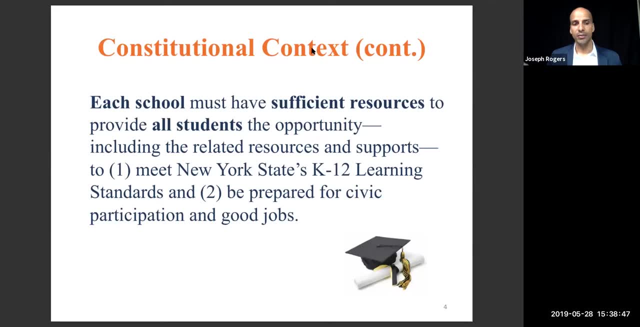 in our society that way. So again, preparation for civic participation was one of the key takeaways from that lawsuit. Just to let's drill down a little bit more, the judges in that case said, and again in the CFE case said, that each school, not just some schools, each school must have the resources that they need in 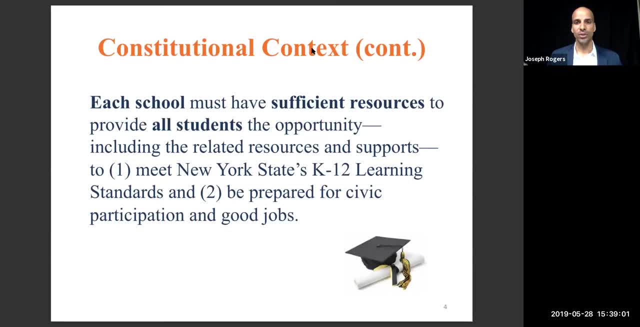 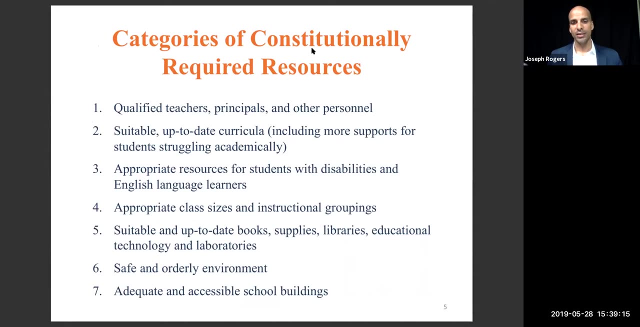 order to ensure all students the opportunity to meet state learning standards, toward being prepared to play their civic roles and to get good jobs. More specifically again, I know I'm throwing a lot of information at you, but you will receive some of the information that you need to be able to. 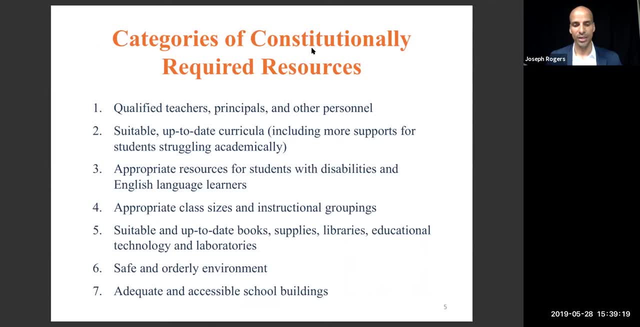 participate in the process. So I'll let you go ahead and read through these details and follow-up emails over the next week or so, But I just wanted to give you a little more background, a little context for the conversation we're about to engage in together. 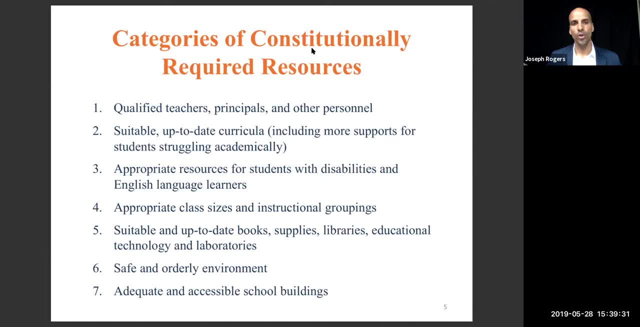 In the CFE case, the courts also enumerated seven categories of specific resources that are fundamental, that are foundational in preparing young people to play their civic roles and again to be able to secure a good job, And those includes. you can read them here. the first one is the 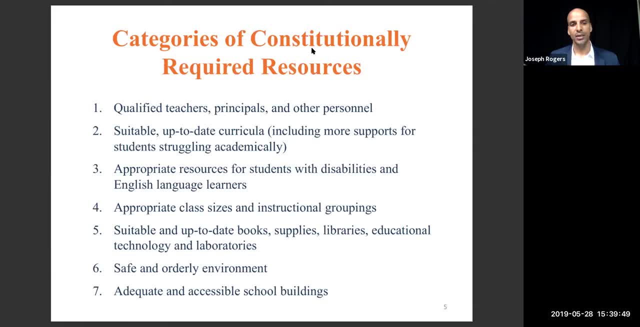 teacher's principles and other personnel. a curriculum that's tailored to the needs of students, particularly students who are struggling academically to make sure they're able to meet state standards and become effective civic participants. resources for our young people who have disabilities and who 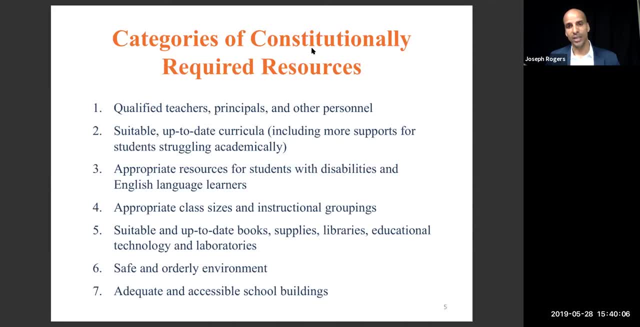 are learning English as a new language. appropriate class sizes. suitable and up-to-date. the judge called them instrumentalities of learning, which is a dense legal phrase, but you can see here that that category includes books, supplies, libraries and other essentials that schools need to be able to. 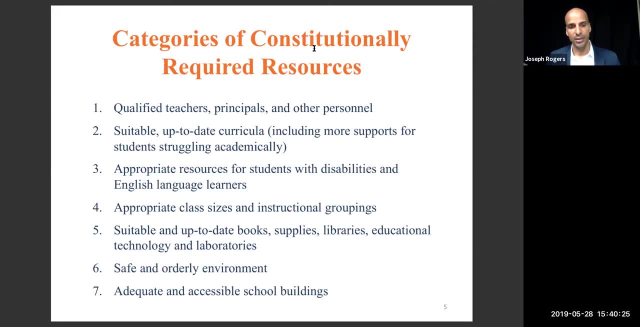 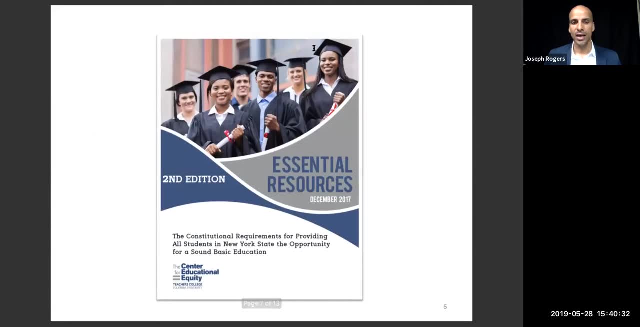 provide to young people a safe and orderly environment and, ultimately, adequate and accessible school buildings. These rights, in great detail in a lot of legalese and policy language, are documented quite well in the Center for Educational Equity's most recent edition of essential resources, which has 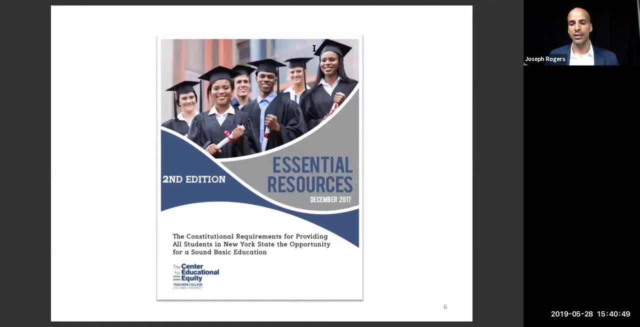 which you can find at centerforeducationalequityorg. It's a, we call it, it's a compilation or compendium of educational rights, every subject area, every social support area, And again, I can't stress this enough. 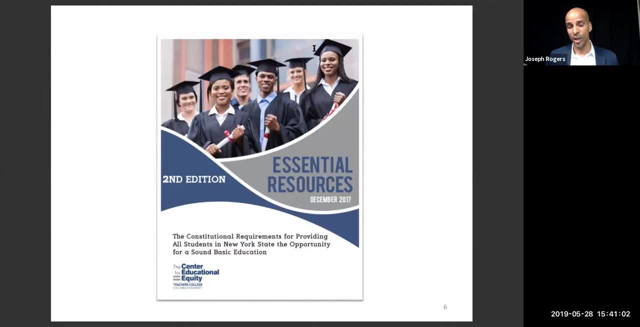 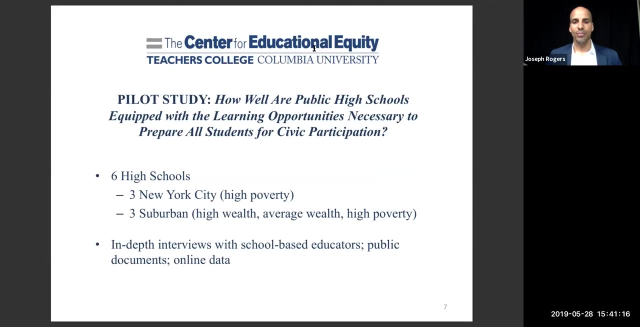 It's not just about right. we need resources, We need funding in order to purchase these opportunities, to afford these specific resources to all young people so that they ultimately are able to participate in and shape our democracy. So the primary text besides the constitution: 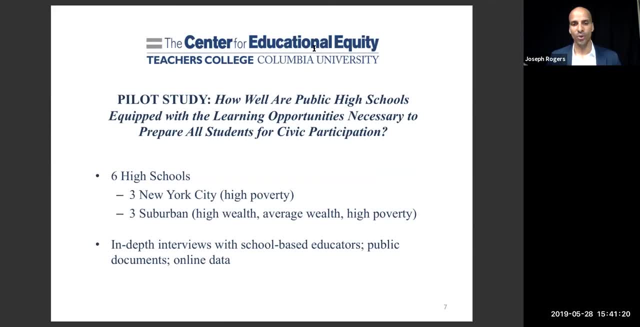 that we want to outline here for you today, again toward supporting your participation. a little later in the conversation is a recent pilot study that my colleagues and I at the Center for Educational Equity, namely Jessica Wolf, who's our Director of Policy and Research- 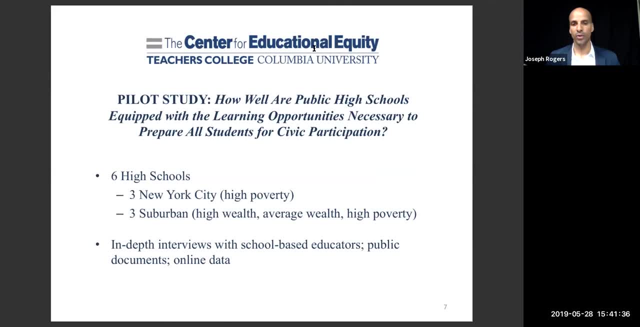 and I, and in collaboration, of course, with our Executive Director, Michael Rebell, conducted in six high schools a small study. That's why, for those of you who aren't as familiar with research research lingo, pilot means sort of an initial effort. 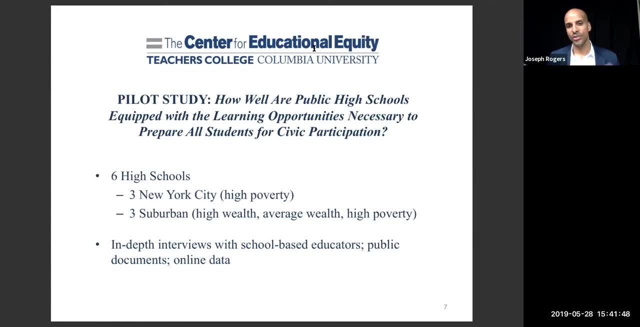 to test your hypothesis, to see whether the questions you're asking are going to elicit the types of information you're looking for toward, later on, maybe conducting expanding the study to include additional subjects or participants, to gain additional information on a larger scale. So, again, this is a pilot study in which my colleagues 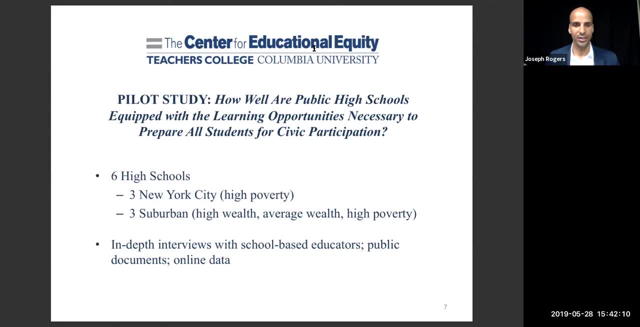 and I went into six high schools, three in New York City, as you can see there, all serving students- One of those students living with poverty, and then three suburban schools: one very well-resourced high-wealth school, a school with more or less average wealth, and then one 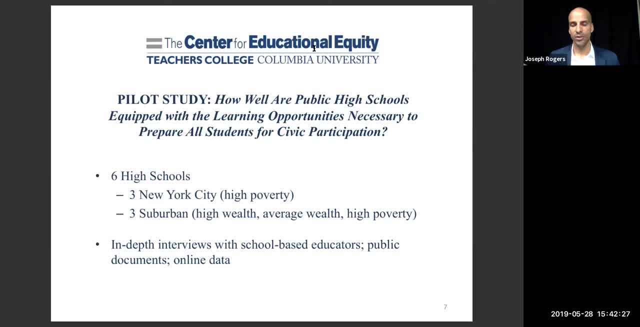 of those suburban schools, also like the New York City schools, was serving a high concentration of students living in poverty. In order to gather the data, in order to better understand to what extent young people in these schools, in a small sample of schools, 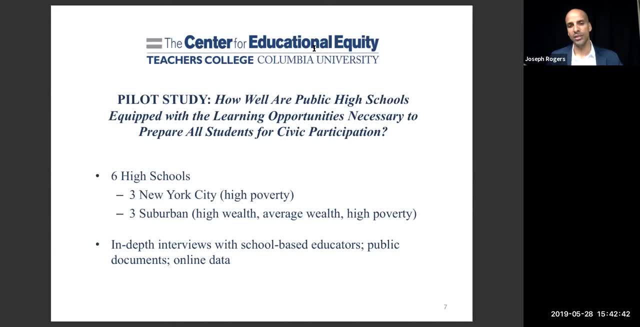 were receiving the specific learning opportunities that you just saw in those seven categories. we spoke with dozens and dozens of educators. We interviewed them, We visited the schools at least a few times and spoke with principals, teachers, especially social studies teachers- and other personnel. 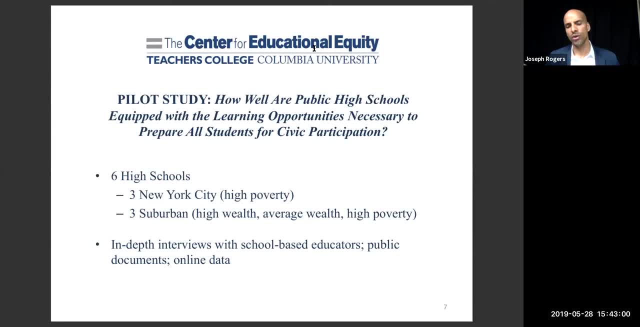 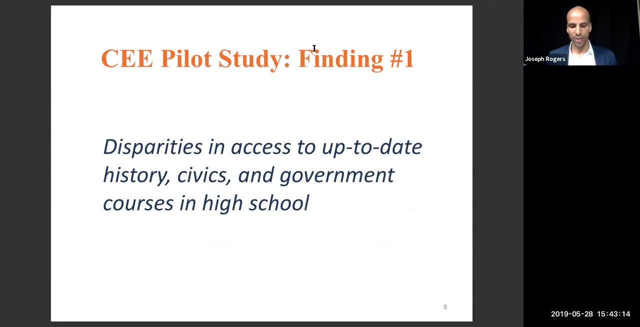 to understand to what extent their schools were equipped and supported in order to fulfill this constitutional obligation that all New York students have. So we conducted those interviews. We also looked at public documents and some online data. So I want to highlight very briefly a couple of findings. 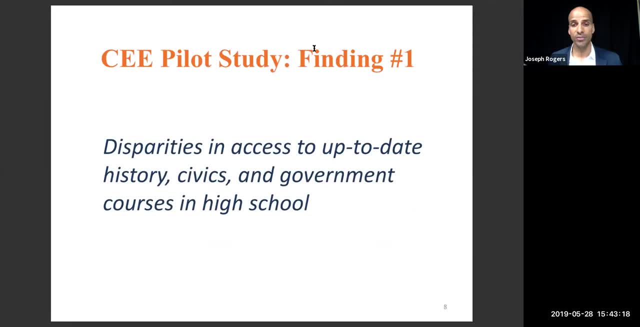 Again, you're going to receive both an executive summary, sort of a quick snapshot of these findings- not just the ones I'm sharing here today, but other findings as well- And you'll receive the full report, which is 50 pages. I think we're up to right now. 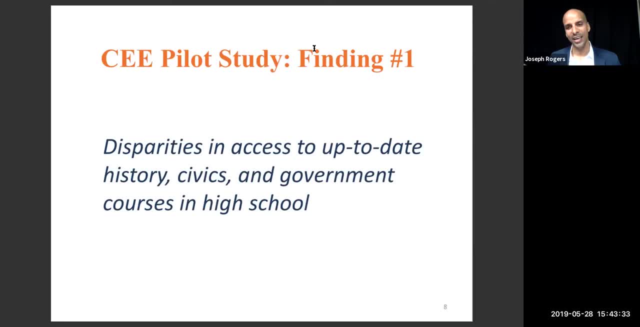 We're excited to release that, to share that with you, And if you haven't already selected some summer reading materials, I can tell you you're going to want to replace whatever you put on your reading list with this report. It's a blockbuster. 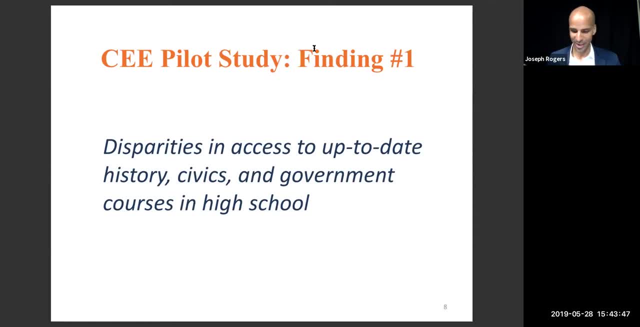 Great beach reading, pool reading or what have you So get ready for that Coming soon to an inbox near you. So let me highlight for you just a couple of these important as I turn to my slides here, these important findings. 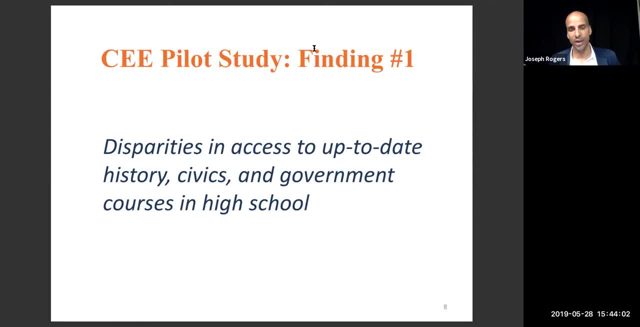 So one finding is we found enormous disparities in access to the basic coursework as well as electives that young people need in many cases in order to become truly civic ready, And I'll pause for a moment there. Just one other contextual piece here that's very important. 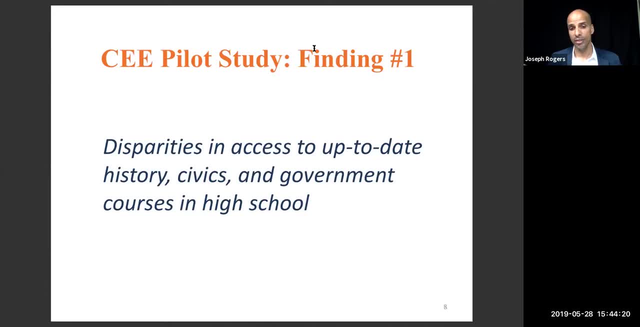 Many of you may know that a few years ago the New York state board of Regents and the New York state education department submitted to the federal government- and every student succeeds- act plan, basically a plan for how the state is going to comply with federal regulations toward meeting the needs of students throughout our state. 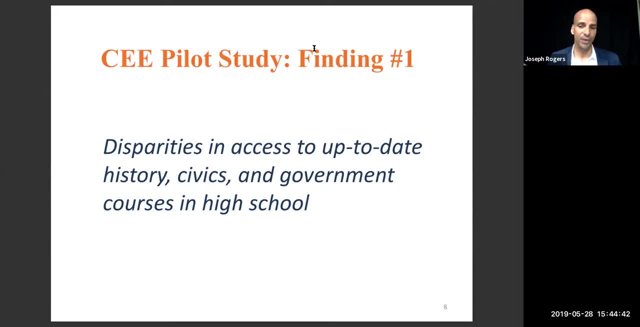 And in fact in that plan for the first time, they identified civic readiness as one of the key goals for our state's educational system. So before we talked a lot about college and career readiness- obviously important, but they added this third C and that was instrumental. 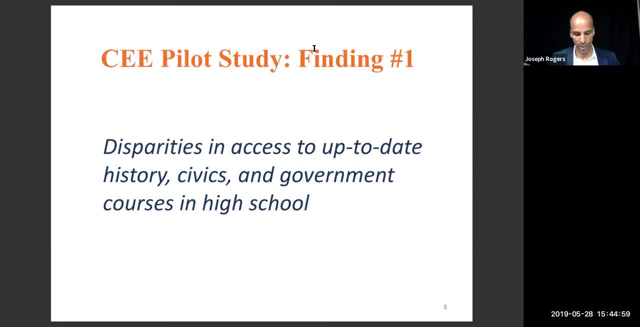 And it is really one to also one of the organizing principles for our work here. The state continues in its official capacity to advance that work And we're finding opportunities to gain synergy, really to coordinate and collaborate Among the various groups, including democracy ready. 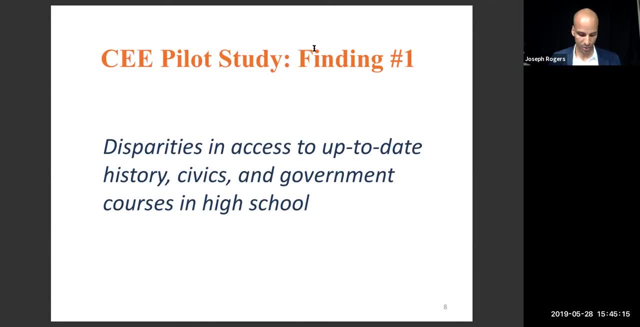 New York coalition and the state's current civic readiness task force. So I will tell you that those disparities and access to some of the fundamental course in high school not only concerned the level of detail that schools were able to cover toward meeting the needs of their students in the core classes. 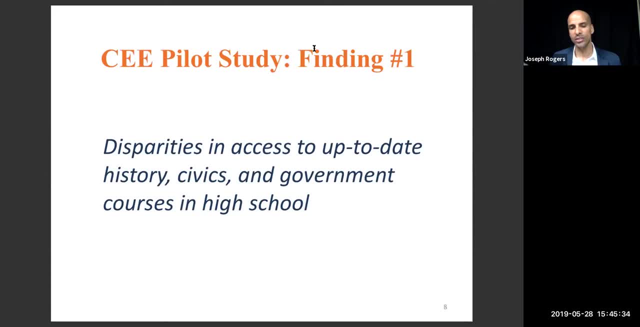 but it include a wide range of major disparities, major gaps in access to civic learning, learning related elective courses and really, just to really drive home the point, we found in our best resource school, in that high wealth district school that had 20 electives. 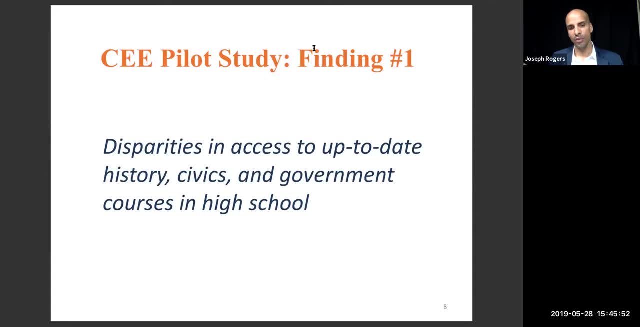 related to civic education, And in some of our the schools that we visited, including most of those in New York city, some of them weren't providing any elective courses not related to civic, civic learning and civic preparation, not because they didn't care about their students. 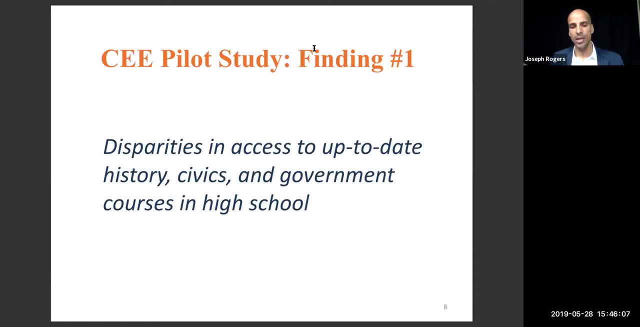 not because they weren't committed to preparing their young people, but due to due to resource issues, they did not have the staffing they needed in order to provide a wide range of opportunities to our young people. I also note here that just back, 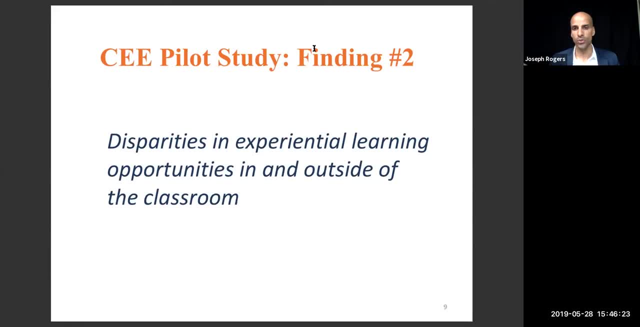 back on that last finding of the better resource. schools were able to provide redundant opportunities, meaning they didn't just have one section of a course, They didn't just have one class, They had multiple courses to make sure that all students were able to access them. 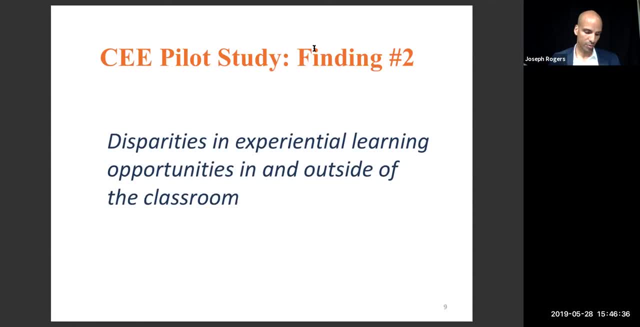 Another major finding that you read more about in the forthcoming report is disparities in access to experiential learning opportunities. That includes both democratic conversation and debate within the classroom, as well as what some would consider either extracurriculars or and. 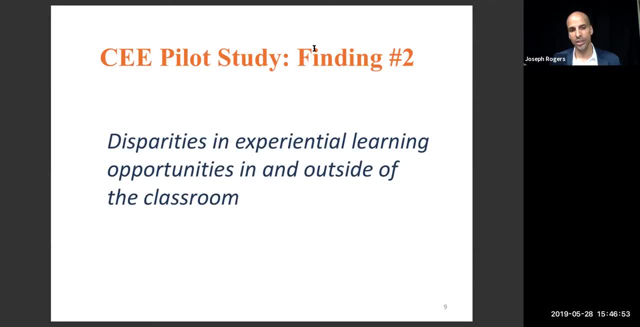 or field trips. So one of the key. you know the literature, the existing literature on civic preparation and civic education says it is very clear in the point that young people need extracurriculars and what some people would see as extra. 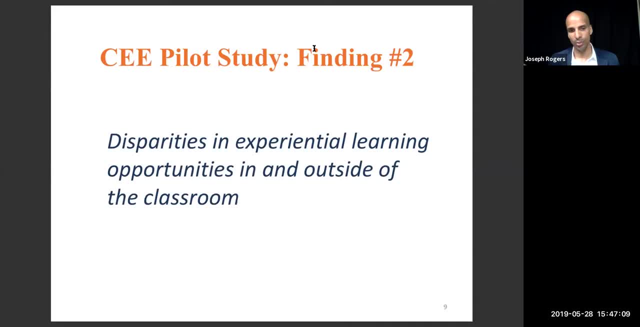 extra resources In some cases. for example, a school newspaper, student government could be a work in the arts, But the theater, for example, which allows them to examine issues from multiple perspectives toward becoming civic ready. We found that particularly the school, serving mostly students and living. 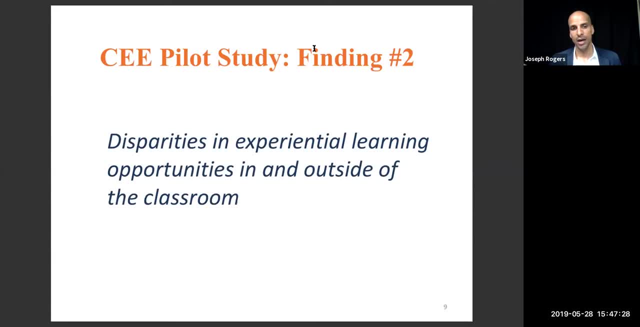 in poverty, they were unable to provide the wide range of experiential, hands-on learning opportunities to young people need in order to practice the skills. It's one thing to learn about, it's one thing to study the text. it's another thing to actually to exercise and to practice. 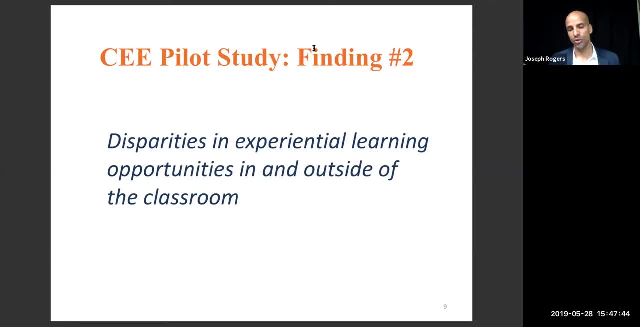 and develop one's skills, And that can only come- which is true for both children and adults- through, actually, you know, grappling with things yourself, real world problems, being hands-on. Another, let's see another important finding here. Jumping along here, None of the students, and so you may find this, either, really surprising. 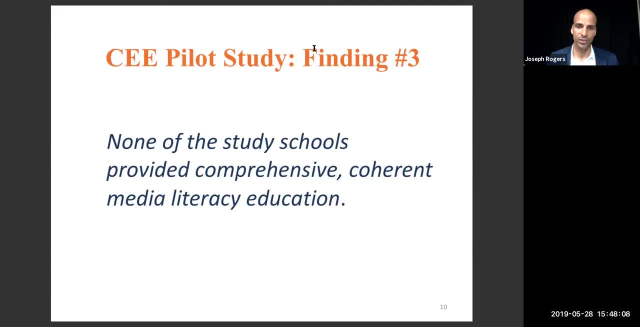 or particularly if you work in schools and perhaps you're a student yourself, may not be surprising, but particularly given the how the internet is so pervasive, how it in many ways drives- whether it's through news or through our browsing- what we learn and what we 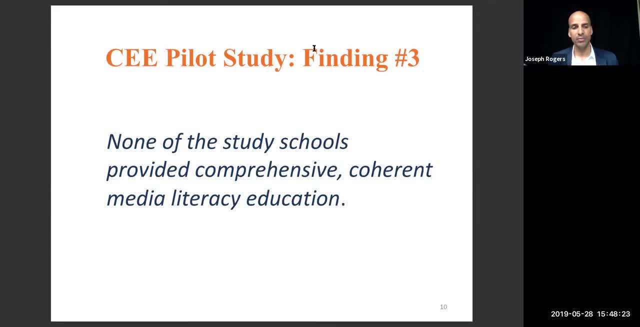 know what we believe we know and what sources we consult. None of the study schools, none of these six schools in our sample, were providing a really comprehensive and coherent media literacy education. So in fact, some of the schools were not providing. 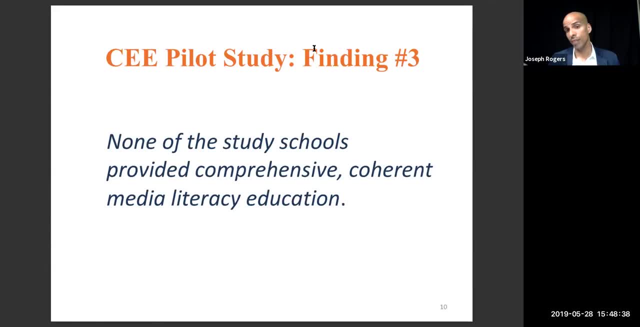 providing access to library media specialists or school librarians. Those are required under state law And yet some students didn't have access to the additional research support, the additional support our young people need to be able to distinguish: good, solid, reliable. 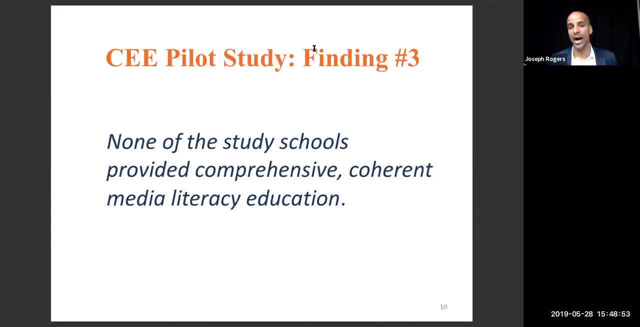 information from unreliable and heavily biased information to be able to develop the judgment, the discernment, to know how to answer questions with good information. So with that I'd like to go ahead and end the session. Thank you, And I think that's probably. it probably sets us up for the introduction to our amazing panelists. 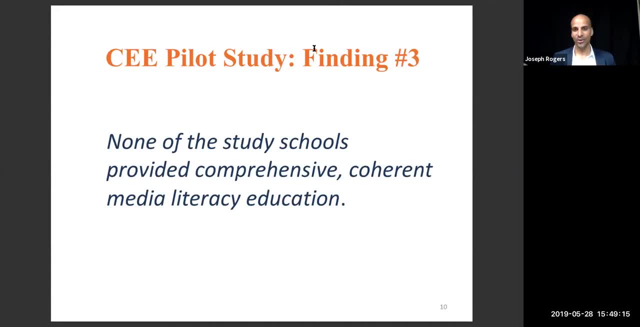 for today and I'm excited here to good. And you see, the panelists are going to start popping in here. their videos will show up and this is this is the queue to appear. Look at that like magic, Wonderful, All right. so I want to recognize that we have a wide range of key stakeholders here. 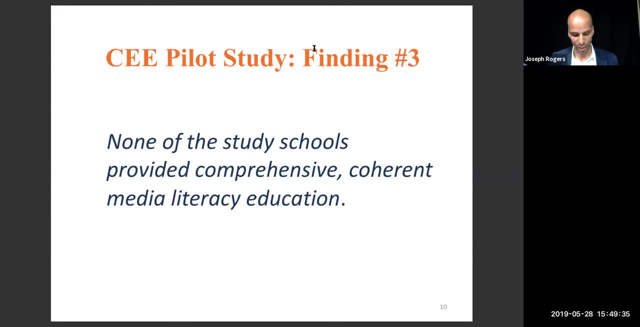 There are more, but often, when people think about education, they sometimes think about education. they think about students, parents, educators, the youth development and nonprofit spaces and school boards. Next time we have a webinar, we'll include additional voices, But right now I'm excited and pleased and honored to introduce Hamza Noor. 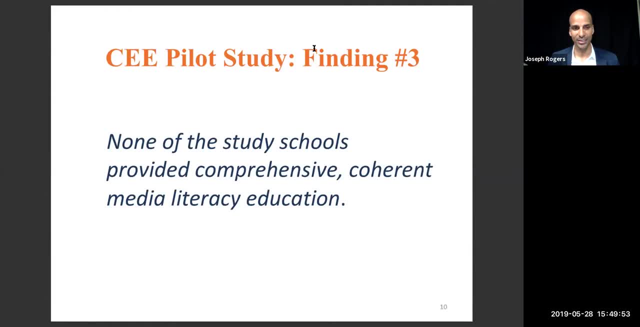 Hamza is an 11th grader at Chalmont High School in the Capital Region. Welcome, Hamza, Hamza, I should also note, is a member of the Democracy Ready New York Coalition and is part of the youth leadership initiative that we launched at the beginning of this. 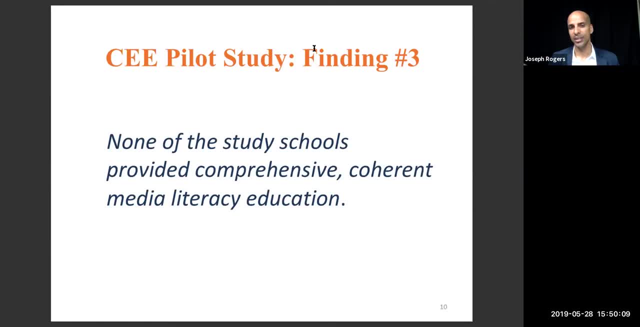 process to enlist young people's leadership and insight and experiences in guiding the coalition toward ultimately guiding the state and recommending to the state some of the changes that may need to be made to fulfill the constitutional obligation. So thank you so much, Hamza, for being with us today. 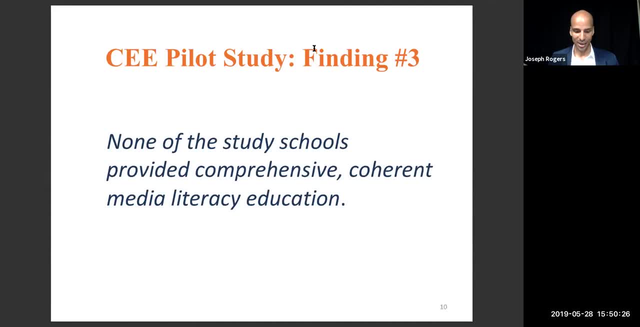 We also have here Leah Entwala. Leah is a parent who comes to us from Seneca Falls School District which is up in the northern North Northwestern part of the state. Leah I'm really pleased to share she's a member of or represents in many ways among. 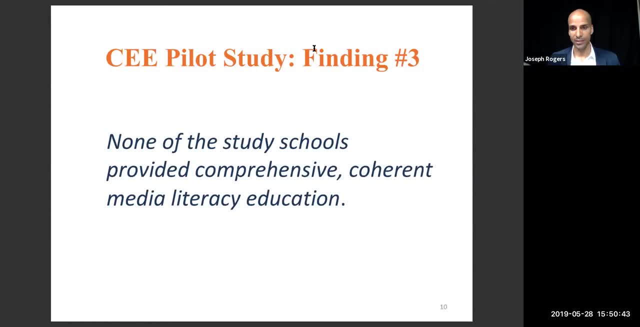 other hats she wears. She's a rural parent And so often we have these siloed discussions about education and educational improvement. Sometimes we have an urban conversation, We have the suburban conversation, We have the rural conversation. Rarely do you bring all these different stakeholders together? 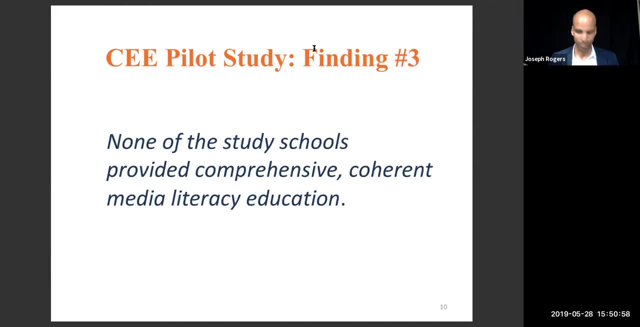 So thank you so much, Leah, for being with us here today and offering a parent's perspective. We have next Tiffany Alan Hubbard. Tiffany is a social studies teacher. It's critically important to have educators at the table. We're talking about improving education, obviously. 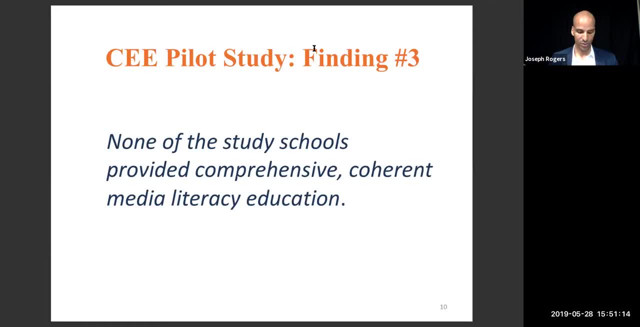 She's a social studies teacher at Hillcrest High School And she is also a site specialist with the United Federation of Teachers or UFT Teacher Center, And they have some exciting civic learning-related work that they're doing with a small network of social studies educators and others. 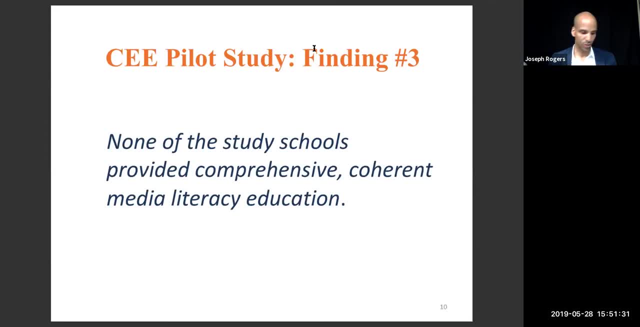 And we look forward to hearing more about that. Stay tuned. Next we have Diana Vasquez, and Diana is the statewide coordinator of the Angelo Del Toro Puerto Rican Hispanic Youth Leadership Institute. amazing statewide organization. partners with schools but largely operates outside of the school context, providing 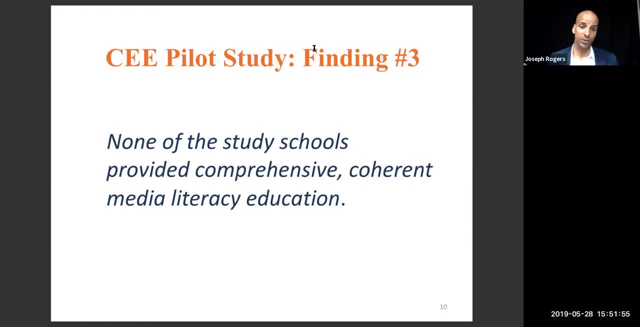 experiential, hands-on learning opportunities that include actual contact and exchange and role modeling with actual legislators And in our state capitol. So you'll hear a little bit more about what they're doing and why that's important. And certainly last but not least, we have Jay Warrona. 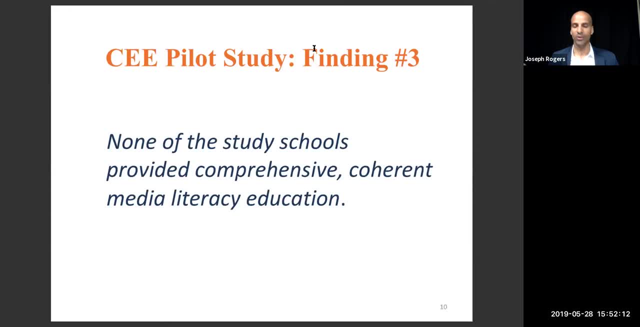 Jay, thanks for being with us. Jay is the deputy executive director and general counsel of the New York State School Boards Association, So it's important we have a management perspective here as well. So thank you so much, Jay. So I'd like to right away switch to and let's go ahead and what I'm going to do here. I'm 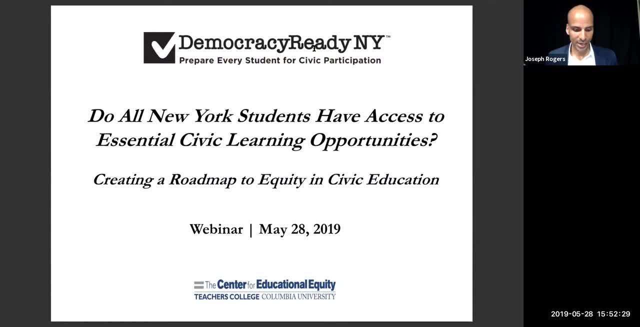 going to bring us back to this slide is. I have a set of questions Based on the findings from this forthcoming Center for Educational Equity report that are targeted at the specific experiences and expertise of our stakeholder representatives. I'd like to start with Hamza Noor. 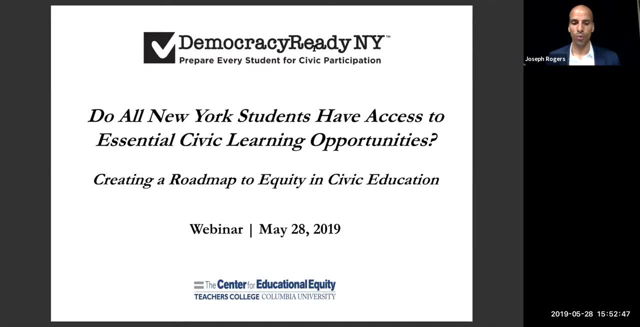 Hamza. extracurricular activities, for example, working on the school newspaper, on the student council or in clubs based on students' identities, are one way that many students access important civic learning opportunities. However, this study suggests that students who work after school in order to help students'. 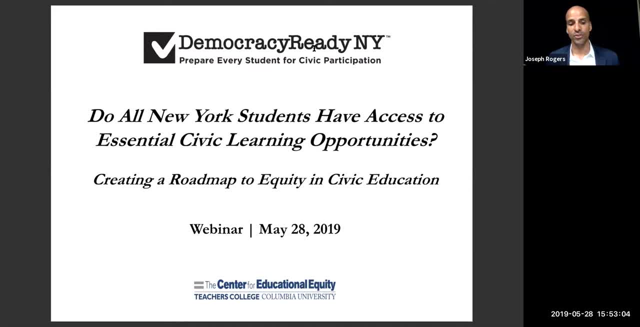 or support themselves and or their families cannot stay after school to participate in any of those clubs or other extracurriculars. What can schools, districts and or the state do, through policy or otherwise, to ensure all students the opportunities to participate in these hands-on, experiential civic learning opportunities? 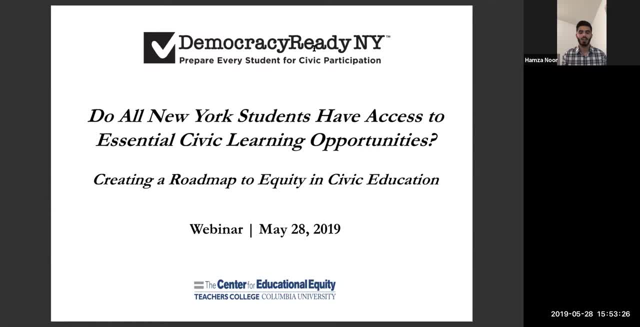 Good evening everyone. First of all, I'd like to say that I'm thankful for the Coalition for giving students this opportunity to represent, Giving me the opportunity to represent students, because you can't solve a problem without talking with the people that it affects. 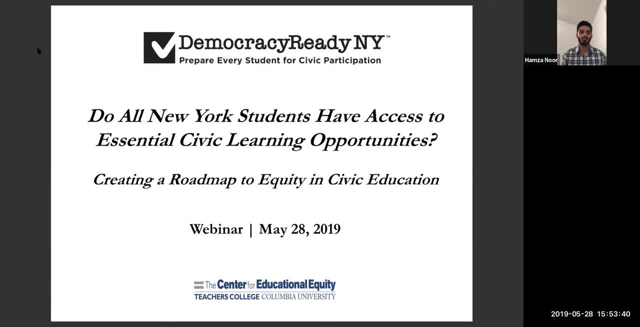 So I'm thankful for that. So this question directly relates to me and a lot of other students, And it's an issue that we've currently been working on in my school district, And so I'm an activist and community organizer And oftentimes I've experienced that the work I do and a lot of other students like me do, 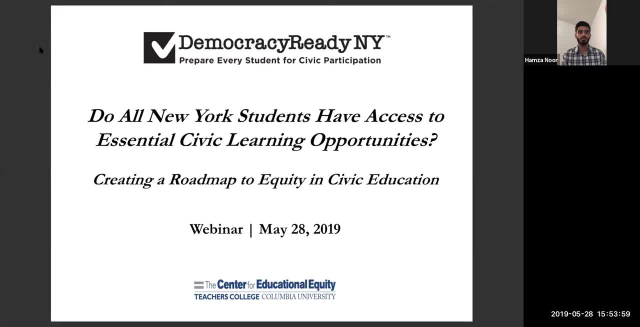 interferes with our schoolwork And, without a doubt, The work that I and many other students do outside of school benefits us just as much as school does, And different kinds of extracurricular activities not only teach us like life skills and they build character. 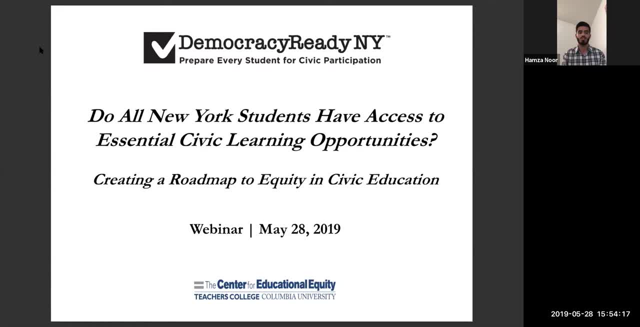 but they also strengthen students, resume and show colleges how a student is well-rounded. Along with that, students get many civic learning opportunities, because they're doing more than just schoolwork and they're doing real life things. Um, The idea that I presented to my school district, and is being discussed by my admission right now as well, is that it's providing students with the freedom, time, space. 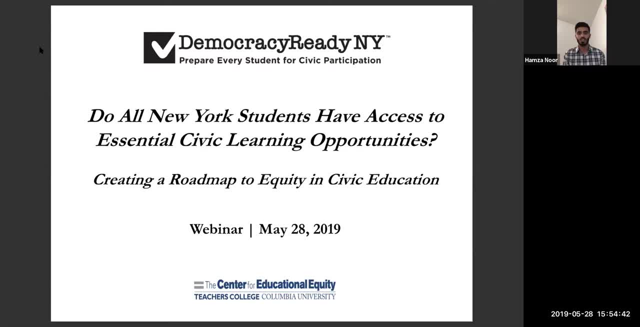 Availability to do extracurricular activities in their school schedules during school days, and a period or small amount of time is designated for students To work on their own project, research on organizing or whatever they they're pursuing at that time, and they can. that can be activism or leadership, like me, or a student working on their own. 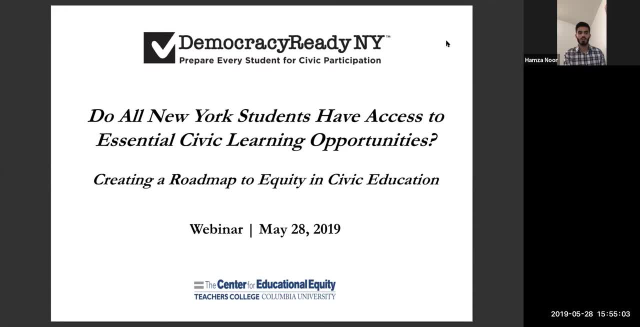 You know business, Or working on their own project to research project, or you know building a robot for engineering class- and The possibilities are endless with with today and students are- can be given Credit and recognition by the school for the extracurricular activities that they. that they do and different forms of projects and organizing different events are great civic learning experiences that should be given credit for. 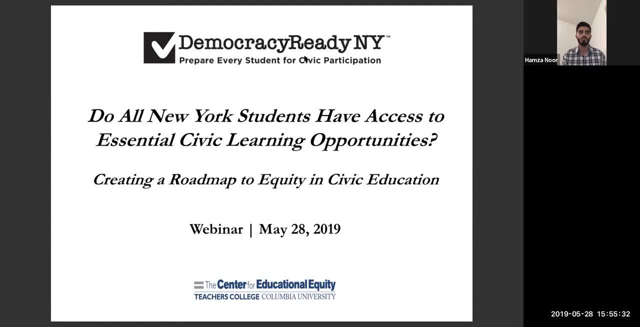 On, after a quarter or Set amount of time, on The students. the students have an adult supervisor that I'm not only like supervisors but provides guidance and helps help soon whatever way they need. And after a quarter set amount of time The adult meets with the students to see the progress that they have made in those in their specific projects and and assesses it and this. 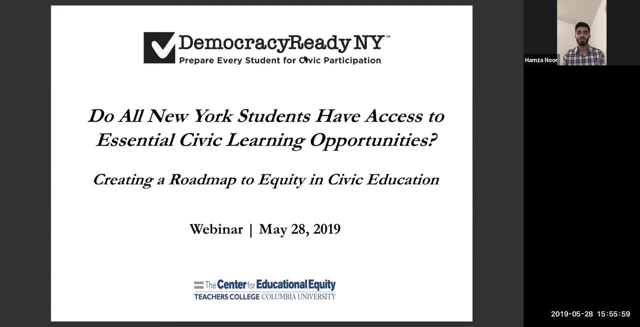 Advisors able to Provide the right resources and The right Information or the right guidance, and just notice them in the right direction to achieve whatever they want to achieve. that includes, like availability of resources in schools or providing new leads to internships or different ways to Get to where their students is trying to get with their project, and this allows- this also allows the adults to assess how the student is learning 21st century skills necessary to be successful in today's world, and students 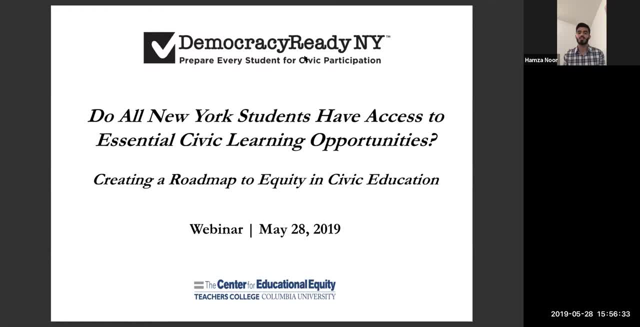 Will be Students being able to work on their own project with that they're passionate about allows them to have real life experiences in high school while also doing schoolwork, which is really important, And that also teaches. from my experience and many other students like me that I've talked to And I see that that teaches a lot more: a lot of civic learning opportunities, experiences and 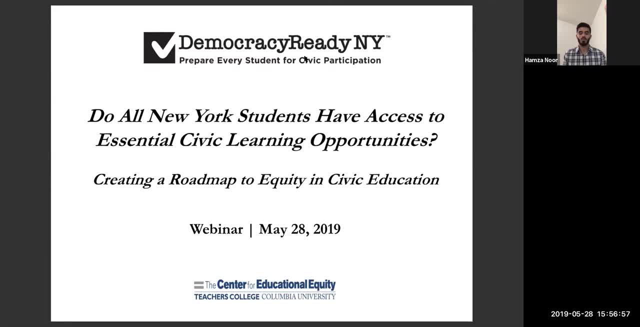 Um, that that that definitely is a really important part of you know learning, learning these experiences, And I think that's a really important part of what's going on in our community is actually doing these things, And if the student at school is able to provide that for you in there in the school schools schedule, that that 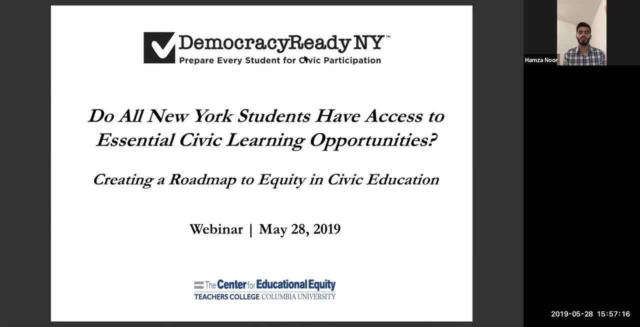 Makes it a lot easier for a lot of students to that aren't able to do these things outside of school to be able to participate in them. and This is the idea that I've presented with my school and they're working on it And I believe that it will increase the civic learning and preparation of New York State students. 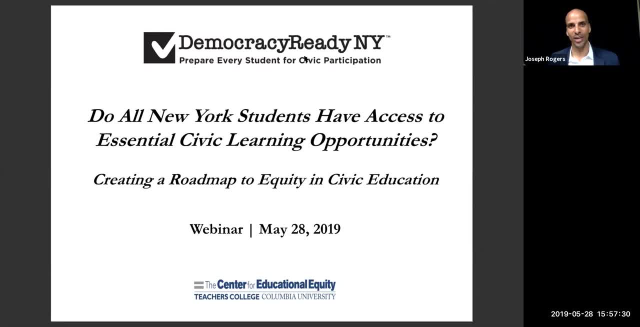 Great, Perfect. Thank you so much, Hamza. Well, how do we achieve equity? by, as you said, embedding these hands on opportunities, clubs and what have you during the school day? You're actually exemplifying civic participation by taking this idea of bringing it to your administrators, and we look forward to seeing how that works out, perhaps a model for other schools. 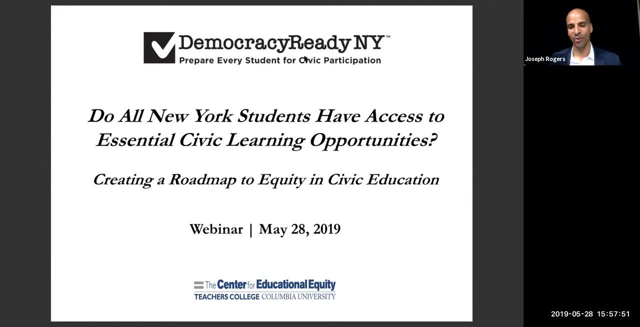 Around the state And we look forward to sharing that and following your work in general. So thank you for for taking that leading us off your arms. I appreciate it. So we have next. again we have Leah and to Allah, Lee is providing a parent perspective today And a question for you, Lee, is when many people think of parents roles in education. 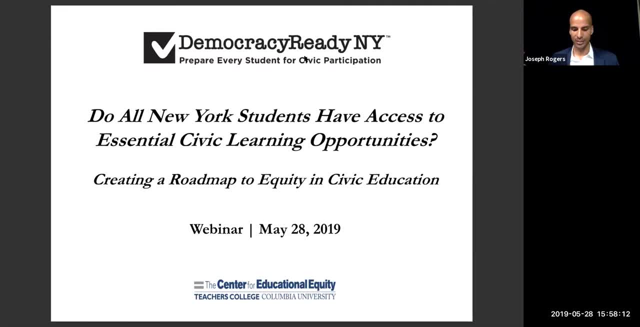 They focus only on school level activities. Some people think about the PTA etc. And those are really important. right, we're not. we're not. we can't understate the value of PTAs And I know some PTAs are involved more broadly at the policy level. So, with an eye toward that, how can we ensure, how can we ensure that parents at the table, How can they help? 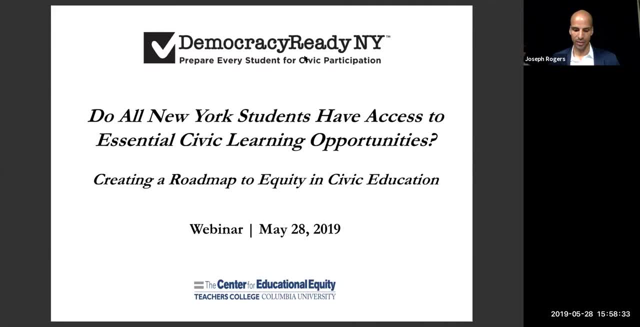 Eliminate disparities and access to some of the civic learning opportunities that we found in our study and that you know are not available at the school district and state levels. What, what can parents do to help move the conversation, ultimately move us all, toward Providing access to all young people to the full range of learning opportunities? 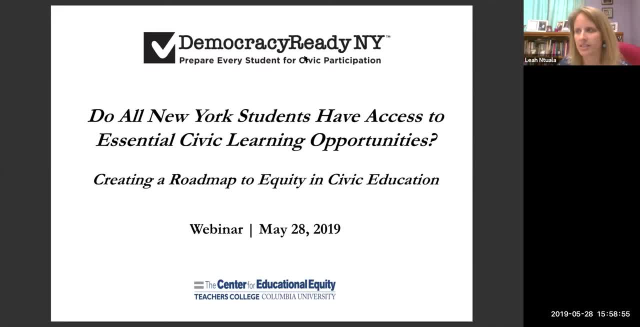 Well, as a parent, I strongly feel that a an essential part of my role in my child's education is Supplementing Whatever it is that they are already learning in school, So using the library to access more information on a topic that my kids are learning already. 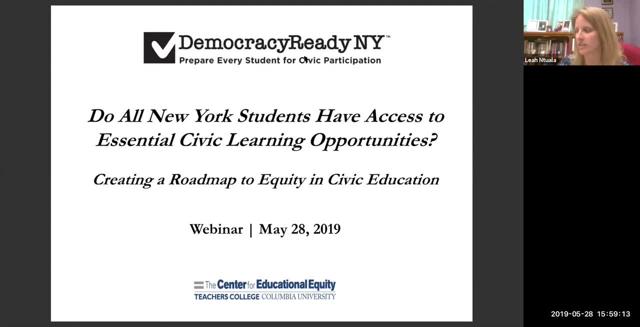 However, you have to sometimes have the resources to do this, which include money, time and transportation, And several communities and students and parents do not have this at their fingertips, particularly in rural areas, I think. But I think the best asset that a 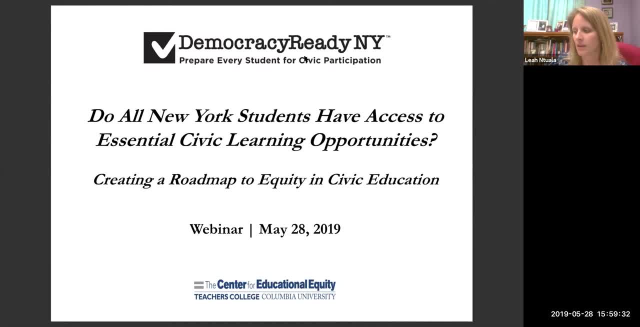 Community always has are are the people, And that includes your parents and everything. but at every level in in any city or town across the United States, You have local leaders. It doesn't have to be civic focus, doesn't always have to be at a federal level. So how do you access the people who are in your community, who are holding local offices? How do you, how do you engage them in the school? 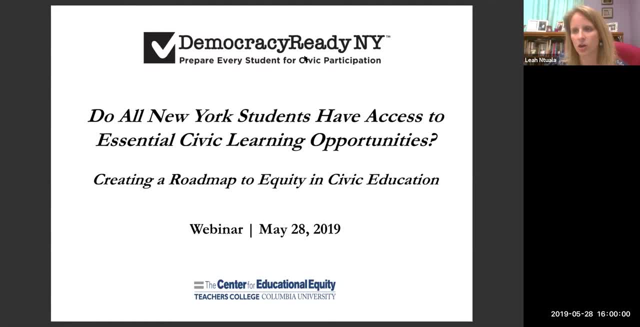 The other thing is a parent is. I feel like some of these conversations, Conversations, start too late in our child's education. If we want our children to be civically engaged, I think it needs to be a K through 12 efforts. It's not just a civic course you take as a 10th grader or 11th grader, or when you register to vote and having had no preparation, 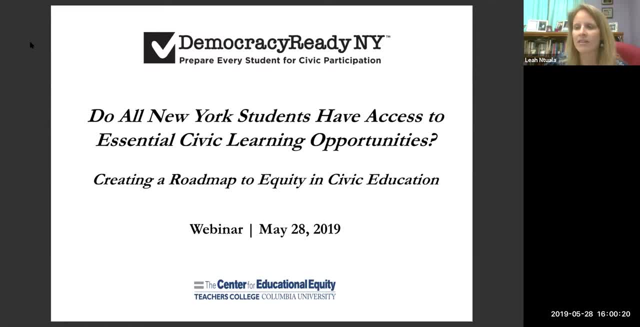 So I think the earlier we can make kids aware of even the calendar of voting is something that you can do that doesn't cost any money. So I think it's thinking creatively. So I think the earlier we can make kids aware of even the calendar of voting is something that you can do that doesn't cost any money. So I think it's thinking creatively. 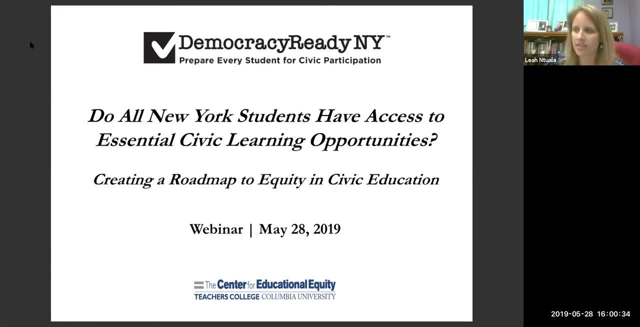 About the resources you have And most of the time we can. I think as a parent we can engage our communities and our students and our children In something that costs nothing but time. so it doesn't cost any time to let kids know and how maybe they would vote on a school levy. 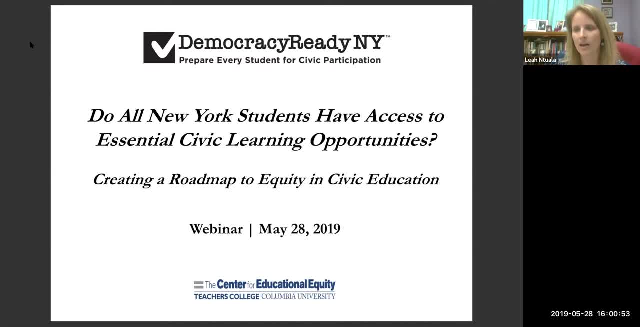 And presenting that information and letting them, K through 12, have mock trials and ballot boxes in their school so they get used to the idea Of what it means to vote and how the voting process can change that, of what it means to vote and how the voting process can change that. 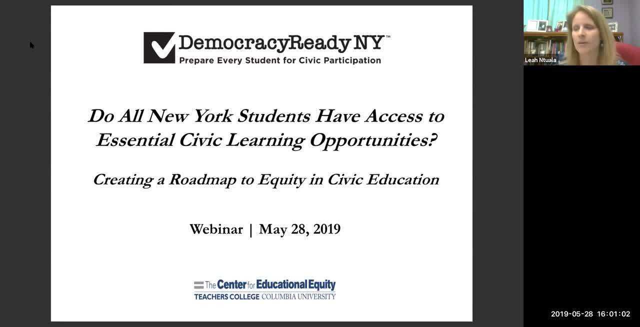 And so I think that's a really important part of being able to get the voting cycles done. when there is a local election that's happening or primary that's happening, It doesn't have to be federal- you can ask those people to come in and present their ideas to the kids and let the kids voting ask questions. 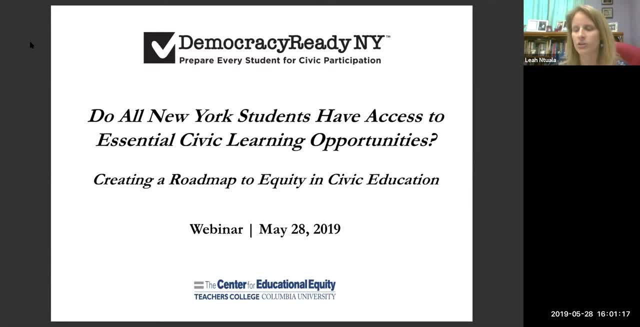 I think registering to vote is a big thing And I think students should be leading those at all School events. there should be a table led by students K through 12 at these events. That says register to vote because if your kid is asking you how you participate, 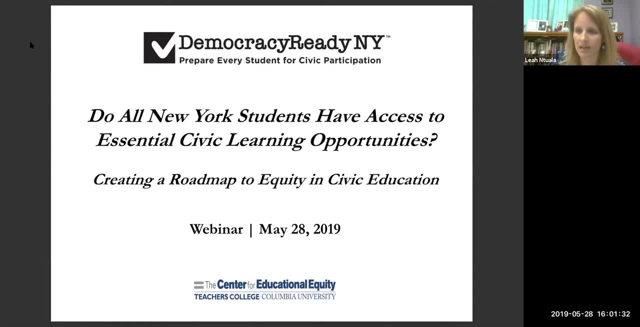 If there's seeing that, then not only does it empower you as a child to know what that means. I think the children then can empower their parents in these activities. I think it's also looking at neighboring schools on various levels to say, if we can't go to DC, how do we access our? 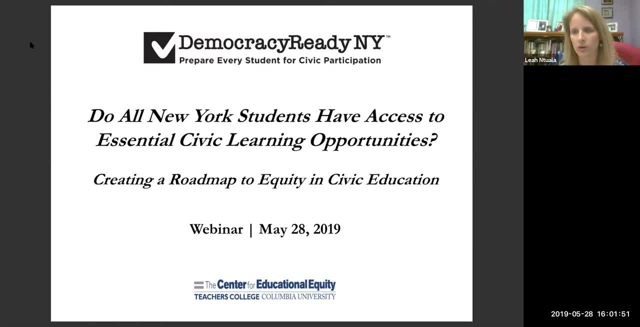 neighboring communities or partnering schools, where there is disparity financially, to say, how can we supplement these kids so that they can go maybe not to DC or something, but to a local historic civic engagement site or having conversations like with this activity, to be able? 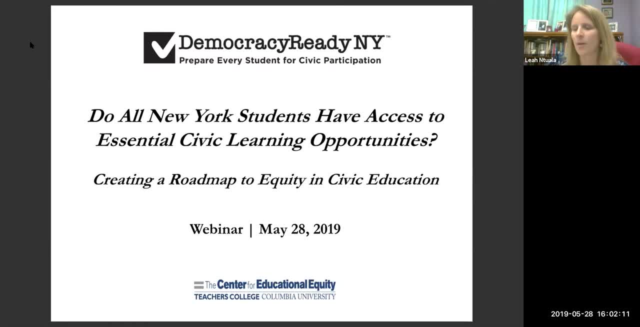 to engage our students more in these panels and topics. So I think some of it is with parents and I know as a parent you're exhausted by your kids' school activities and their homework and all our kids do those things differently, but it's recognizing that your biggest 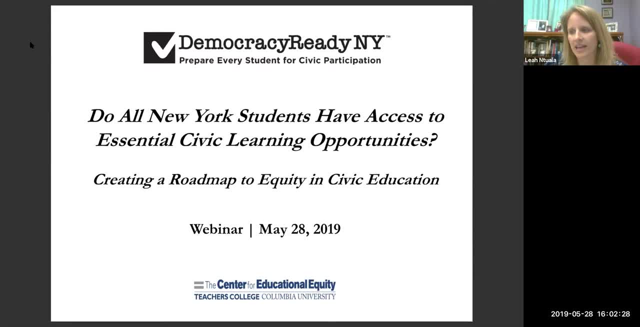 assets are your kids' activities and your kids' activities are your kids' activities. and your assets are always your people. and how do we engage the people in our community to want to partner and participate with our students, knowing that the more knowledgeable we make them, the 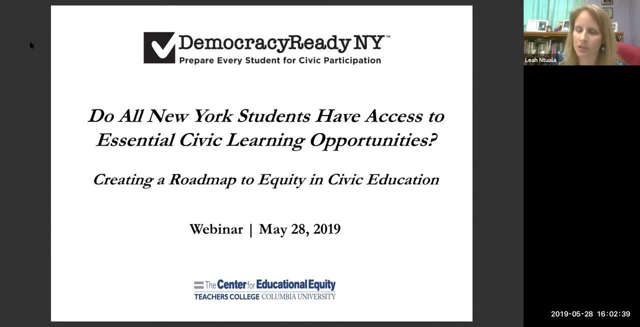 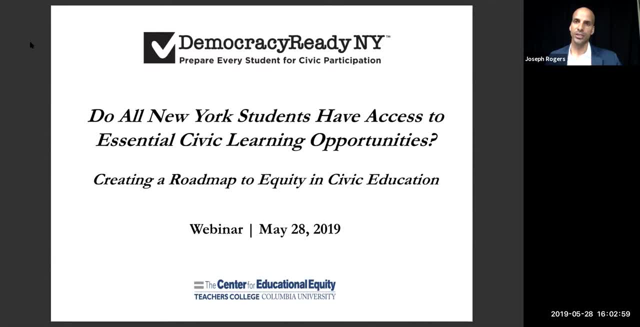 I think that's a great point. I think that's a great point. Particularly in rural communities, it may be difficult to transport young people to and from extracurricular, whether it's learning opportunities, whether it's through clubs or what have you. 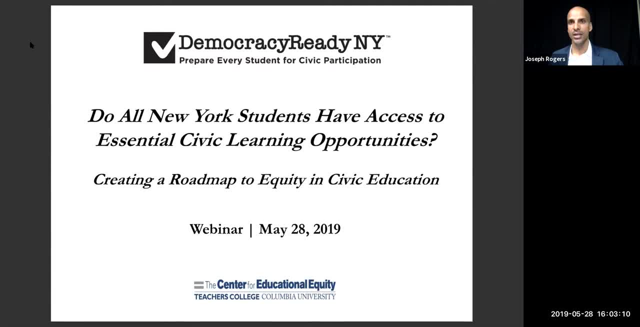 And I remember that from a study we conducted a number of years ago that that was something that rural principals and teachers told us about- is that that can be a major barrier. There are costs associated with that. You have to be able to provide adequate transportation beyond. 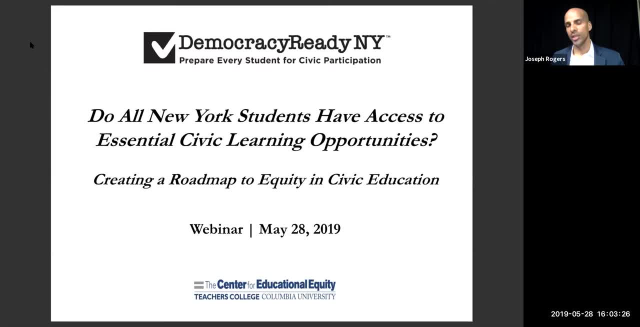 that required for participation in the regular society of kids. I think that's a great point. I think that's a great point. I think that's a great point: school day. But he also says something I think is really important. I just want to underscore. 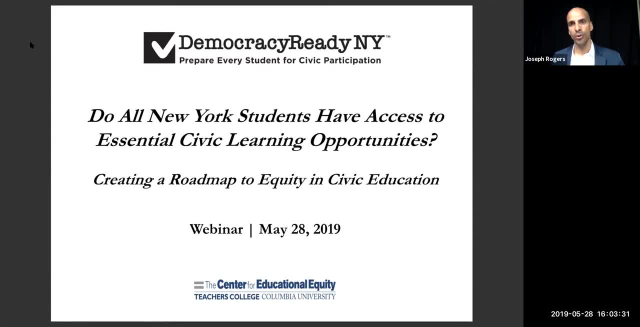 which is about using existing resources, including your people being your most important resources. So, while there may be things such as transportation in a rural community or staffing, or you know other resources in those seven categories that we discussed earlier that you may need more of, 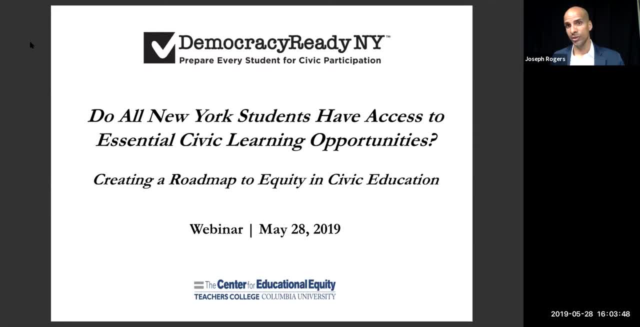 or may need different kinds of in order to prepare young people. look at what you do have already and see how you can make the best use of that And that included, as you said, making sure young people, our students, are involved meaningfully in hosting forums. 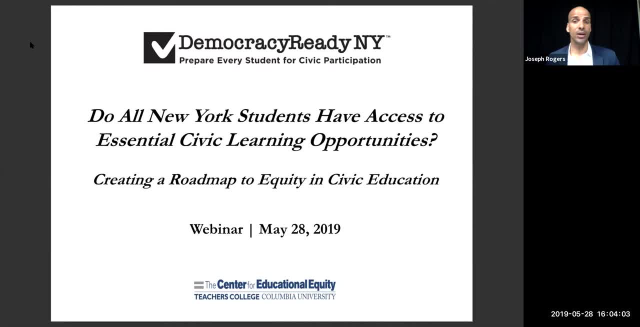 participating in these kinds of conversations about how do we better strengthen our schools toward ensuring all young people these kinds of opportunities. So thank you again, Leah, for sharing your perspective as a parent. I'd like to turn now to Tiffany Allen Hubbard Again. 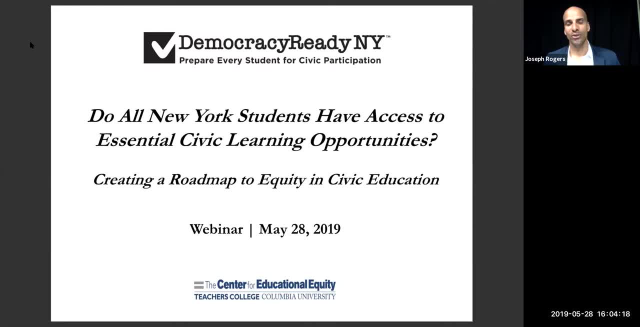 Tiffany is a social studies teacher at Hillcrest High School in New York City and she's also a site representative or a site support Site coordinator with the UFT, with the United Federation of Teachers Teacher Center. So she actually teaches and she supports other educators in her school and beyond in. 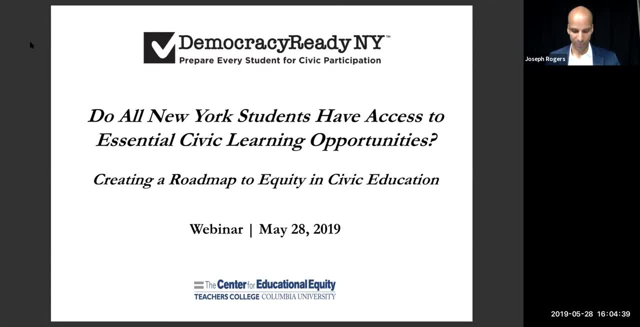 serving their students well. So, Tiffany, if I may ask you, the study findings suggest that some high schools have the resources to hire a sufficient number of teachers to provide a wide range of course offerings across the curriculum that contribute to civic readiness, Including, for example, as I mentioned earlier, social studies electives. 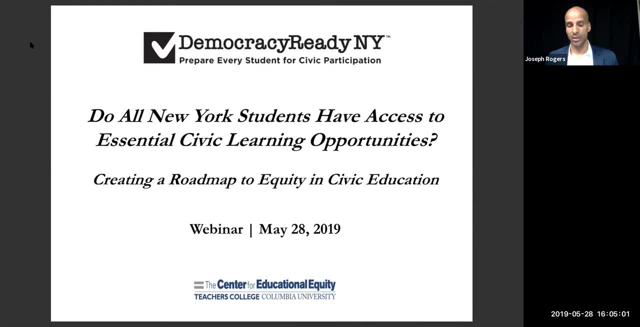 and current issues and advanced coursework related to civic issues, while others offer no or very little more than the core classes, the core courses required to graduate. Does this matter, And if so, how? And then what can we do from a policy perspective, from your perspective? 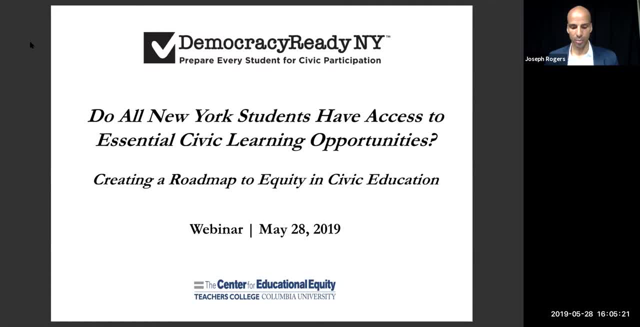 as an educator, to correct some of those disparities, to make sure all students have access to a rich and wide range of coursework, if it's important. Good afternoon everyone. This has really been an interesting meeting of the minds So far. I'm really 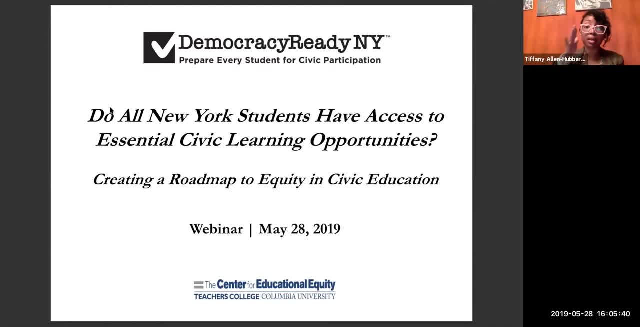 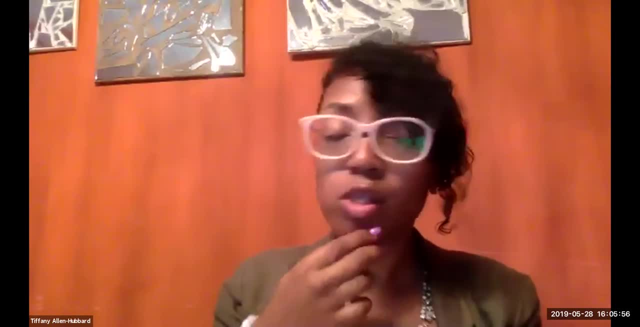 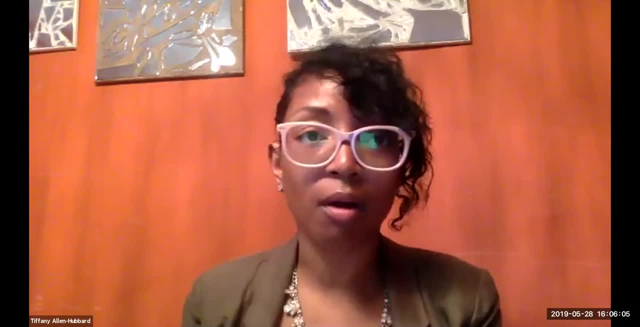 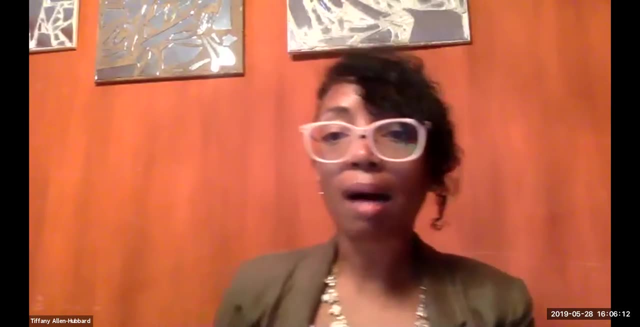 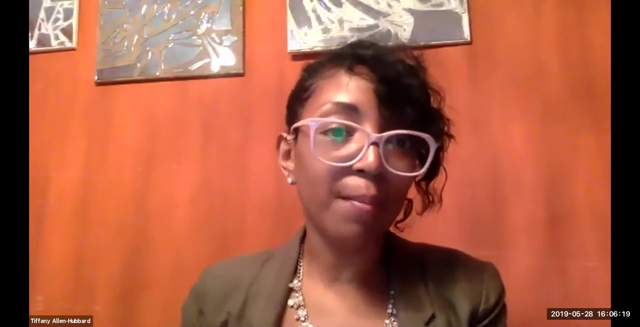 Right now I'm at Hillcrest High School in Queens, which is a large and pretty diverse school And we have so many opportunities for students to engage civically through things like our theater program and our public service program, connection to NYPD and FDNY Explorer programs. 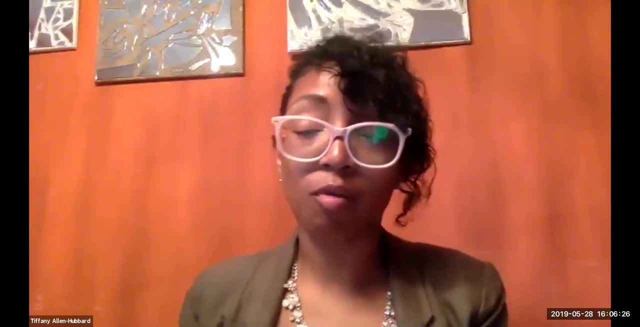 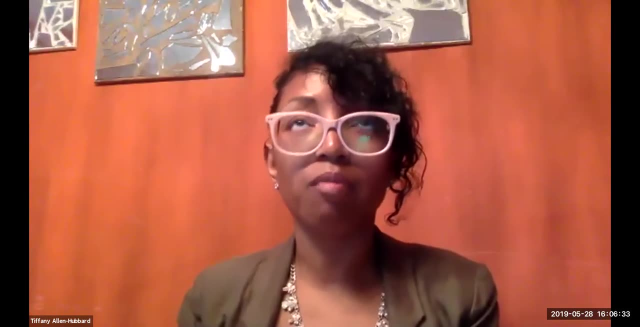 mob trial Model, UN, so on and so forth. I really wanna speak today from the perspective or from the understanding of those schools that don't have that, which are the rest of the schools that I've taught in. It is very difficult for schools. 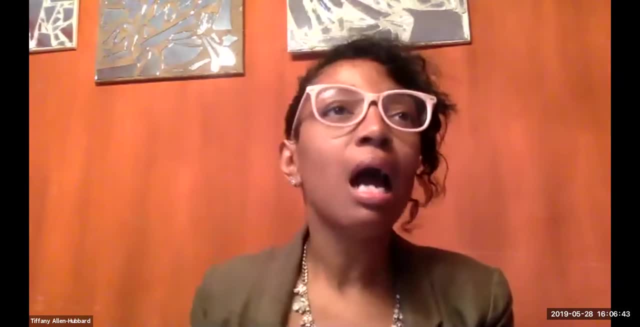 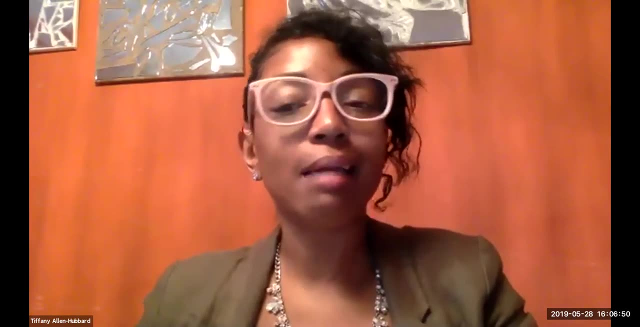 especially when they're operating in a small capacity. You know, there was this thing that happened in around the 90s- 2000s where, like a lot of the big schools that had a lot of teachers and a lot of students and the ability 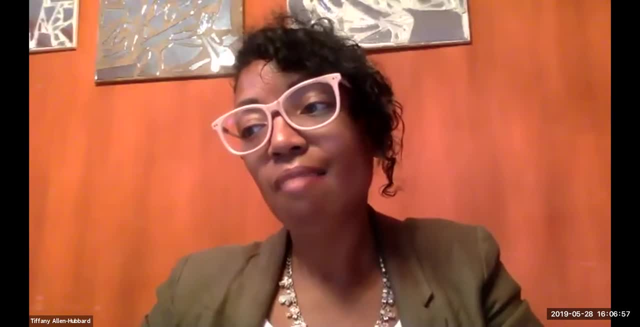 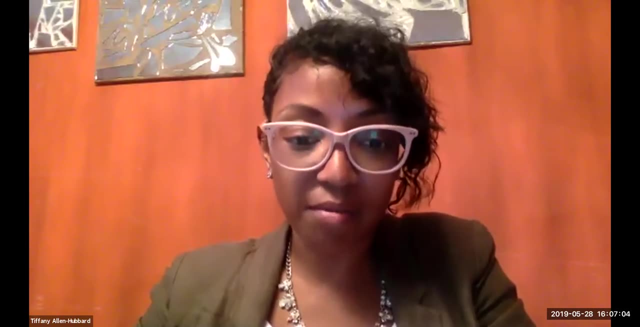 to kind of provide. these kinds of experiences have been made into smaller schools where you may have 20 teachers, you know, with a student body of about 500 kids or 600 kids, And in that way those kids don't have the same access. 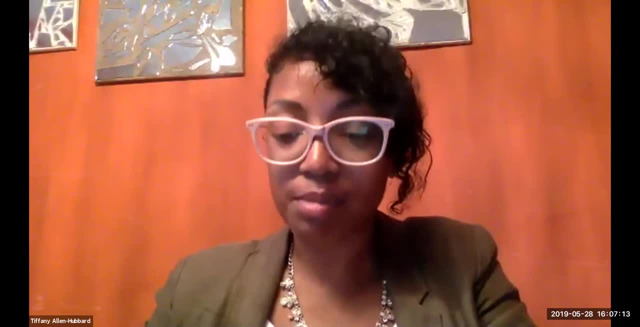 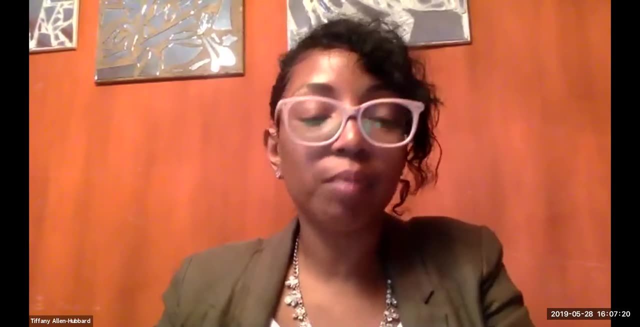 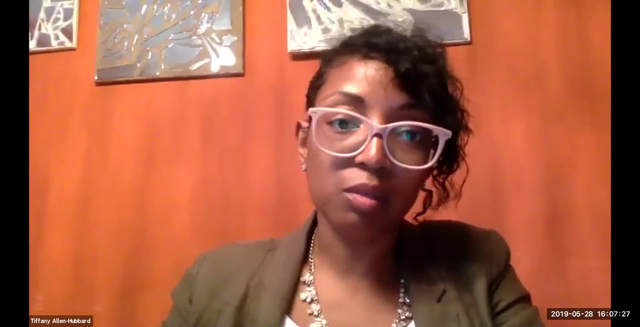 to different kinds of coursework and different types of extracurricular activities, And I think it definitely matters. So, even within the city, or even if we're looking at the state in general, this is a major, major issue. So what are the things that we can do? is the question. 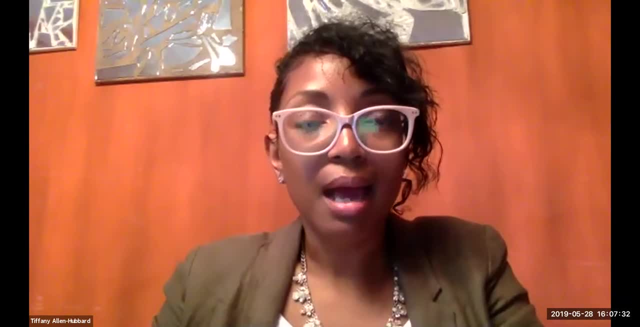 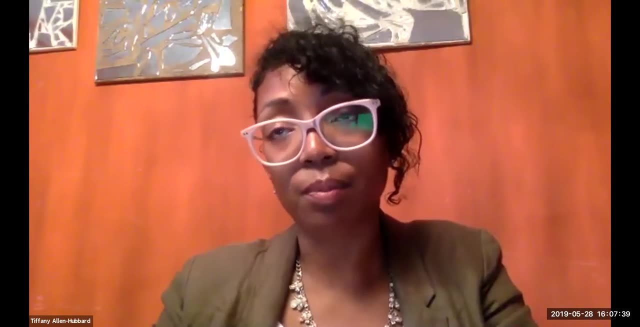 One of the things that we need to do is make sure that schools have available for at least extracurricular activities, even if they can't program within their school day, to provide a lot of support. Some of these schools, as we talked about, 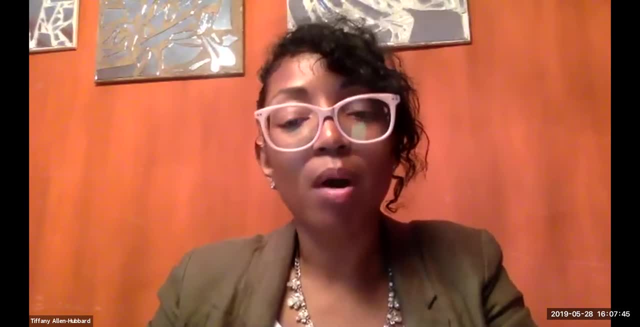 were like: maybe the smaller schools and those small schools can have partnerships where each school might run a different program, or you know, and then students can visit them. you know, and then students can visit them. you know, and then students can visit them, you know. 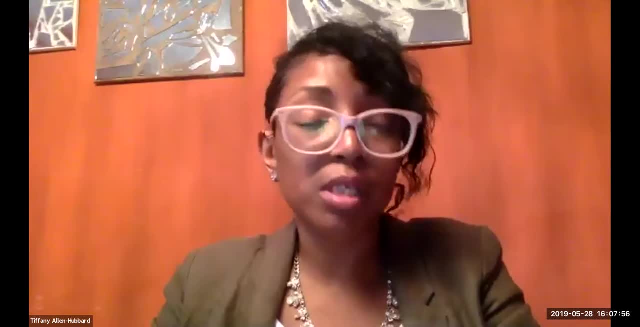 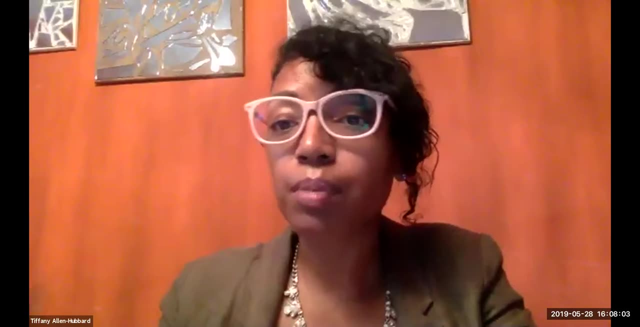 and then students can visit that program from other schools. In New York City we typically have high schools that have a campus, with maybe four or five high schools that exist in the same building, So this would be a good opportunity to have students cross-register for programs. 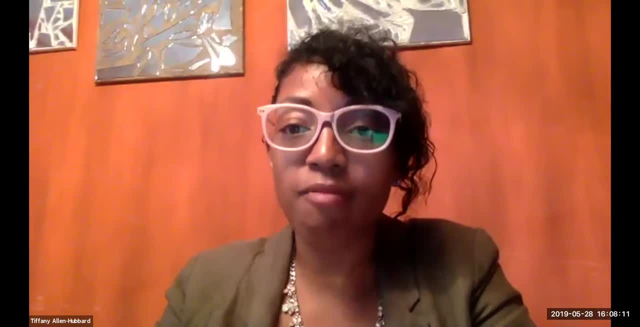 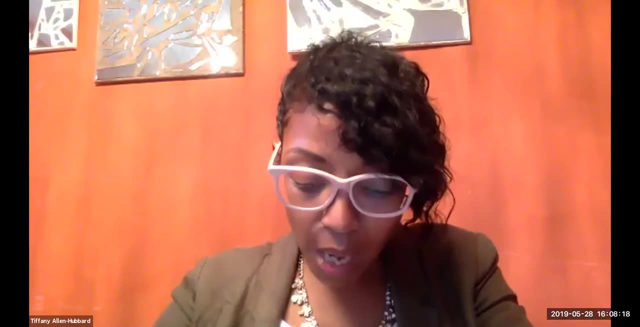 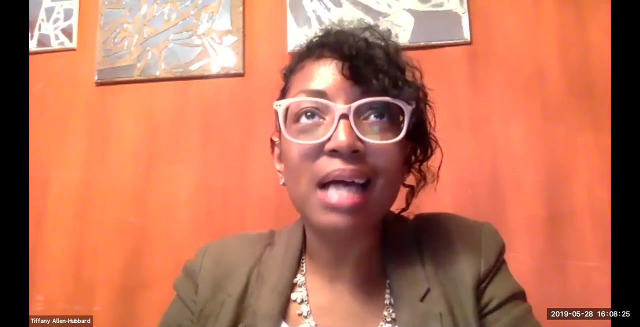 but also cross-register for AP courses and things like that that haven't been available to students, And I think that that is important. A couple of things that really caught my attention. A couple of things that really caught my attention was these ideas about students in government. 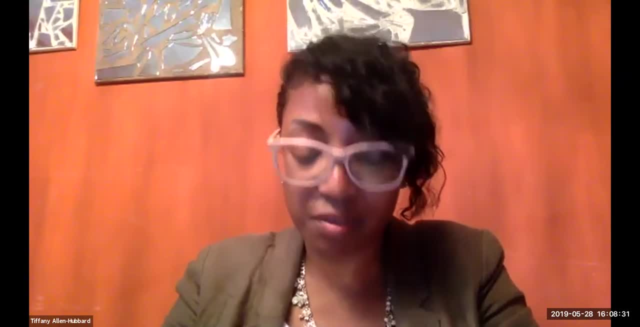 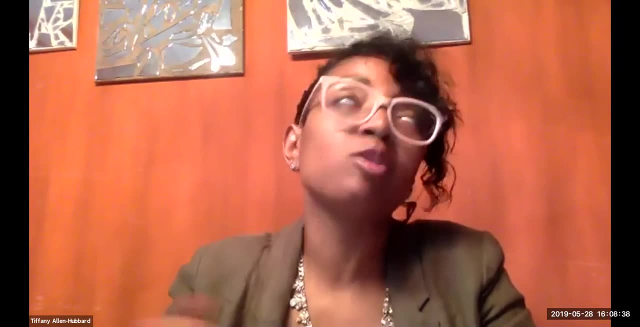 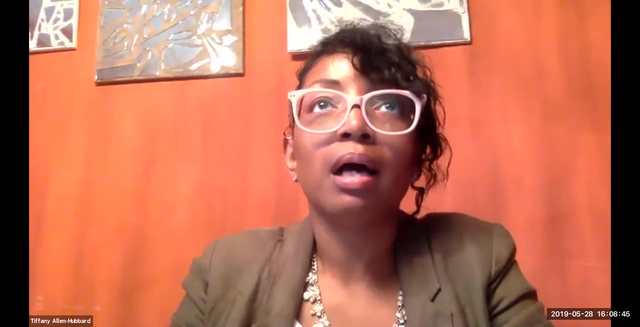 and, as Hamsa said, students really becoming vocal advocates for themselves. One of the opportunities that we can provide is the idea of, like participatory budgeting, where we actually have students involved in determining which of these extracurriculars will be supported. 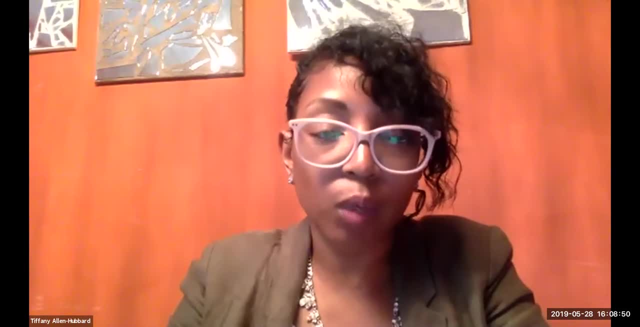 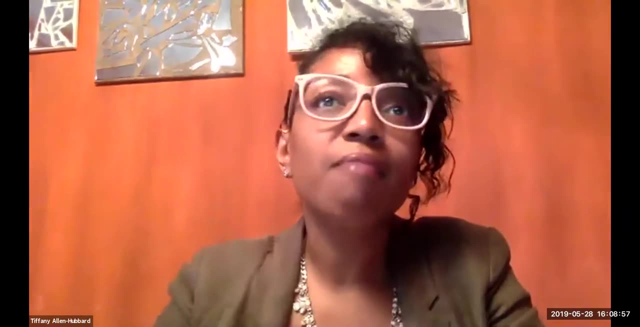 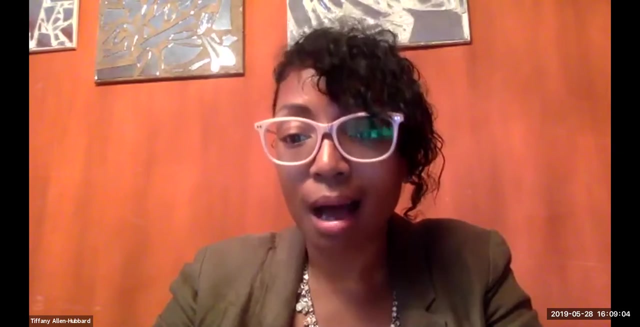 and how we will support them, So students actually determining what should happen in their school. Also, I talked a little bit before about just having functioning student governments. A lot of schools don't have those Democratically elected student government where students like Hamsa and other students 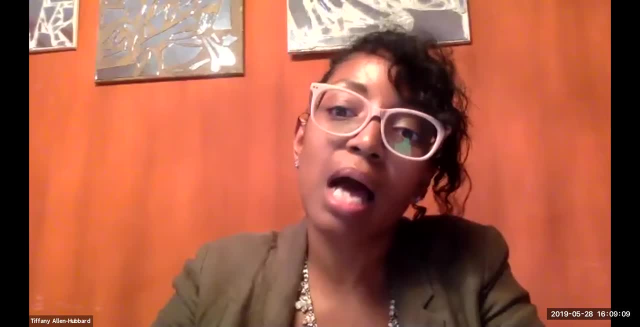 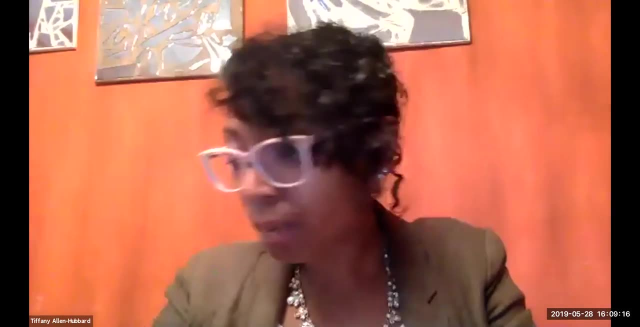 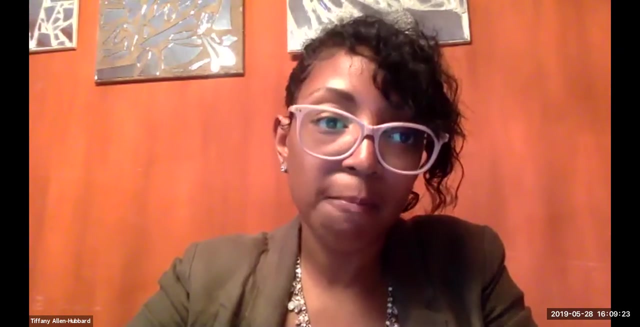 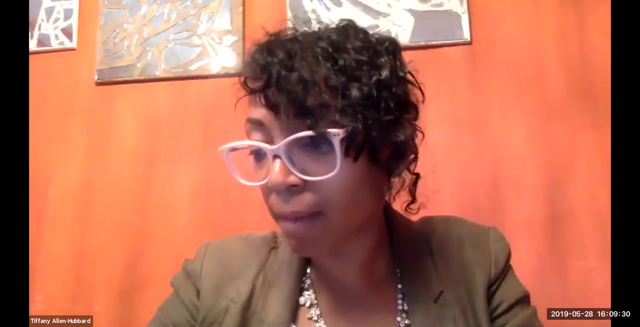 can really have a grassroots kind of emphasis and talk to their classmates and kind of increase awareness. Another thing that I brought up and I think is important is the idea that students they need to be able to see education from multiple perspectives. So even if we had some sort of program where students could 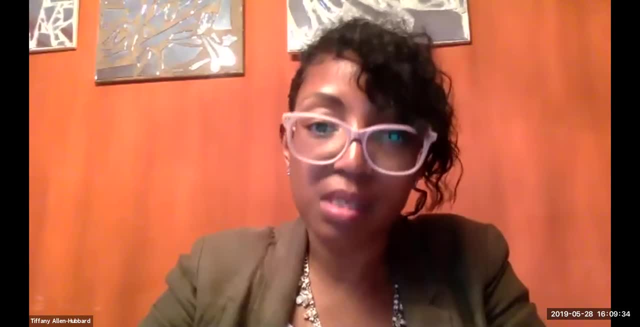 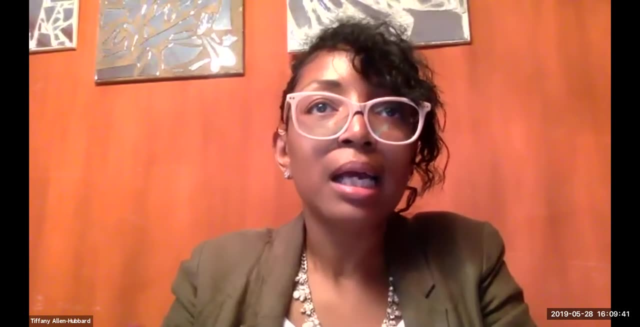 if they are participating in student government, that those student governments can visit other schools to see what is on the agenda for other schools and how they operate. I think it's important to kind of have that kind of energy where schools are sharing the great things that they do. 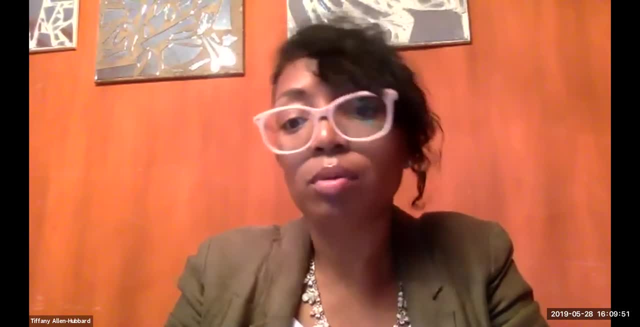 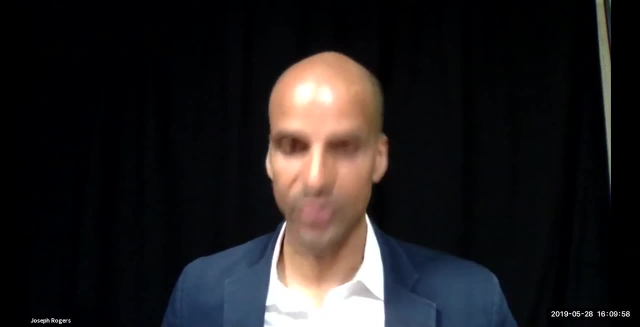 and students are well aware of what's going on in their schools and in other schools as well. Great, thank you, Tiffany. I appreciate it. A couple of things, Well. first let me say here because I know some of our members of the public: 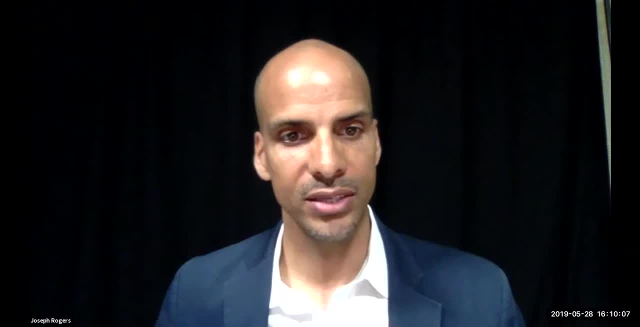 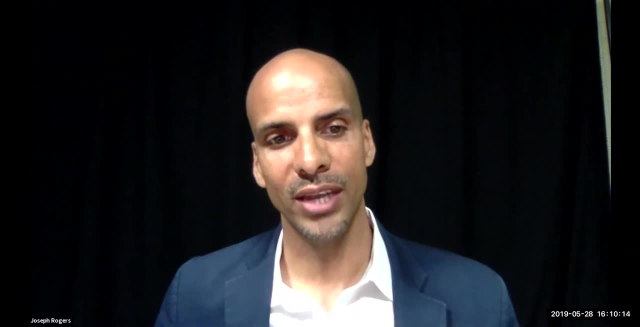 some of our education stakeholders who are with us here today, and it looks like we have around 60 or so, which is a good number. One of the things I was remiss in doing at the beginning of the conversation was to make sure people knew how to use the tools. 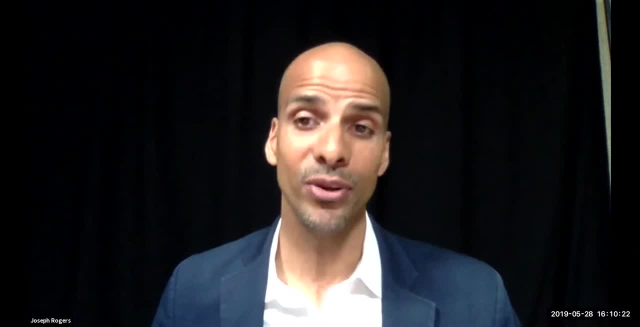 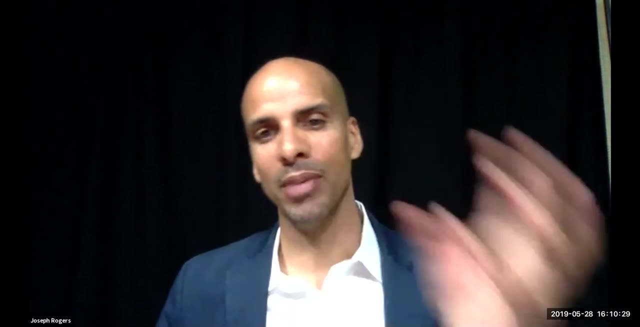 at the bottom of the webinar screen. So those of you- I see some of you are chatting it up in the chat box at the bottom, You'll see. you should see at the bottom of your screen a little bubble icon with three dots. it says chat. 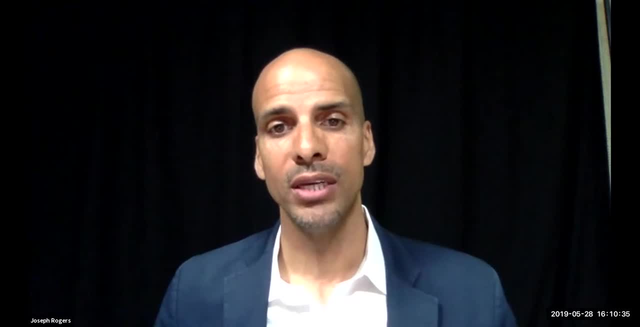 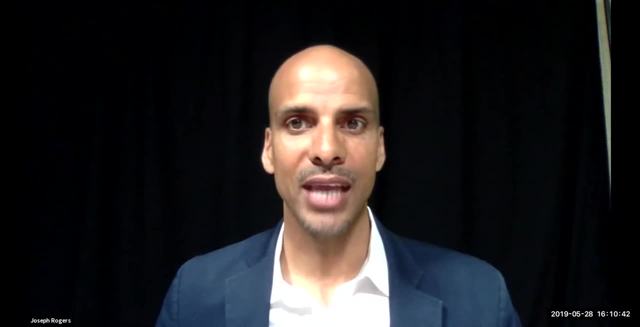 That's where you can one request help if you need help, tech help. you're new to the platform, this particular tech platform. I should mention that Cassidy Grubbs- Cassidy is our support person for the webinar here today and she's managing the chat box. 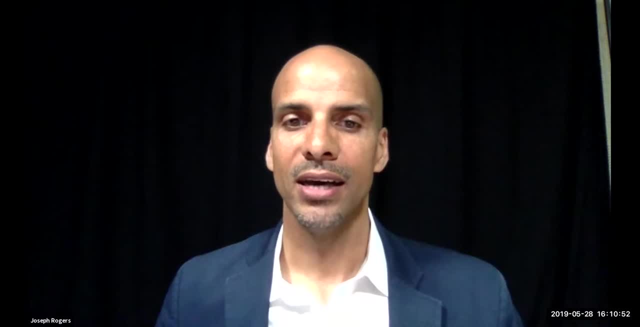 So for those of you, thank you, Those of you who have been commenting and hearing responding to some of the things you've heard our panelists say, please continue to add to the chat box any comments. I will transitioning because we're about to pause here. 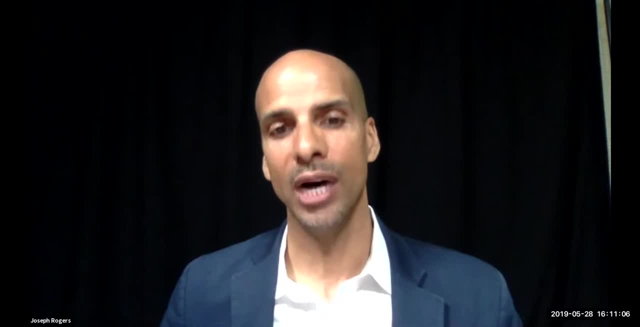 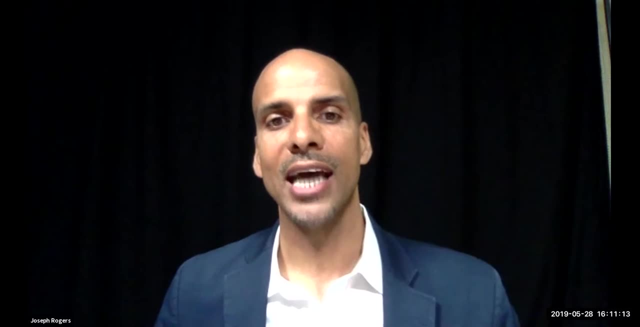 I want to make sure that you also know that we have a Q&A button. there Again, at the bottom of your screen, you'll see a button has a large Q stamped on it and it says Q&A. That's where you want to submit questions. 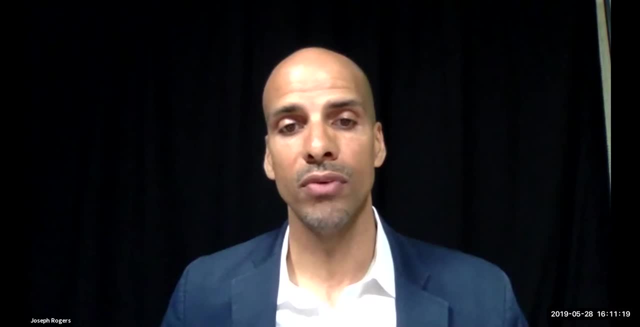 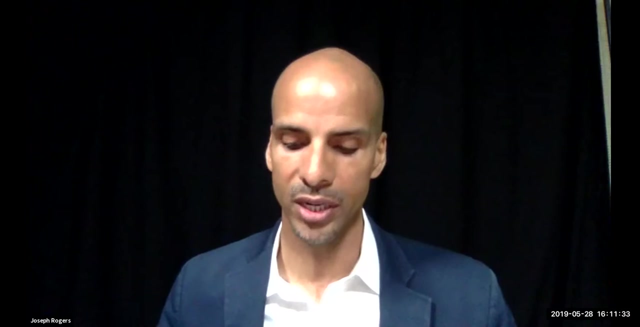 for the entire range of stakeholder representatives with us today. Or it could just be a broad question about equity in civic education, ideally one related to the research findings, the constitutional right or some of the specific proposals and questions. you've heard our featured stakeholder representatives. 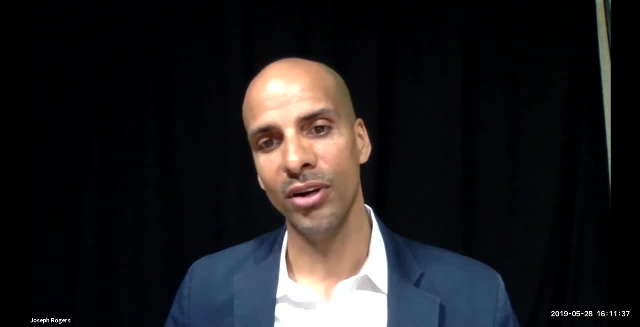 share with us here today. So you have the chat box again for just a comment on what you're hearing. You have a Q&A box at the bottom there if you'd like to pose questions, And you can start doing that, not just for Tiffany. 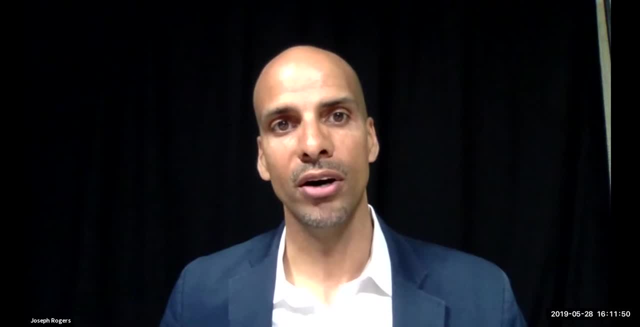 but for Humza and for Leah as well, And ultimately for our final two stakeholder representatives, And then we're going to broaden the conversation- I actually have a question for you- And then we're going to try to get to at least a couple of the questions. 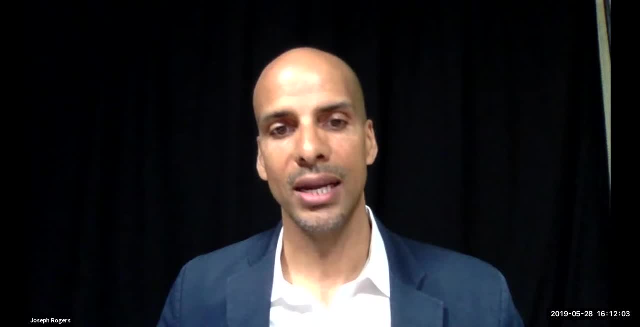 that you submitted through the Q&A box. Again, we'll be looking at that box to pull questions. So if you enter them in the chat box before I had a chance to point you to Q&A, please go ahead And it won't be redundant. 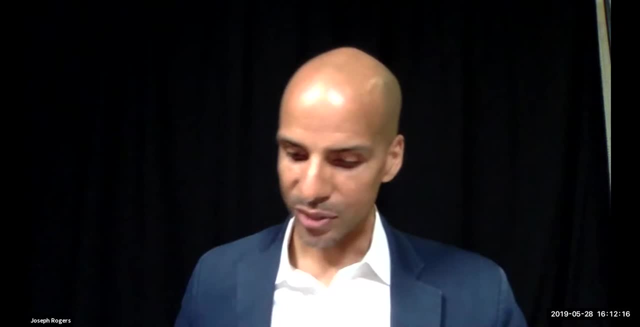 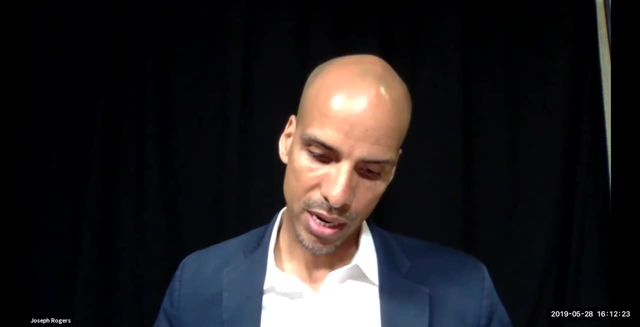 Go ahead and enter them in the Q&A box. So, Tiffany, thank you again for your contributions to the conversation here today. I already have a couple of things. A couple of things jumped out at me. You talked about staffing and how you feel like where you are now. you 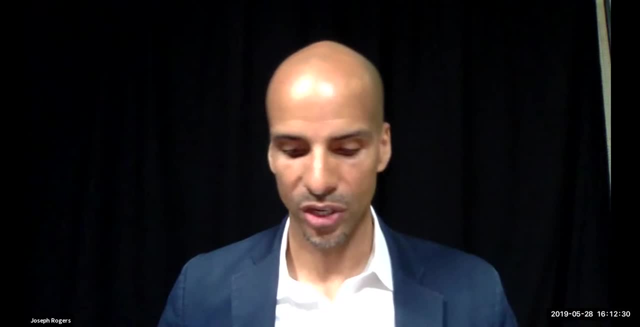 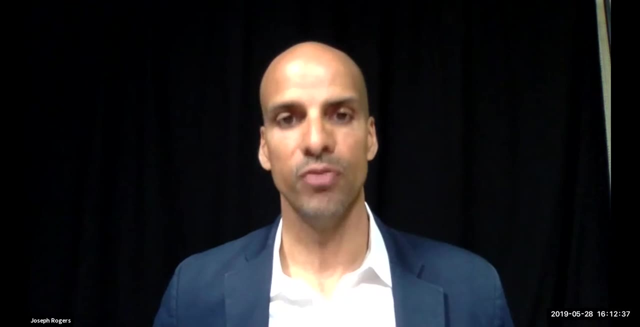 have a wide range of courses. You have the kind of extracurricular opportunities that many of our young people need and deserve And you talked about. in some of the other schools you've been in. they didn't have the staff capacity, They didn't have enough staff or staff. 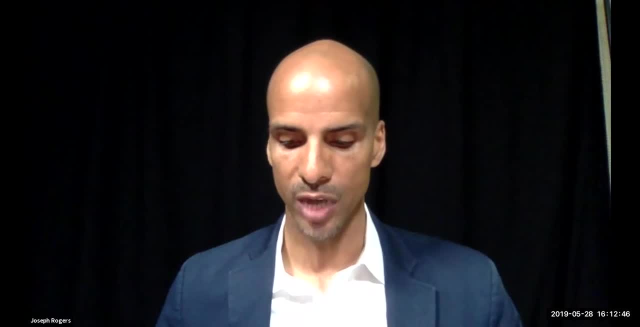 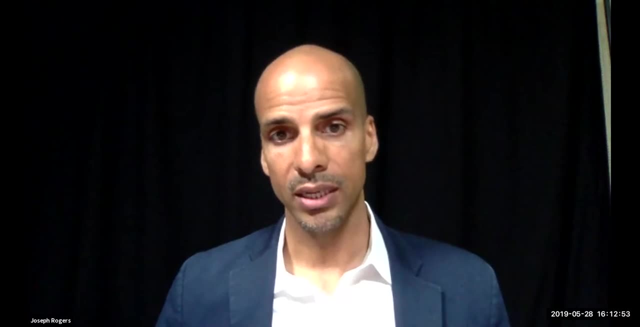 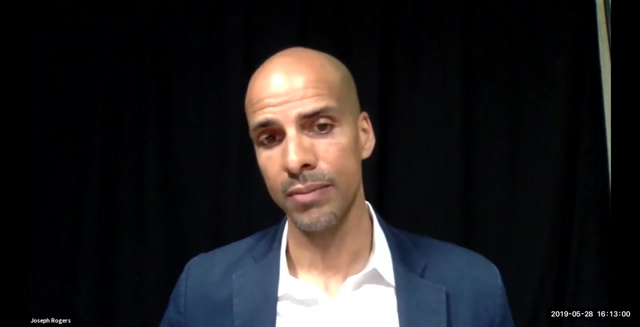 with the right certification or qualifications to be able to provide some of those opportunities: Elective courses in civic learning or clubs. again, these things take resources and it's not one thing to say students should have them. It's another thing for schools to receive the resources. 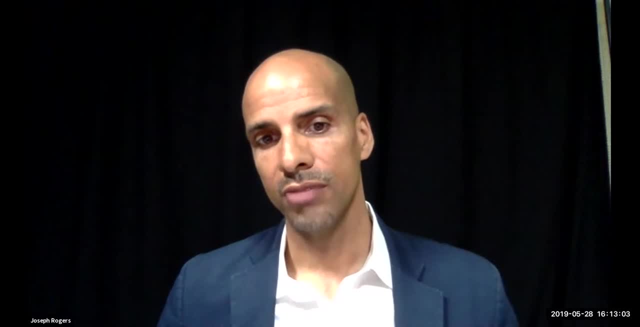 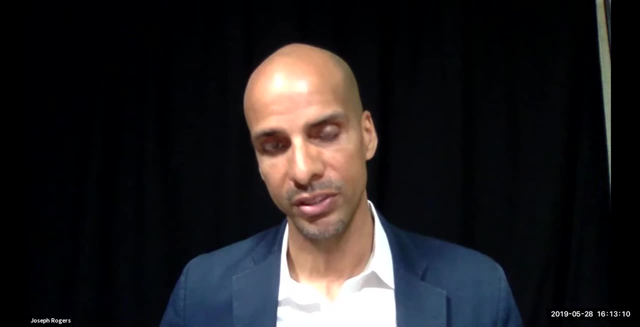 But also sort of the policy, guidance and structures from our state and from local districts toward encouraging schools to do more of this work and helping them to develop models, As Tiffany mentioned. one of the models she recommended is with schools where you have buildings in which schools share facilities. 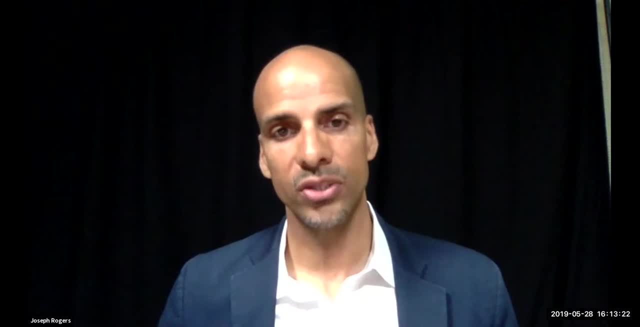 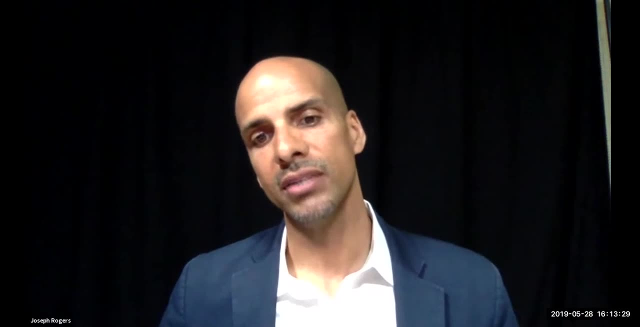 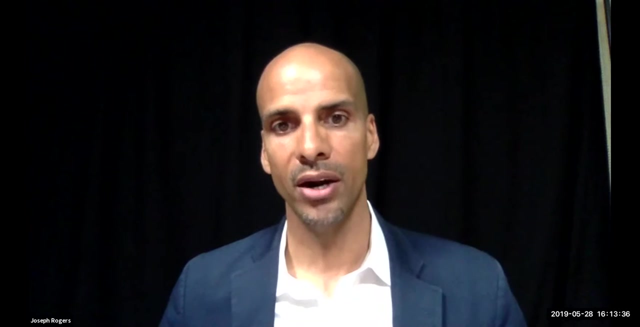 We call them co-located schools. Hello, Yes, can districts or the state ensure that- and that may be very New York City specific in some ways, may be specific to our large urban districts- what can our states and district do, what kind of policies can they implement toward ensuring that it's easy, not not cumbersome, to share? 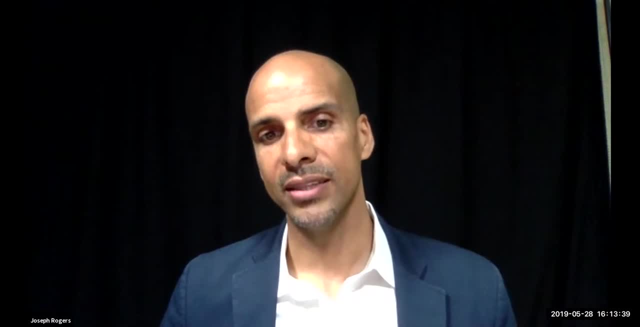 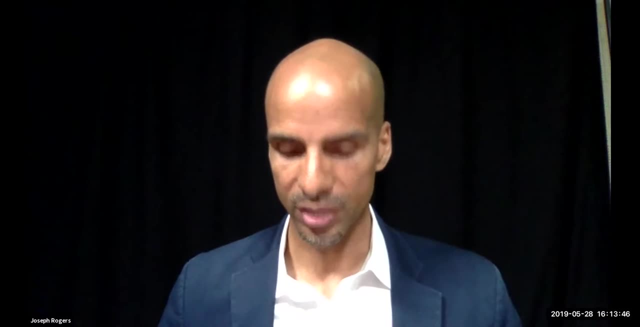 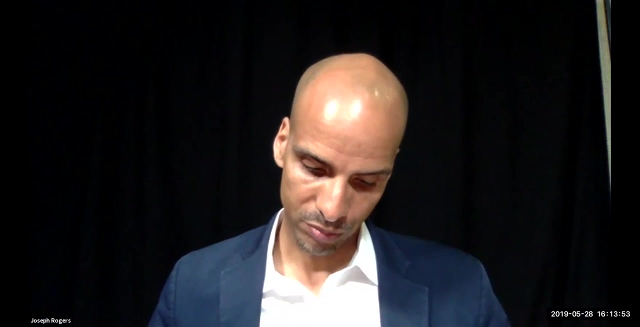 coursework, to the extent that that's appropriate and to the extent that it truly does provide every single student in those schools, in each of the schools, the opportunities that they need in order to develop these skills and acquire these: the knowledge to become effective civic participants, to become civic ready, and you talked about also. in this case, this has some policy. 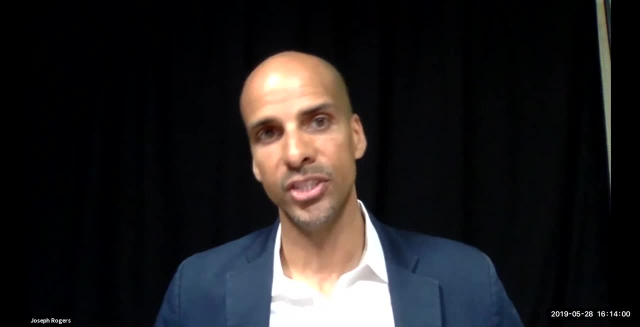 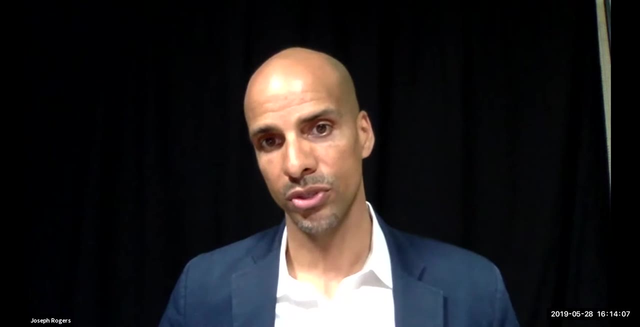 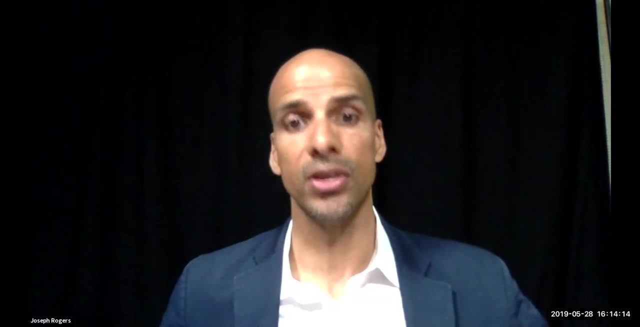 implications. also, you talked about making sure schools are able to visit each other or or staff and students. maybe parents also from schools are able to see what other schools are doing, to learn from their models and to really develop relationships toward improving opportunities for students at all of the schools in our state. so I know I've heard other people talk about that. 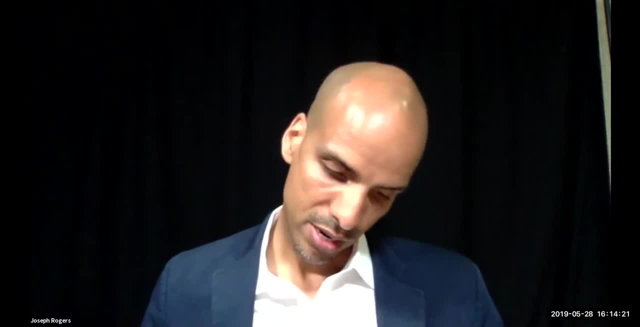 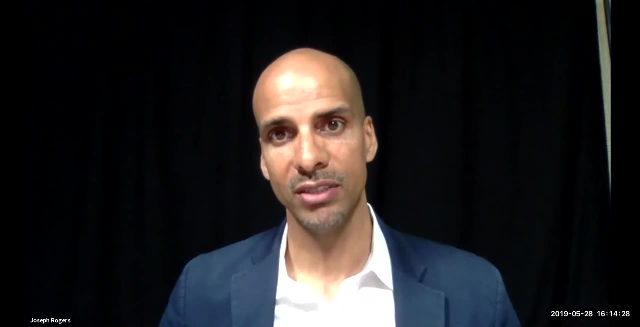 this keeps resurfacing, but I'm glad you introduced it here. you also talked about participatory budgeting, again harkening back to what some of the hums's recommendations and some of the actions he's taken around getting young people, giving them an. 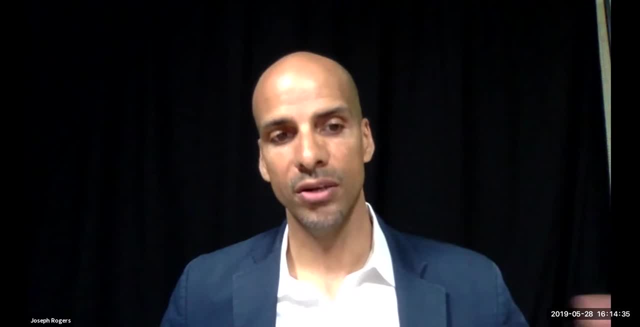 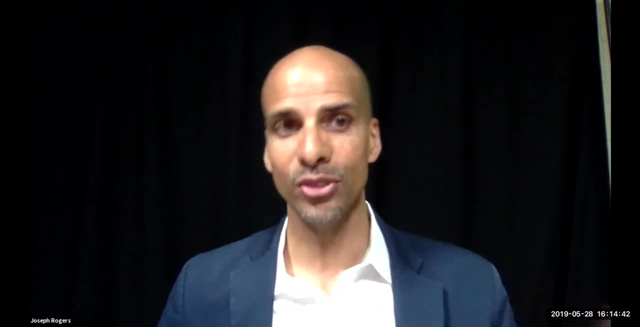 opportunity to weigh in on what kinds of extracurriculars and courses they would like to see and that they believe they need toward preparing them to be civic ready, not so that they're choosing between you know the many things they, all of which they should have. 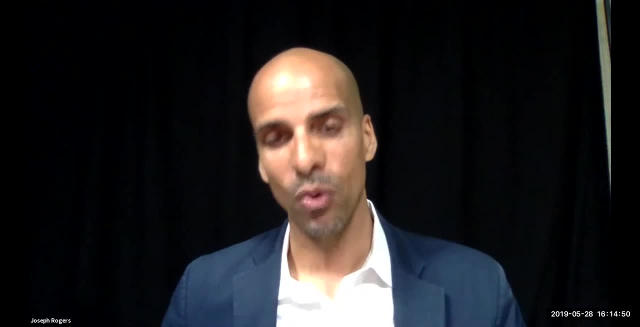 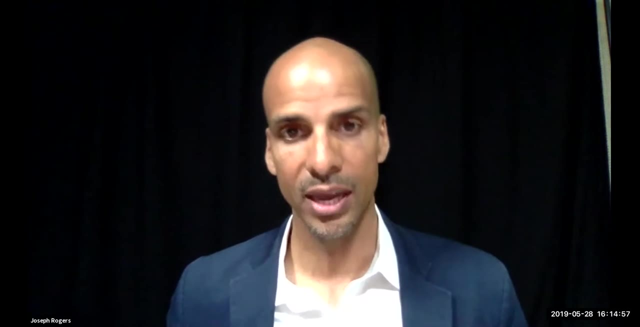 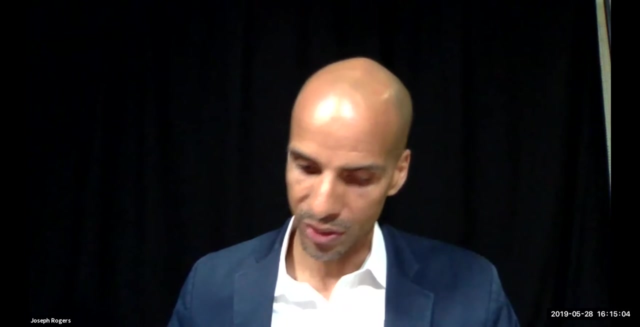 right. it shouldn't be a false choice, but they should have a wide range of options and have some significant say, should be able to drive some that decision-making. so thank you again, Tiffany, for sharing an educators perspective here. with that, I'd like to go ahead and turn to- and I do see. thank you everyone. I see you continuing to chat. terrific, please keep. 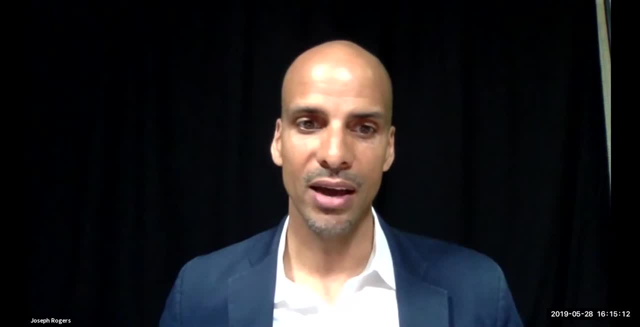 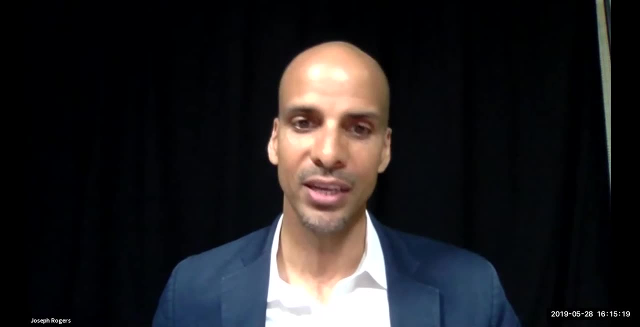 the comments coming in again. Kasky is managing that box and I see we have some questions coming in as well and I'll have a chance to take a look at those to see if they're for specific individuals or maybe broad questions. I see we. I think we're up to about six questions now. please continue to submit. 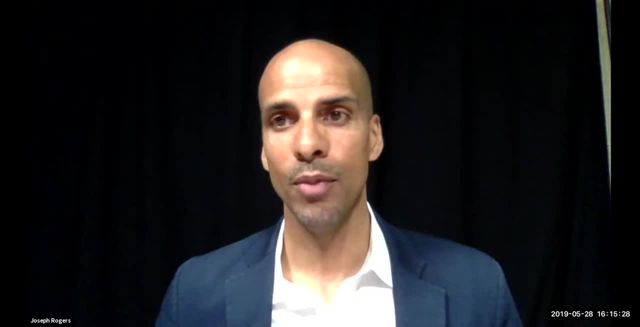 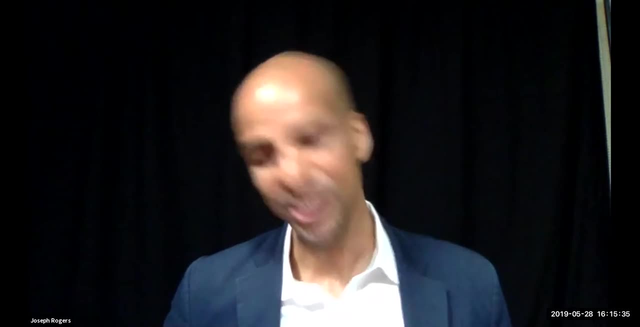 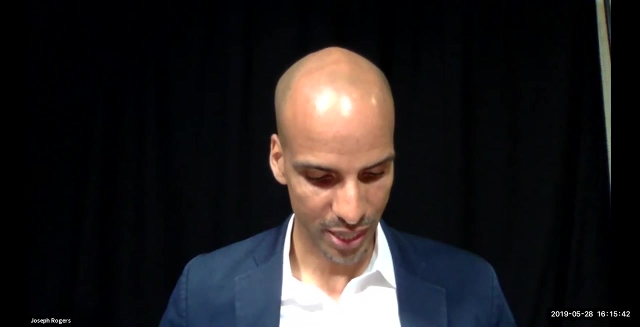 questions and we'll try to get to as many of them as we can in the time we have here today. so, with that intermission, with that, I'd like to go ahead and turn to our next featured stakeholder, and that is miss Deanna Vasquez. and Deanna, again it comes to us as the state coordinator for the 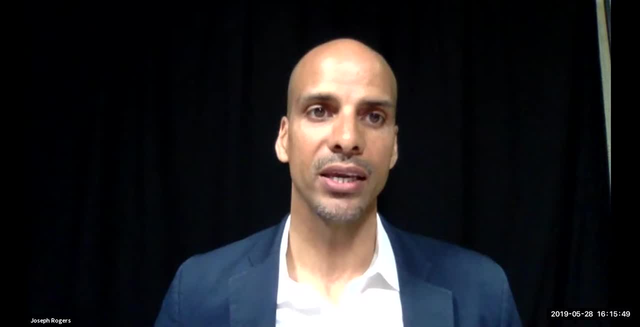 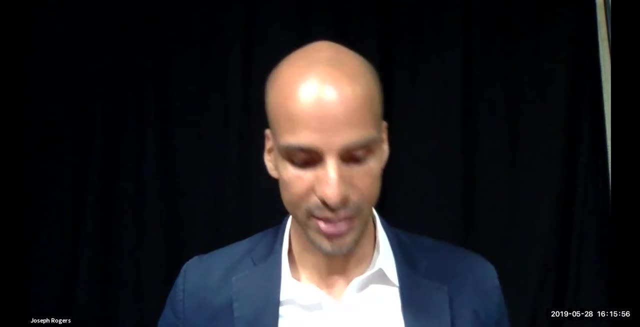 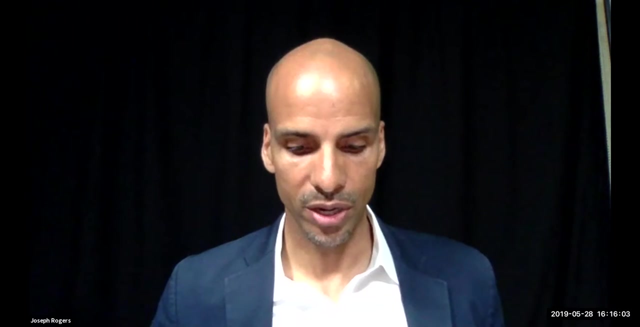 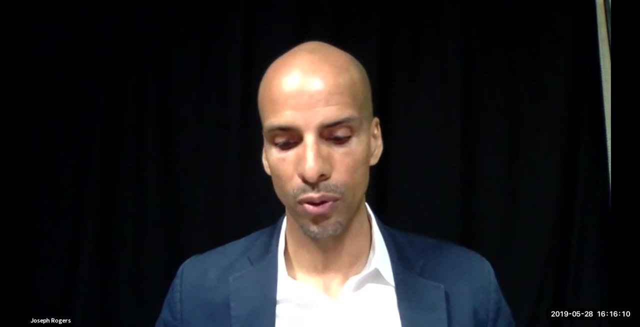 Angelo del Toro, Puerto Rican Hispanic Youth Leadership Institute. Deanna, I'd like to ask you, if I may. some students benefit immensely, we know, from participating in rich hands-on experiential civil civic learning experiences and youth leadership programs beyond their schools, the community setting and otherwise. many of these programs help young people acquire. 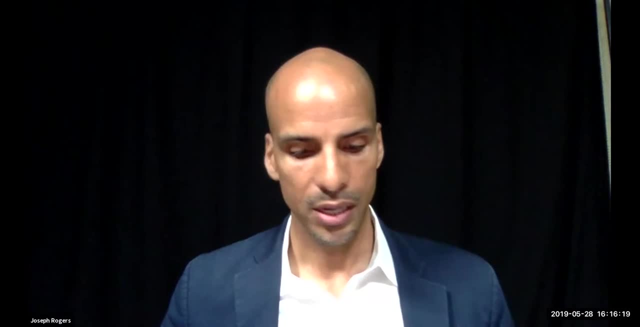 a real-world understanding of the political process. just to name one example, What can schools, districts and or state officials do to ensure that all New York schools are able to offer similarly rich civic learning opportunities so that all of our young people are prepared for active and effective engagement in civic life? Why does that matter? Why does the work you're? 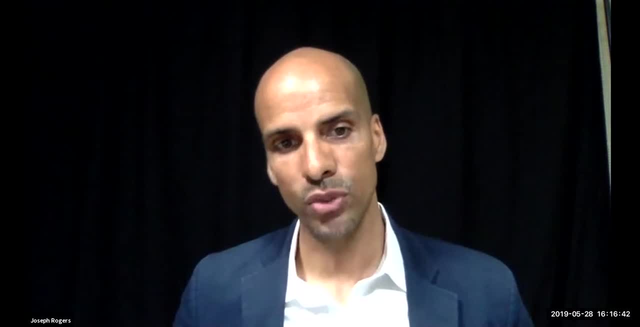 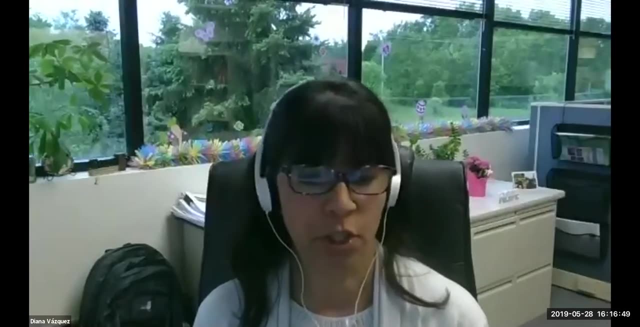 doing and that perhaps more schools would do if they had the resources and the guidance. why does that matter? for our young people, for their civic readiness. Good afternoon, everyone happy to share what highlight is all about with you. I'm going to give you a little bit of background of our program. 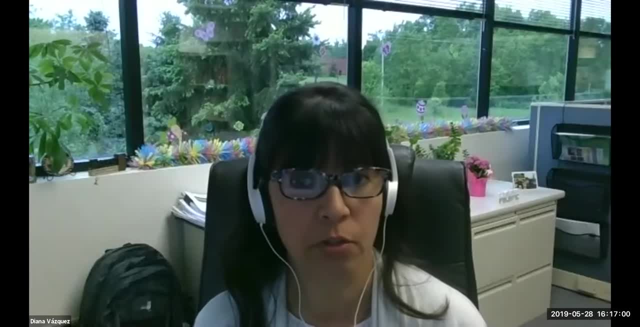 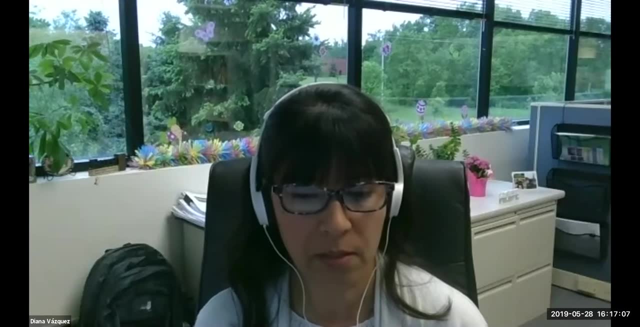 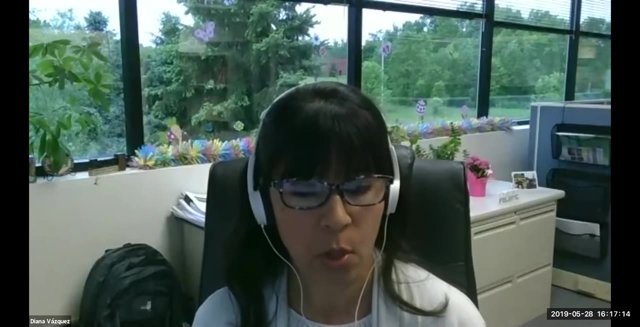 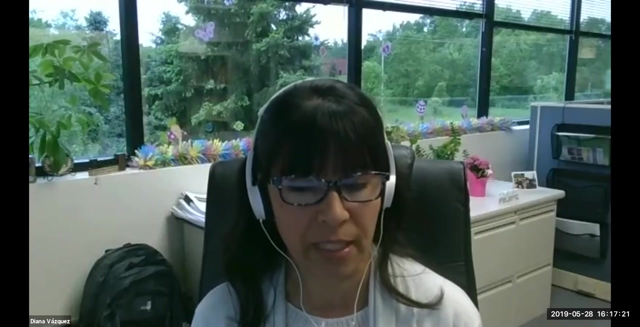 The effectiveness of the Angelo del Toro Puerto Rican Hispanic Youth Leadership Institute has been documented effectively for over 30 years of history. This inclusive, cultural, responsive and interdisciplinary training model has empowered young Latino leaders who think strategically and globally. The Puerto Rican Hispanic Youth Leadership framework is extremely effective. 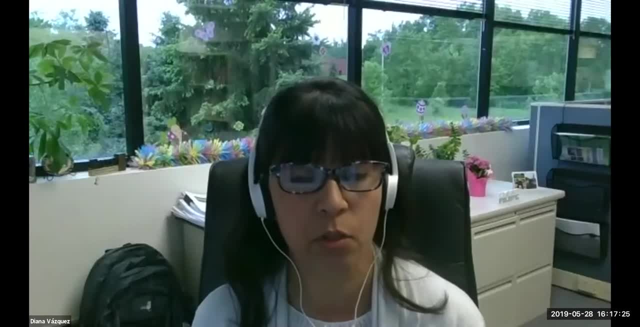 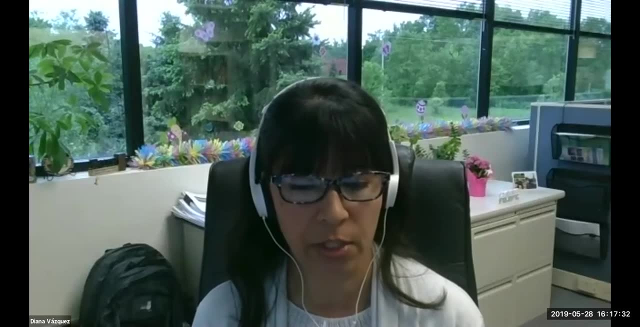 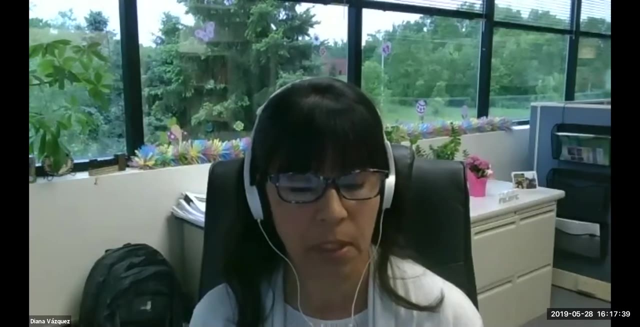 design for implementation in the wider context of school communities. The core of this design is the collaboration and interaction between students, the facilitators and the curriculum. This framework can easily be implemented to include content area teachers across curriculum, especially for social science and language arts, Once the teams of facilitators 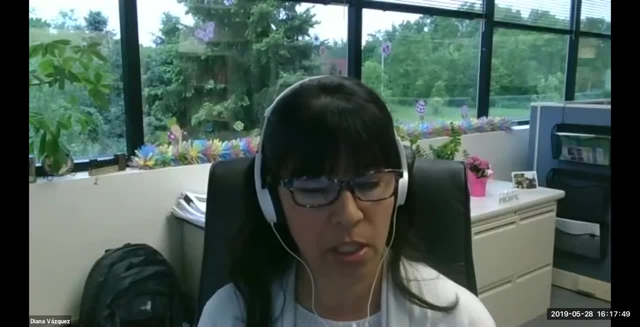 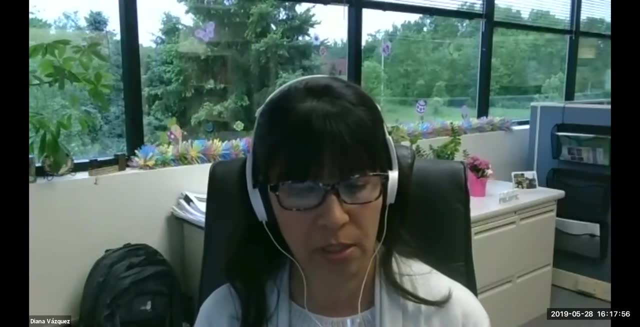 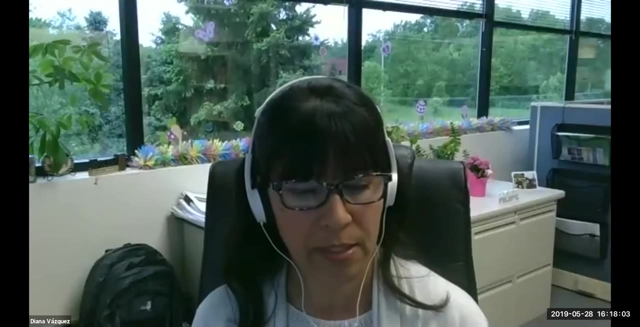 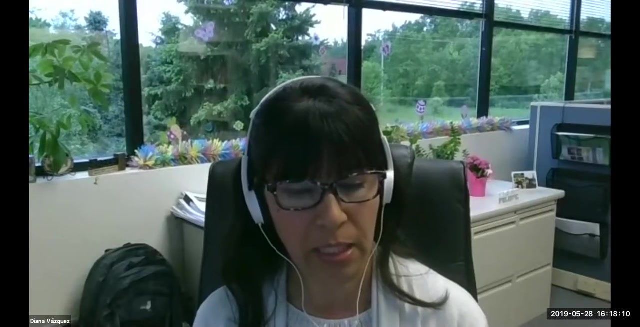 and content area teachers are established. then community building occurs within the classroom. The Prylight curriculum is easily expanded to include not only issues in government and interest to the Latino school community. The focus can be really expanded to include various ethnic, civic and other concerns as well. The skills of focused discussion, questioning, critical thinking. 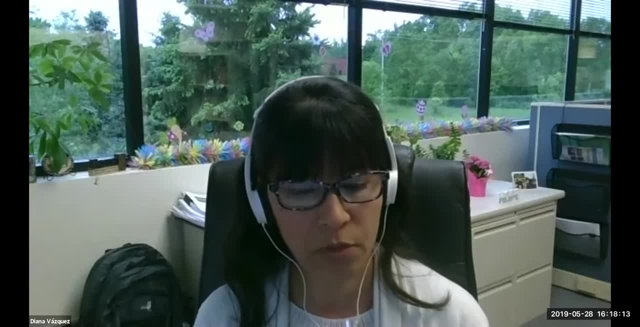 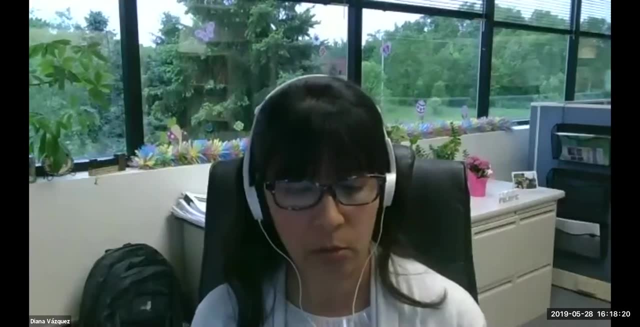 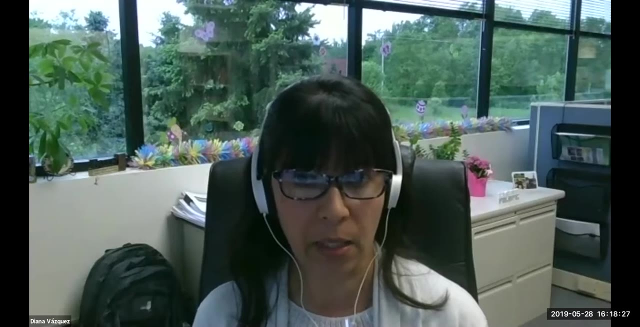 and analysis are indispensable and paramount to all students in classroom across the campus. The Prylight curriculum is also a tool to help students to think critically about local, state and global issues that formally consist evidence-based arguments, both verbally and written. These critical thinking skills are then practiced and redefined in 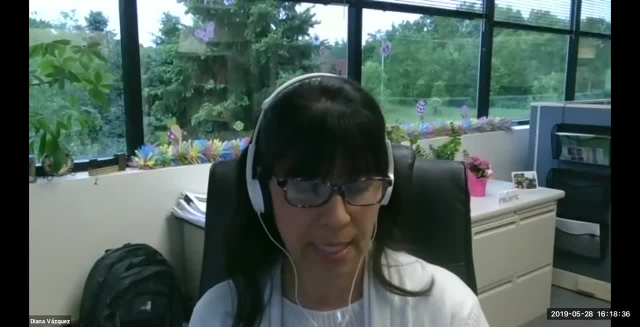 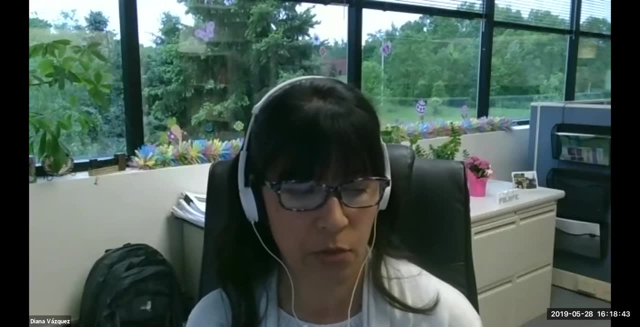 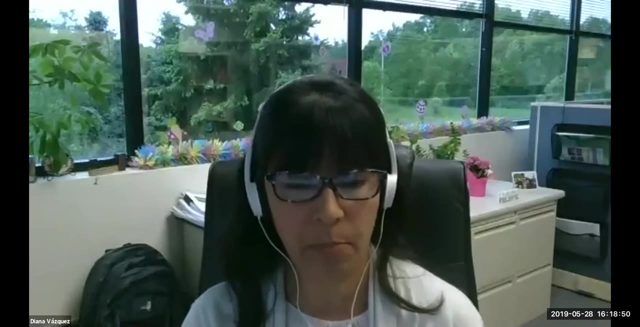 discussions and debates in small and larger group settings. Students have the opportunity to read a wide range of bills and discuss with peers and facilitators regarding the text of these bills and research directly related to them. They also annotate paraphrase and formally sophisticated. 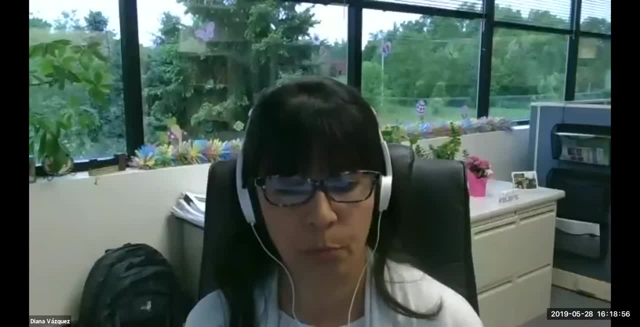 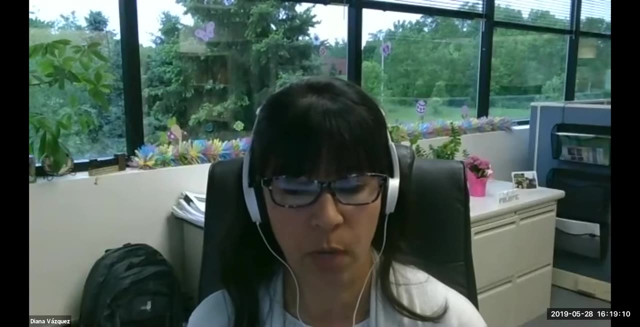 arguments based upon the bills and research to support the stance or argument. They can and are required to take the role of those who oppose their position. in order to look at the bills from all perspectives, They become global thinkers, readers, writers and civic leaders. 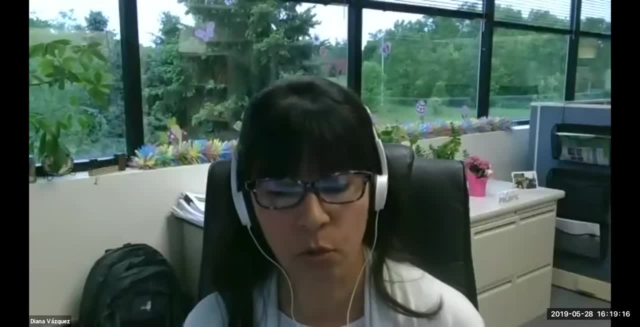 The multi-grade and multi-ability dimension of Prylight is also worth noting. There is a responsibility inherent in Prylight participation that could be fostered in larger school communities, with 9th and 10th graders being mentored by 11th and 12th. 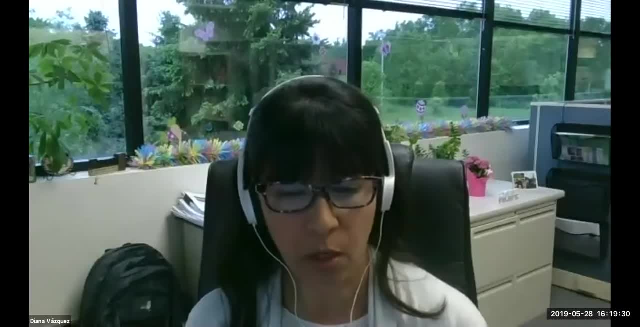 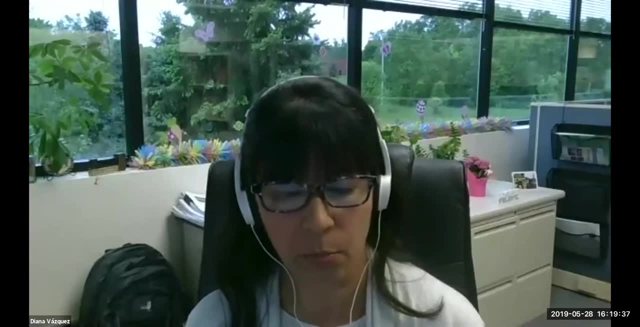 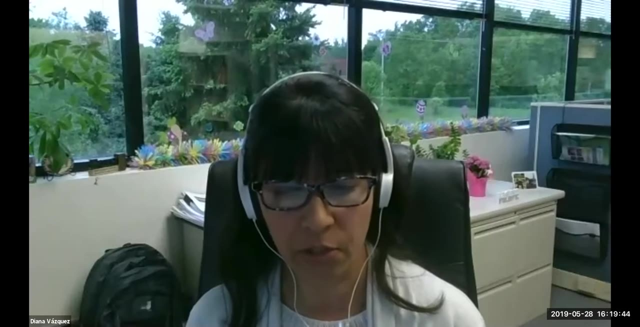 graders, returning students. Learning about the inner working of our government is a way to ensure the future generations are aware of how they can spark changes within the communities, as well as advocate for themselves and others. One way for schools to allow for this same understanding is 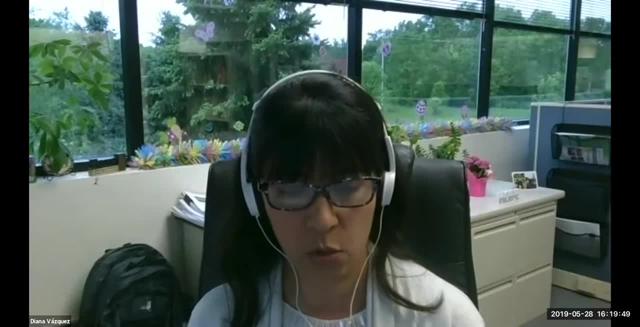 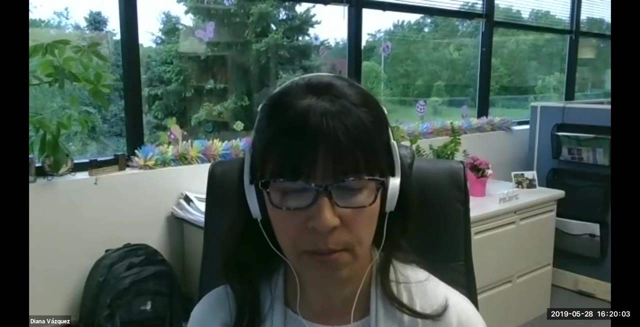 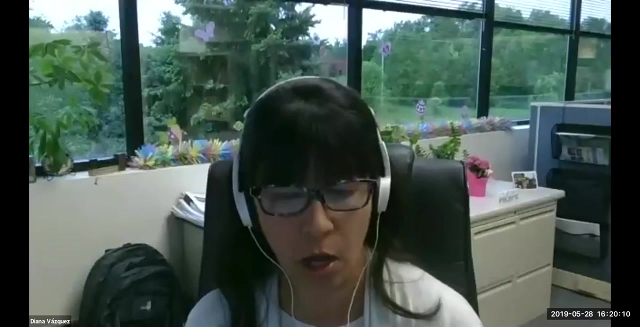 to have students study the law-making process using current relevant events and bill as examples, Additionally allowing students to conduct research on current topics of their choice in order to spark professional debates in the classrooms. Creating a hands-on experience, rather than textbook-based experience, for studying law and law-making process is part of what makes Prylight. 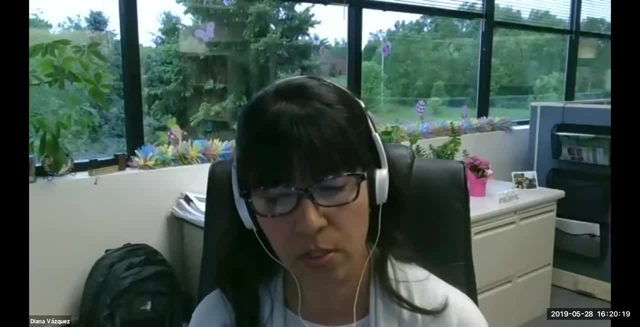 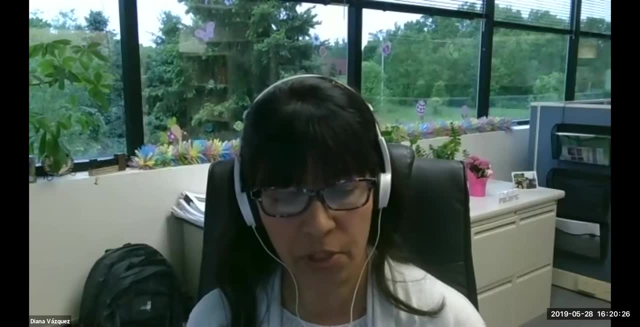 so valuable for us. Mr Vianna, I want to thank you for your time. I'll now turn it back over to you. Thank you, Deanna. I'm glad to be here. First of all, I want to thank the faculty for their 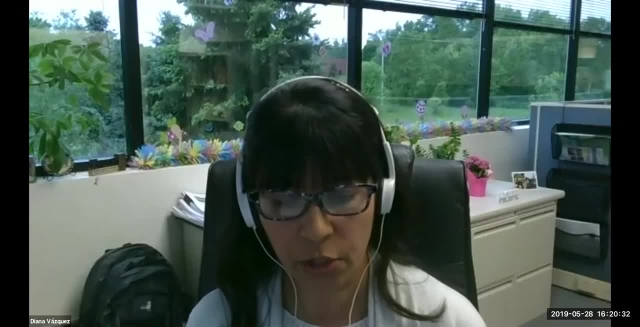 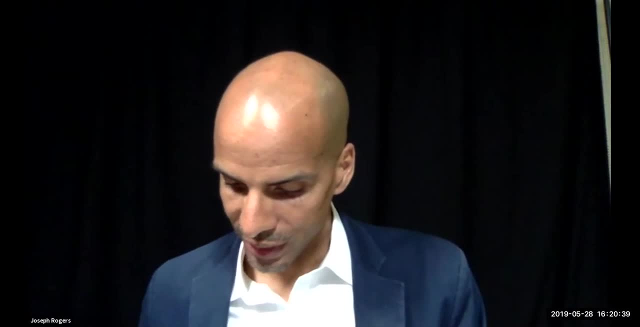 great work and support. I've been a student at Prylight for a long time. I've been attending some of the higher education classes here at Prylight. Many of you may know that I've been teaching the inaccessible history curriculum at Prylight, which is a little bit different. 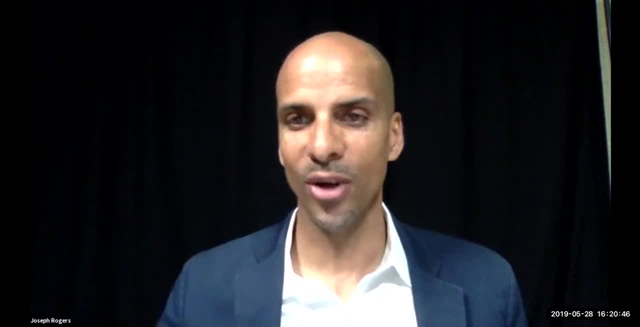 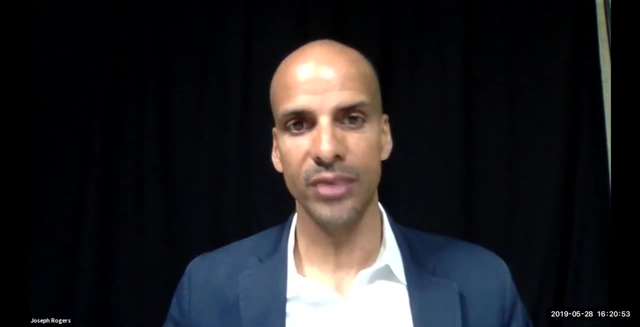 continue to come in. It looks like one thing I just saw. I haven't seen all of your comments, I know Cassidy has, but one thing I noticed there is- you're right, I think someone mentioned that- the study that we focus on the Center for Educational Equities Research Study. 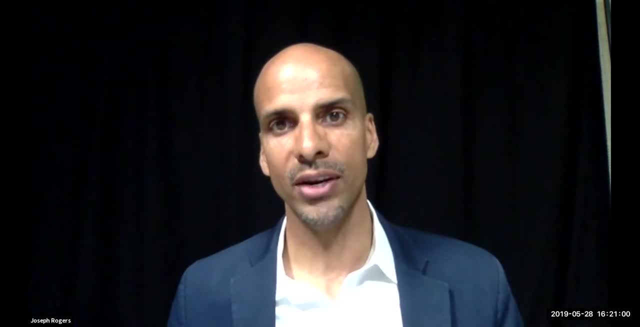 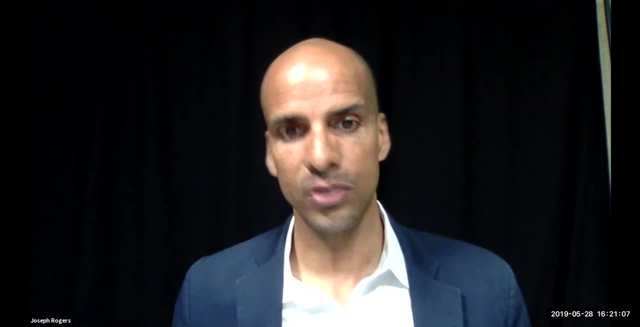 does focus primarily on high school and some of the opportunities you're hearing here are from a high school perspective, but this is a broader conversation. So I think, as we, you know, as we think about Diana's description of Prylai, or the Puerto Rican Hispanic Youth Leadership Institute, 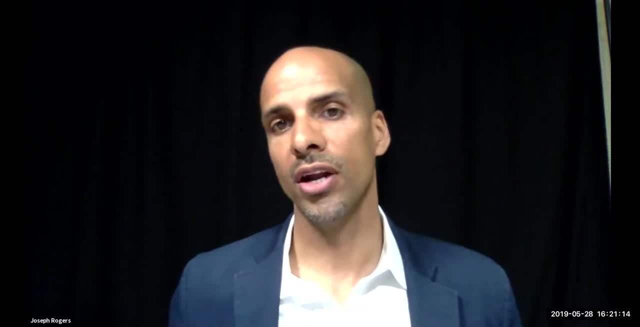 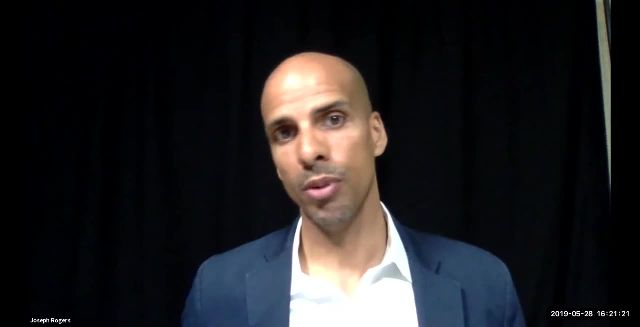 we should also be thinking about how do we make sure that our young children- you heard this also from Leah, I believe, earlier- how can we make sure that our young children, from an early age, are fully prepared and have access to not only the text? Diana, you mentioned the text not being 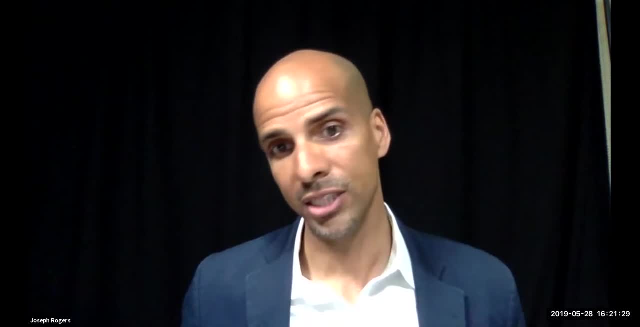 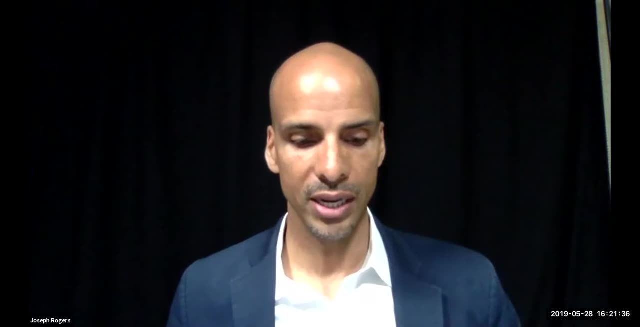 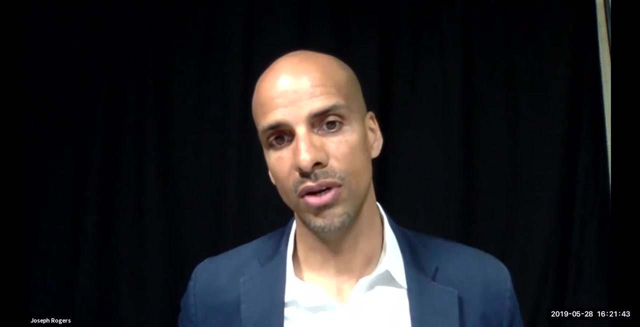 sufficient that all of our young people, again from all ages, need access to experiential hands-on opportunities. I think each featured stakeholder here today has commented on A couple of things. you really drove home- for me at least, Diana- how this hands-on experience, this really rich experience with legislators. 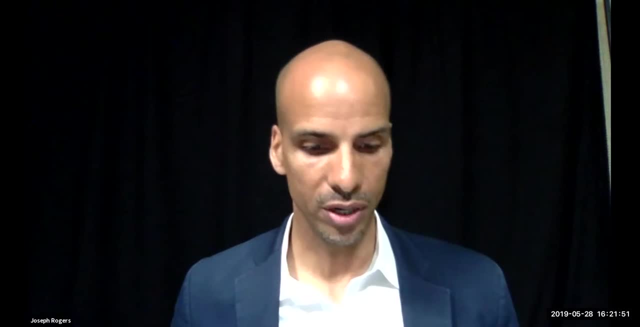 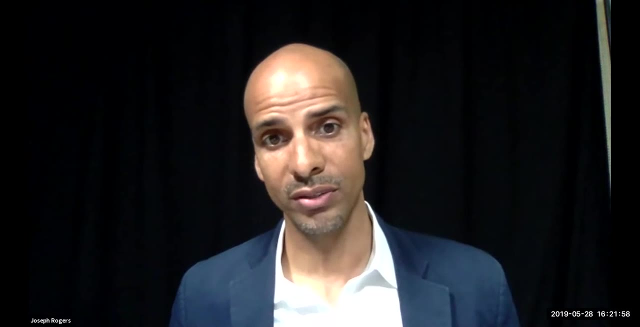 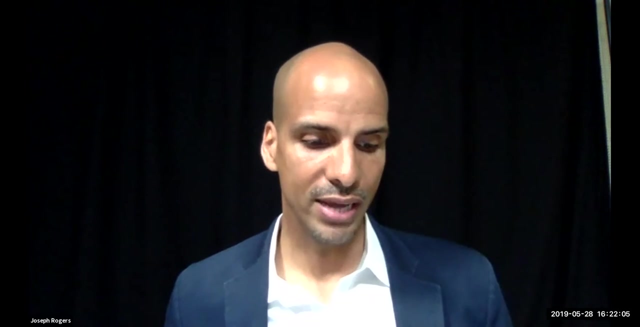 with the legislative process prepares the young people you serve to become active civic leaders. You talked about how they actually develop bills. right, They've developed legislative bills and they get to understand the political process through that lens. You talked also about how they examine issues from multiple perspectives and that's so critically important, We know in. 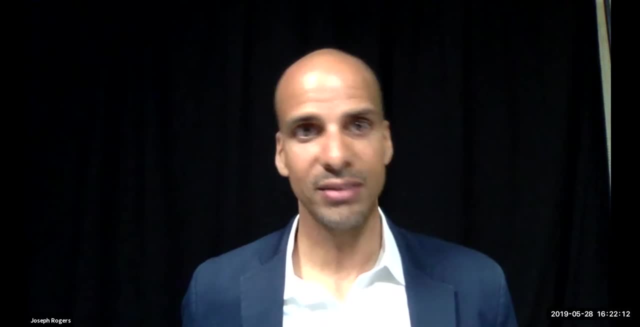 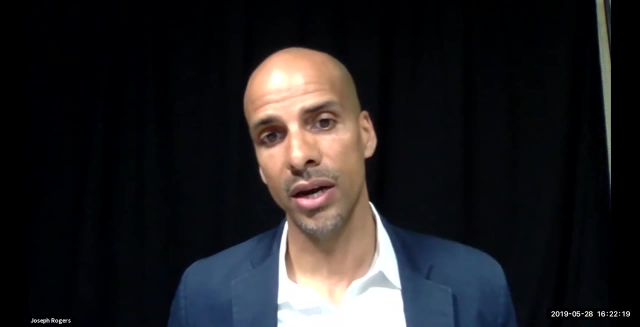 today's sort of fraught political climate, sort of this tense environment we're in, where very rarely do you hear civic leaders, electeds and otherwise, listening to other stakeholders, those who may have opposing views. So what better way and what more important and early way to make sure our young people have 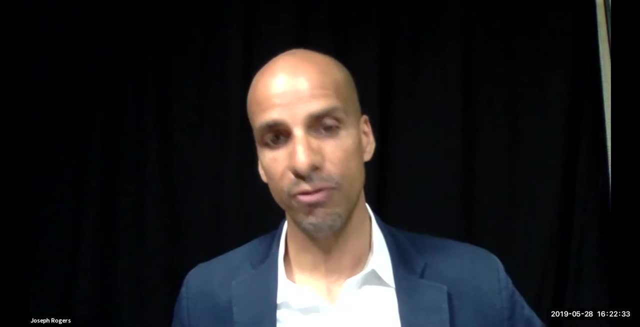 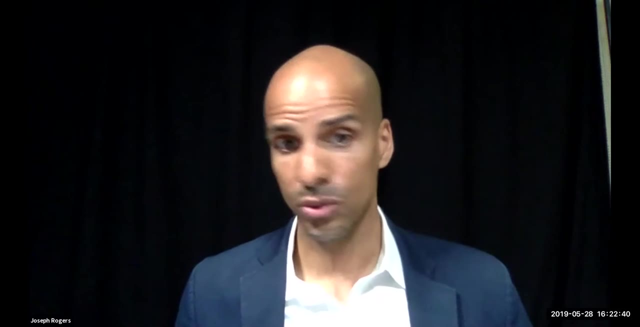 these opportunities than through the kinds of experiences that Prylite offers and that you've proposed to us today can be available to students at the school level, And we don't want to create any competitors for Prylite, I'm sure, but I know you would be happy knowing your. 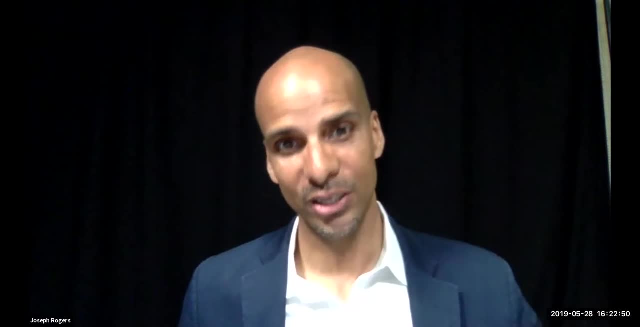 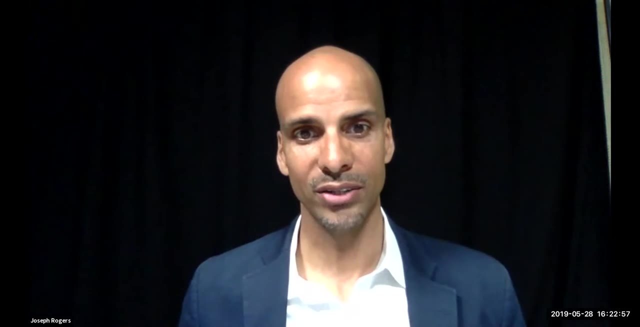 mission and your vision. You would be more than happy to see additional schools emulate some of the very rich and excellent practices and opportunities that you're providing there. So thank you again. It's so important that we have a nonprofit partner, someone who's partnering with. 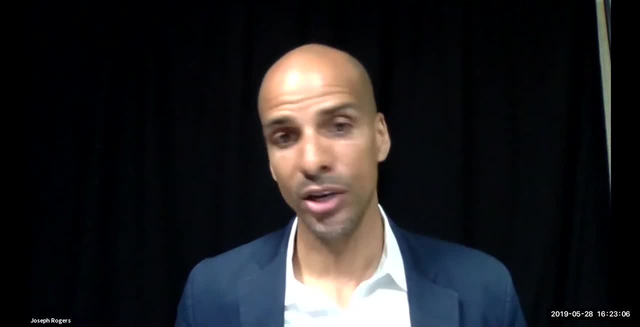 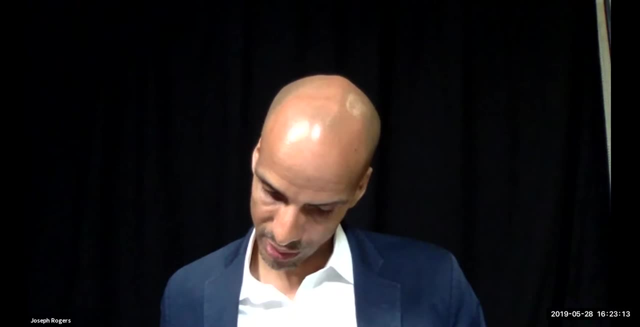 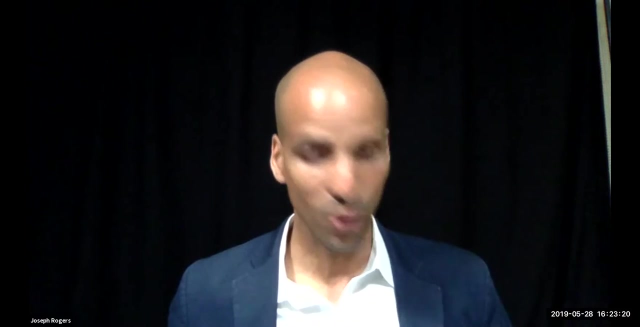 schools and providing opportunities. Thank you again, Diana. Certainly one other thing I want to mention here: let's see skills practice. Okay, good, We addressed that. So, again, please continue to comment, Please continue to add questions to Q&A, And we're going to, in just a few moments, get ready after we hear from our 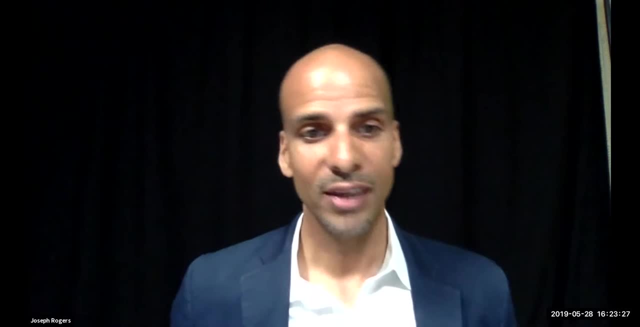 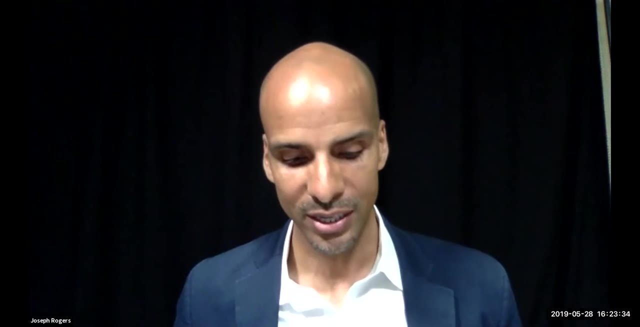 next future stakeholder. We're going to then turn to you- participants, public education stakeholders in New York and address some of your questions. And also I'm going to turn to you, Diana, and I'm going to turn to you, Diana, and I'm going to turn to you, Diana, and I'm going to 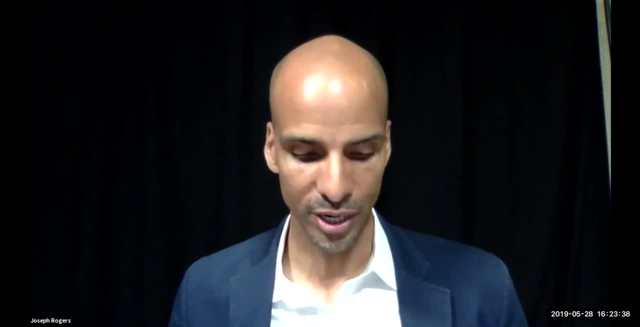 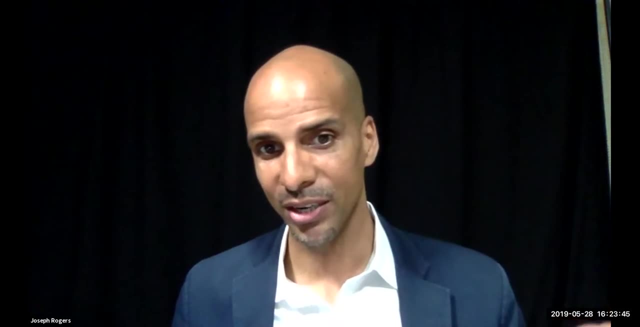 have a question for you that I'd love for you to respond to, if you would, in the chat box And, ultimately, in future conversations. This is, you know, we have a few folks here who are providing very rich insights, but we hope to, as the Democracy Ready New York Coalition, provide additional. 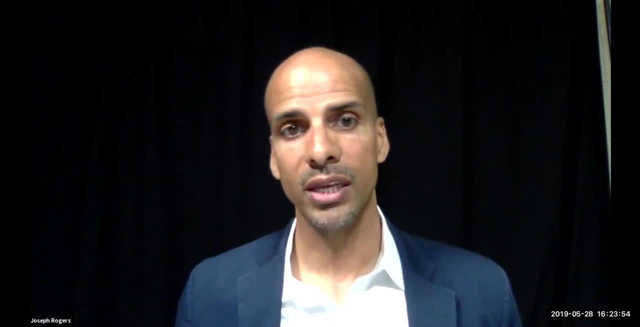 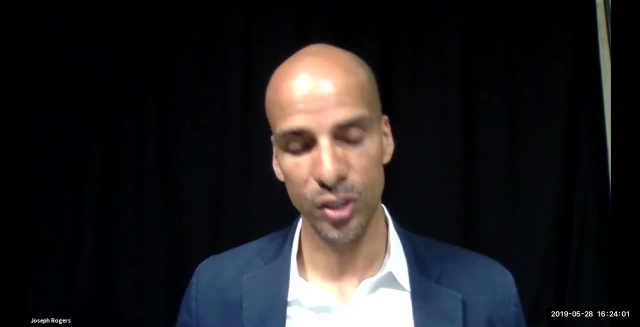 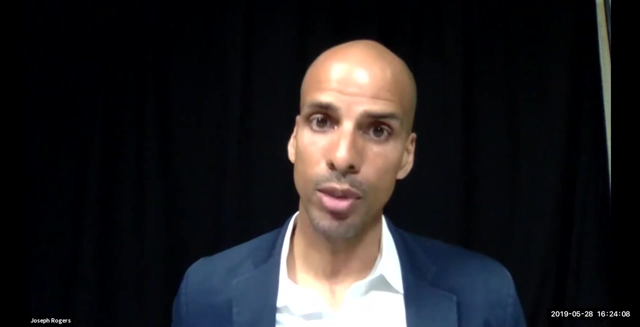 opportunities, including in-person opportunities, for key stakeholders like yourselves to engage in the conversation, to shape this work, to partner with us and, ultimately, to make sure that the conversation is being heard by everyone who has a vital stake in the civic preparation of our young. 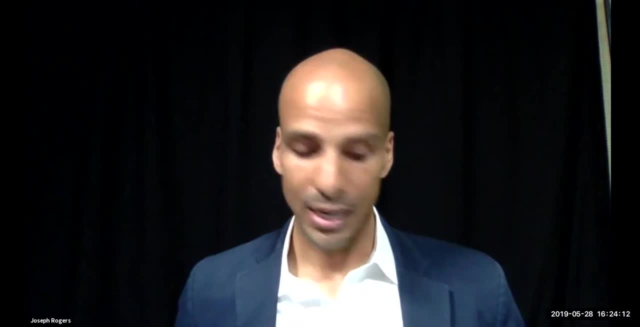 people, including young people themselves. So, with that said, I'd like to go ahead and turn to Jay Werona. Again, Jay is the Deputy Executive Director and General Counsel for New York's the New York State School Board Association- also a vitally important perspective. And, Jay, I'd like to ask. 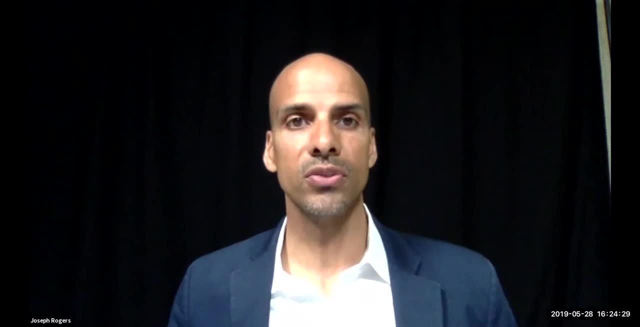 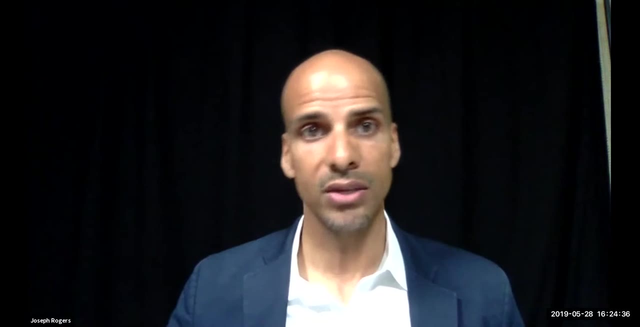 you schools that serve large numbers of students with extra educational needs, including those who may be struggling academically. what are some of the things that you would like to hear from them? Jay Werona is the Deputy Executive Director and General Counsel for New York's the New York State School Board Association- also a vitally important perspective. And, Jay, I'd like to ask you: schools that serve large numbers of students with extra educational needs, including those who may be struggling academically- and, as you know, in certain pockets of our state we have large 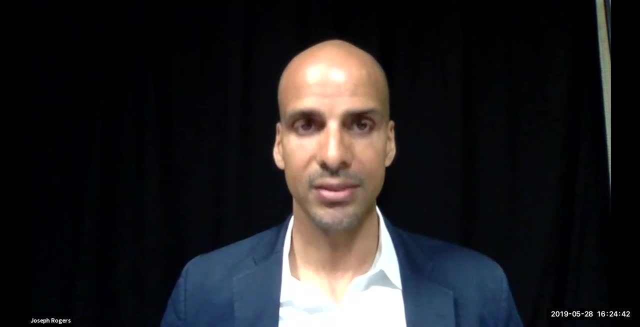 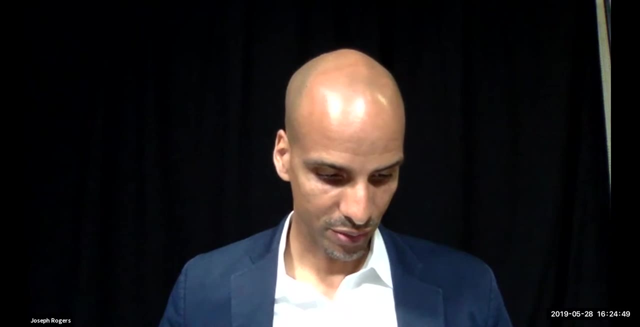 percentages of students who are having a hard time meeting state standards, not because they're incapable, but because they need more help. Many of the actually- I don't want to repeat the question, but you could answer that question as well- To provide those additional opportunities, Jay. 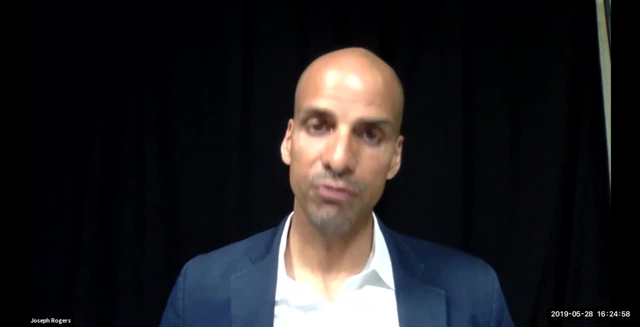 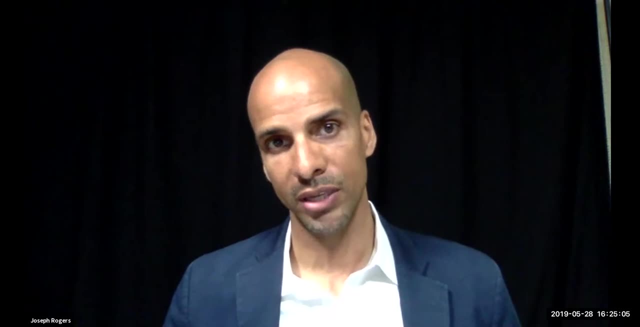 they have to provide fewer course offerings, They cut field trips, they cut extracurricular opportunities, et cetera, just to make sure that our young people, under their current accountability system and because young people should have the fundamental skills, 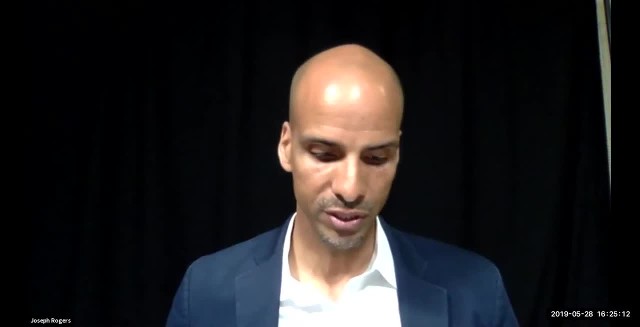 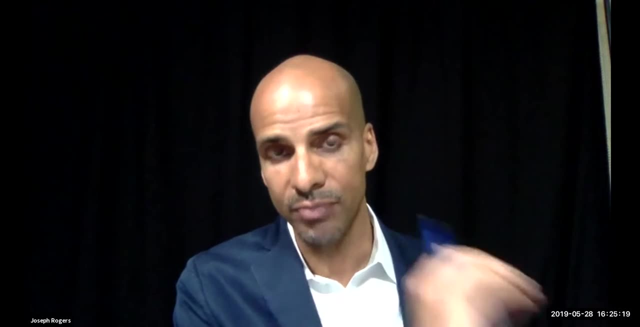 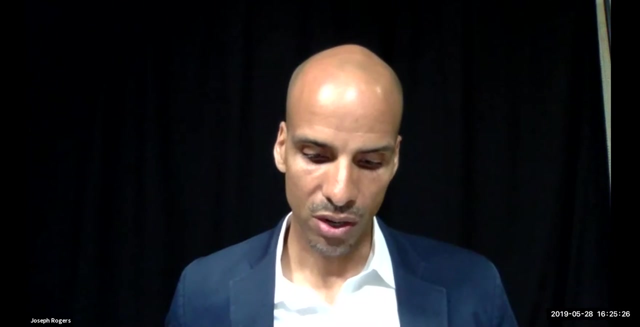 are able to meet basic state standards, to at least achieve proficiency. Are there ways to avoid some of these trade-offs between sort of the core, the basic curriculum, and just trying to scrape, you know, meet basic proficiency standards and these additional opportunities that we know are rich, that are hands-on, or is it simply inevitable that you? 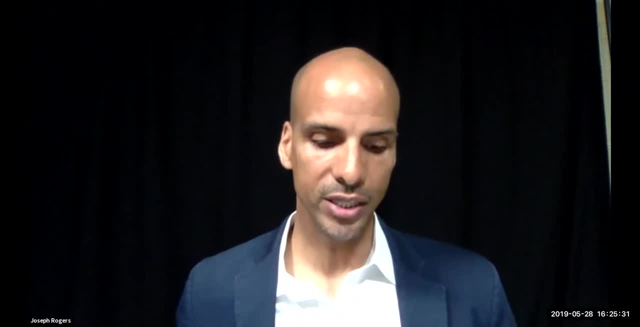 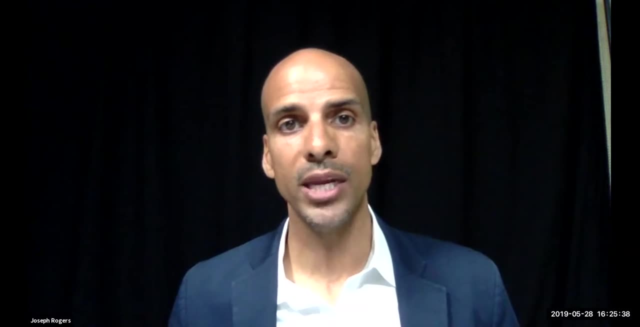 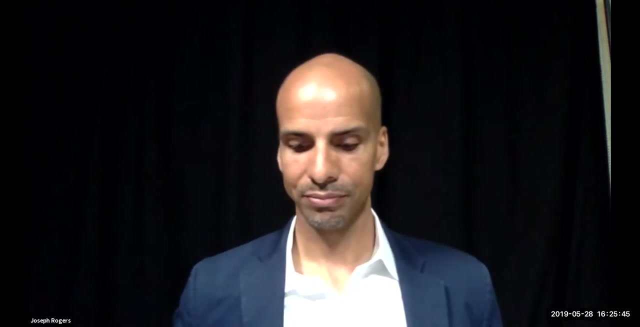 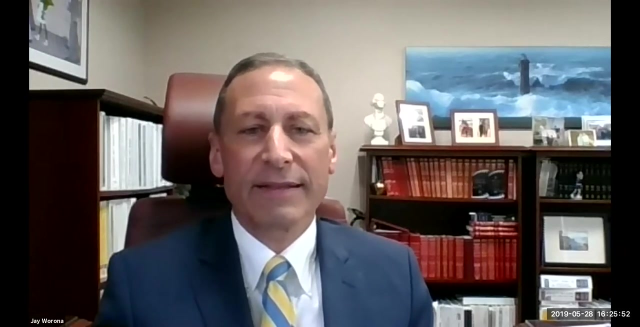 got to choose one or the other. If we agree that having a wide range of civic learning opportunities is good for all students, as the research suggests, how do we do that, leaving all the competing students with the same standards? So I would like to hope, on behalf of all the students of the state, that it is not inevitable. 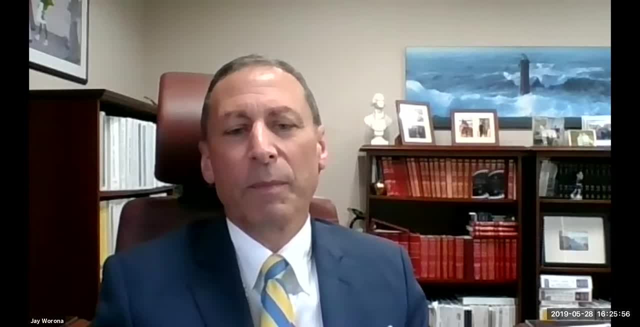 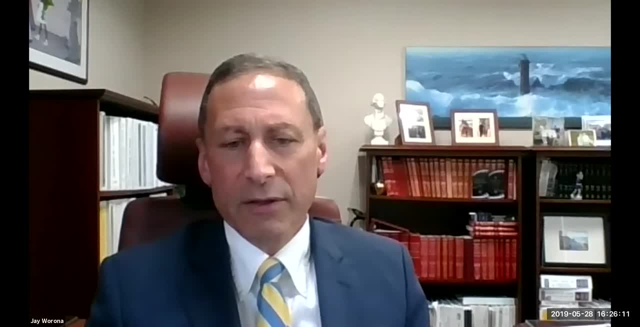 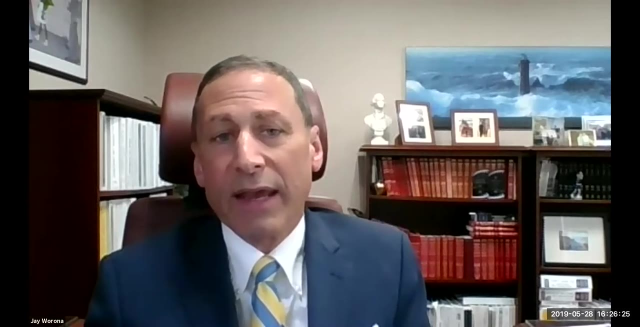 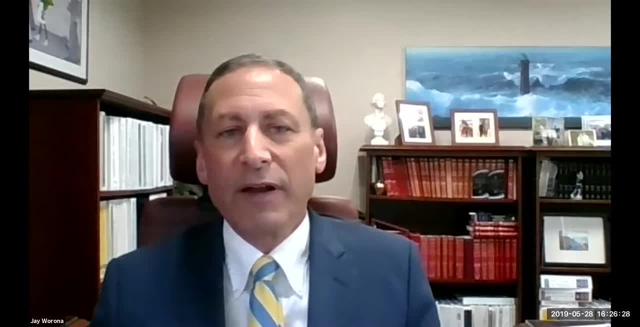 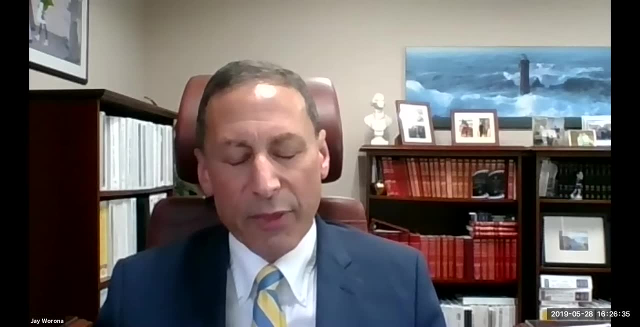 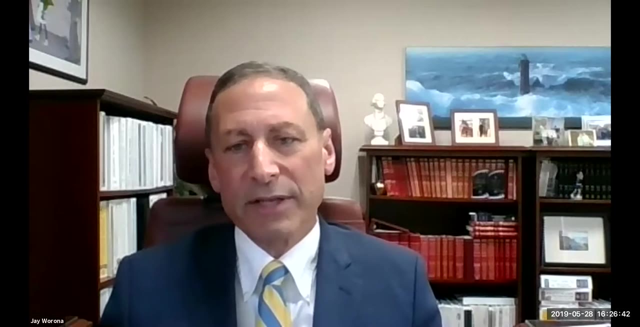 what we need to not accept is that funding is necessarily all we're going to get. I know that there are certain things that we can't control, like horrible recessions that are cyclical, but in funding public education, I'd like to say that I 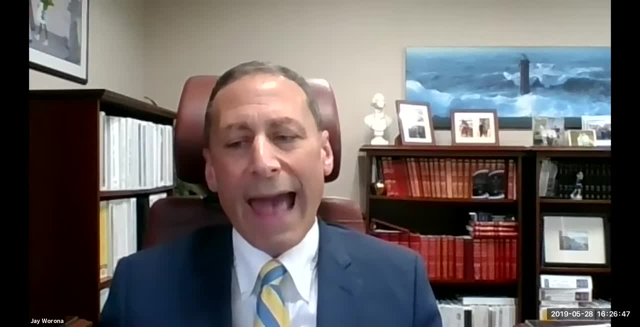 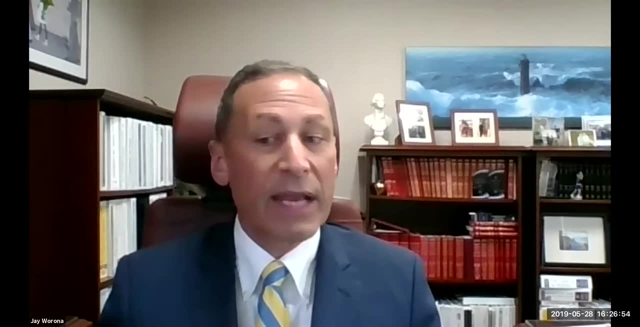 think the state needs to consider what resources it actually needs to ensure compliance with the state's educational priorities, particularly those that are constitutionally mandated In civics education. as you know, the Court of Appeals- our highest court in the state- said was: 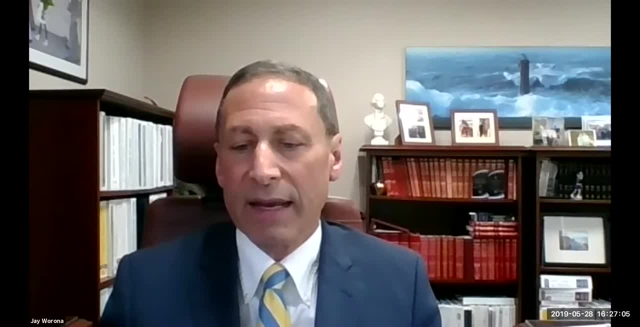 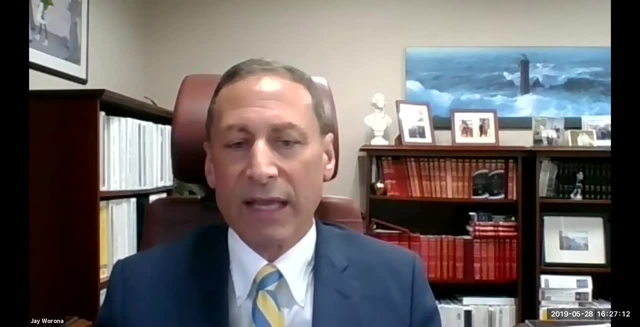 one of those things that was constitutionally mandated, And so, if this is a constitutional mandate, I don't think it is acceptable to say that we need to balance things to be able to take other things away that are necessary. So I would start the conversation by: 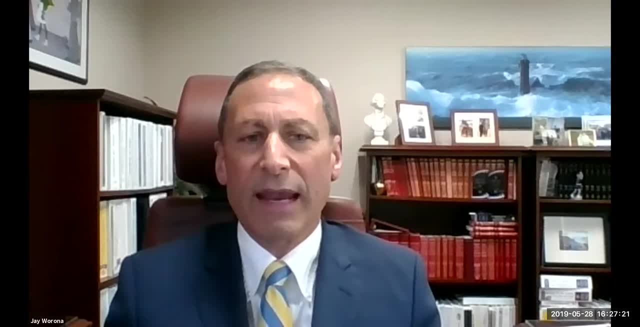 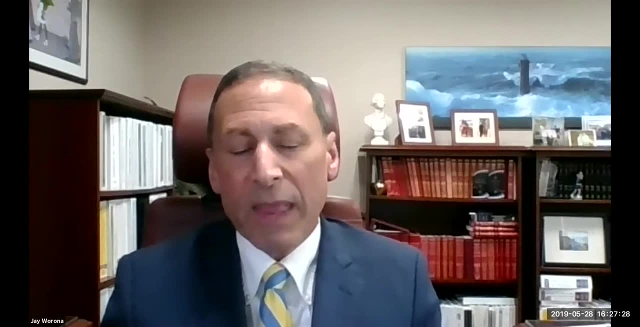 not accepting where we are right now. I think we need to keep the state moving in a direction to cost out public education, to place us in a position to see what it really does take, and they have to continue to do that on an ongoing basis so they don't dip into those periods of 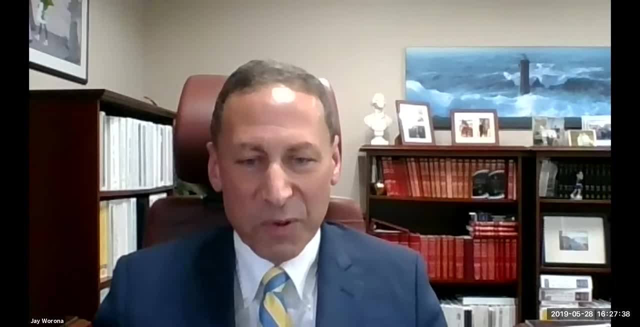 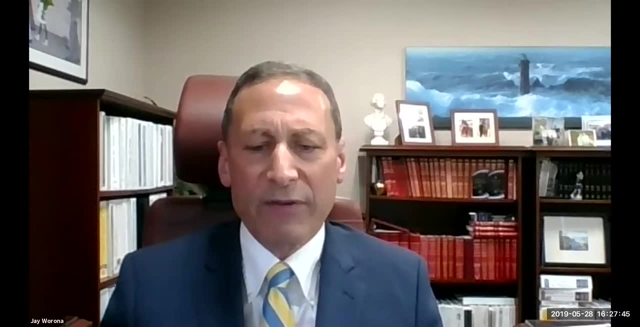 time where kids don't get what they need. Now, that's the, that's where I think, the aspiration where we want to go, but I think practically, I think we perhaps have to continue looking about embedding civics learning opportunities throughout the P through 12. 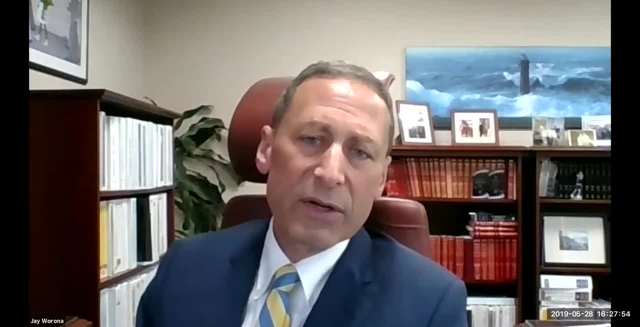 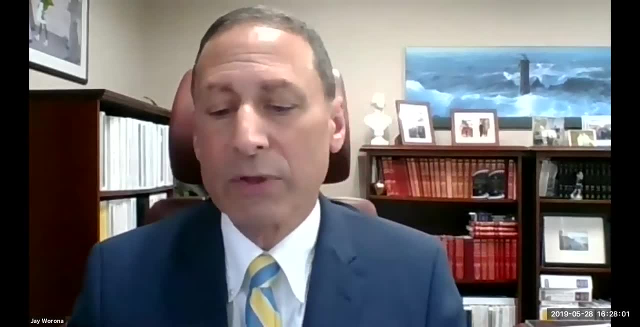 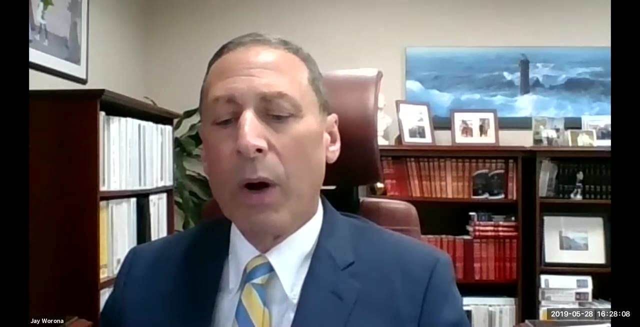 curriculum so that students acquire this necessary skill set throughout their entire educational opportunity with us. I think we need to consider mandating civics learning opportunities, but if this is going to be done, I think, practically speaking, the state needs to consider what can be. 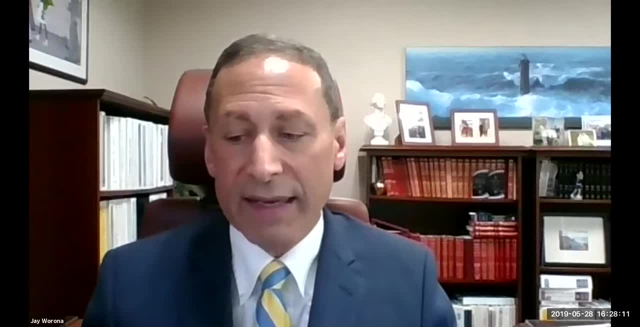 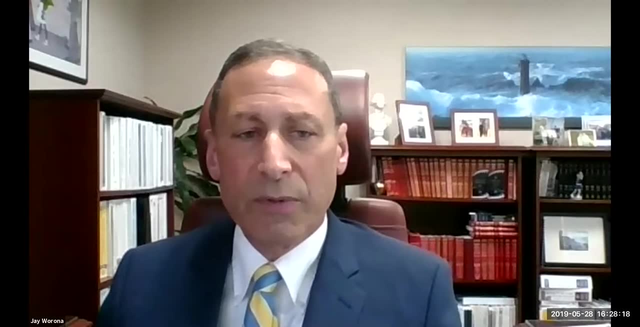 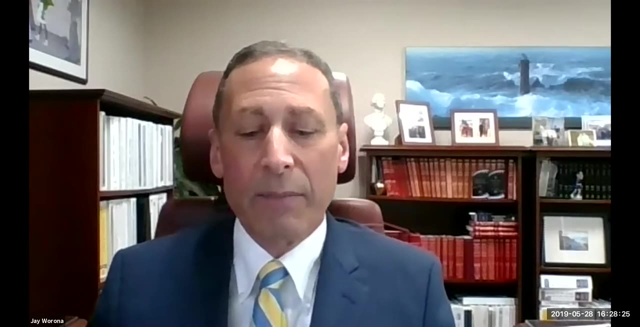 can be eliminated in our present curricular mandates that are either outdated or unnecessary. so we don't just keep another thing on top of what school districts need to provide, because then it's going to be all watered down and we're not going to provide them their opportunities. and finally, I think and I 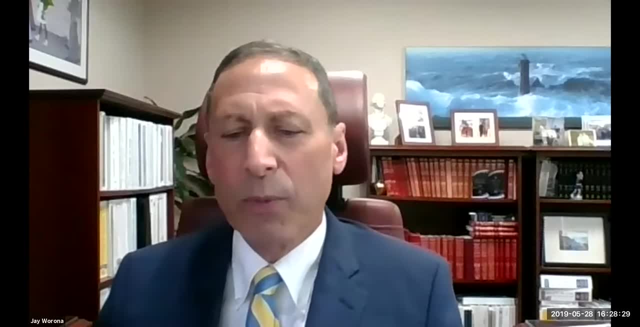 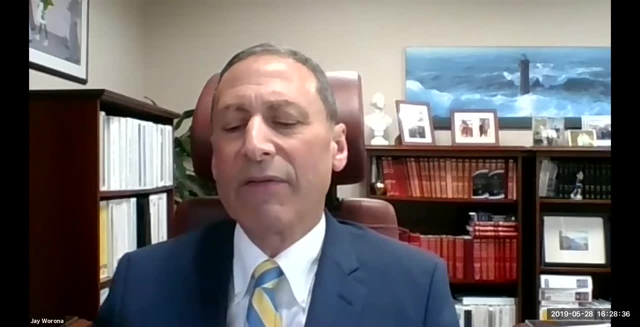 think Hamza said this beautifully and I think Tiffany made this point as well. other people have made this point throughout the discussion- and that that students need to have extracurricular activities and their opportunities for them enhanced, because these opportunities are truly the key to ensure that the important skill set of civics is actually becoming integral. 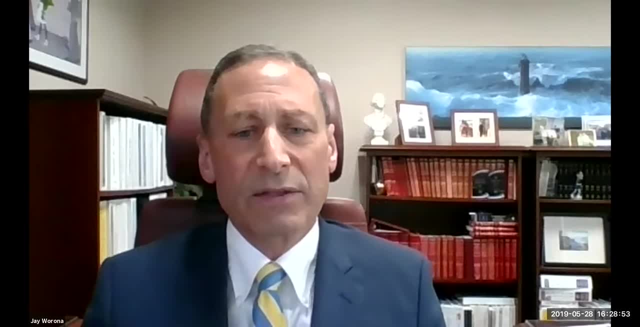 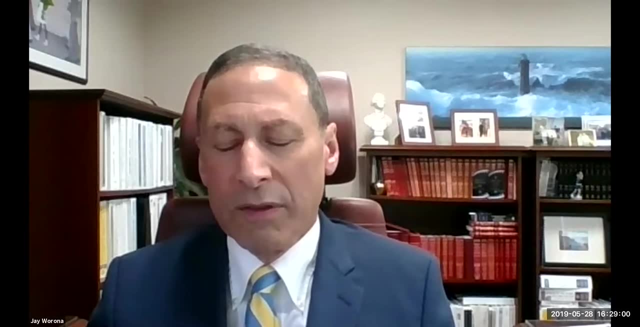 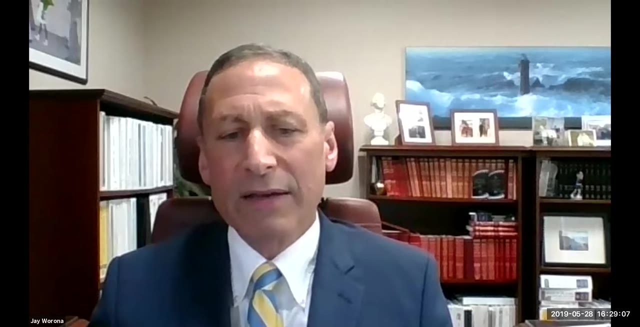 into the students educational opportunity. one of the things that I think is very sad and- and I think it was Tiffany who said this- that that you know these are important opportunities but many, many kids and many, many school districts throughout the state don't have the opportunity. I'm active in the New York State Bar Association. I know that the 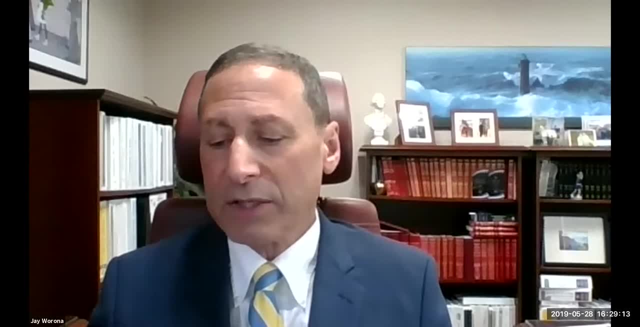 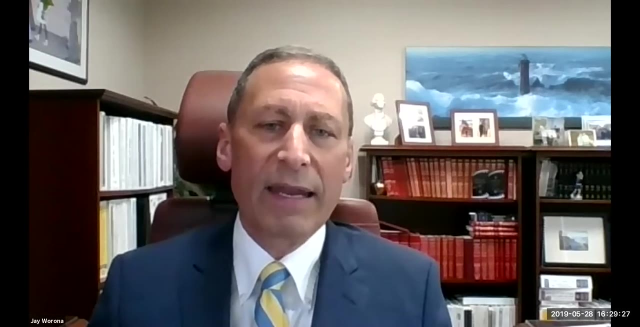 Law, Youth and Citizenship Committee that I am on sponsors the moot court competition. they just had their statewide competition this past week and I and I watched some students from Long Island win that competition and all I could think about was how absolutely sad that it is sad it is that kids 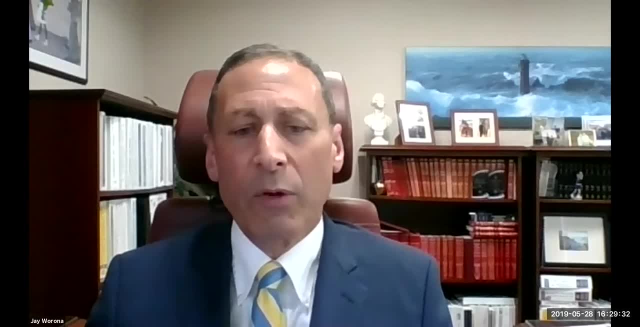 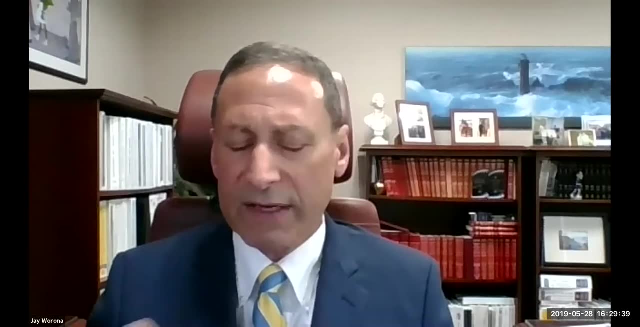 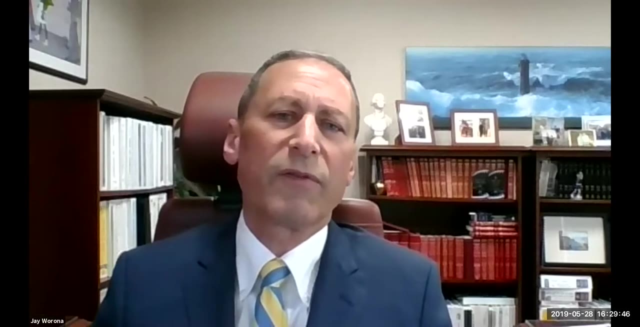 throughout the state don't have those opportunities. the We, the People program has another wonderful opportunity to get kids totally engaged in understanding our civics opportunity. you know civics and and in our democratic system and far too schools- too many too few schools, excuse me- are involved in that exercise. 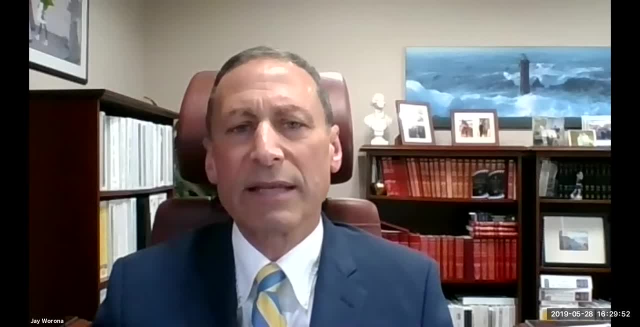 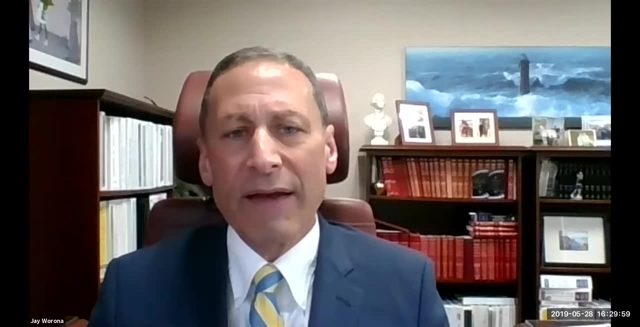 and I understand why, but I do see that when kids are engaged in these activities- unlike what they're learning in their textbooks- they're actively engaged. these are, these are learning opportunities. they were never going to forget and it is. it is very sad to watch how many of these kids are and how proficient they become, and to see that 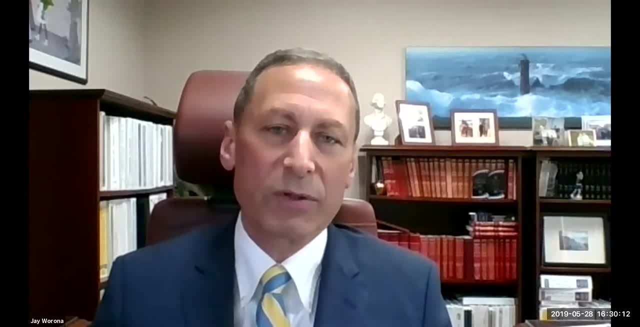 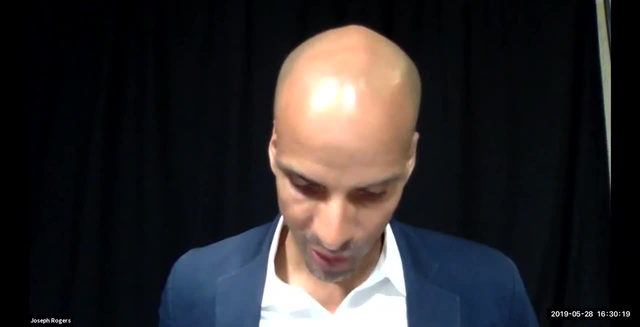 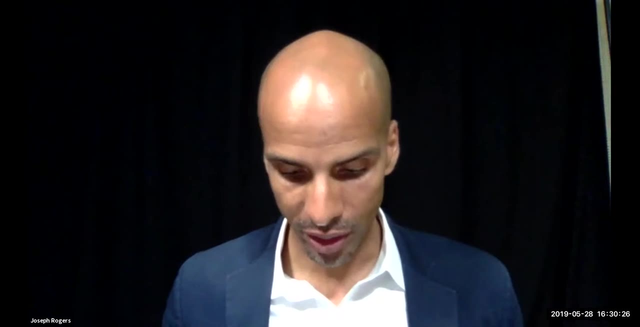 so few of the students in our state actually have these opportunities. it's just unconscionable. great Thank You, Jay. a couple important things I want to know here from your remarks, and then we're gonna switch over to our engagement with our, with our public stakeholders out there. you said you know this is a 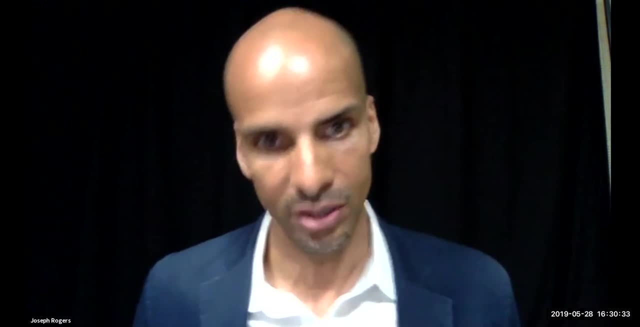 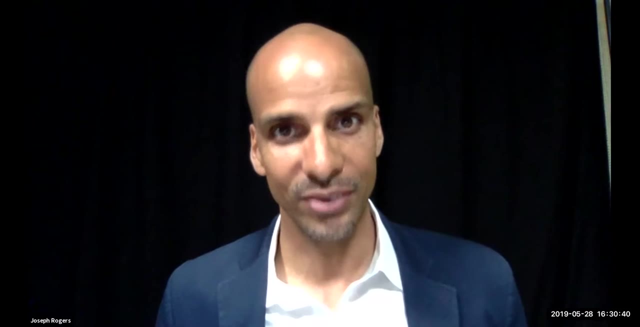 constitutional obligation, this is a constitutional right, this is the law I and a constitutional right doesn't dissipate in a recession. it doesn't dissipate, doesn't go away right conveniently when we're going through financial hardship. and I think you suggested that the education of our 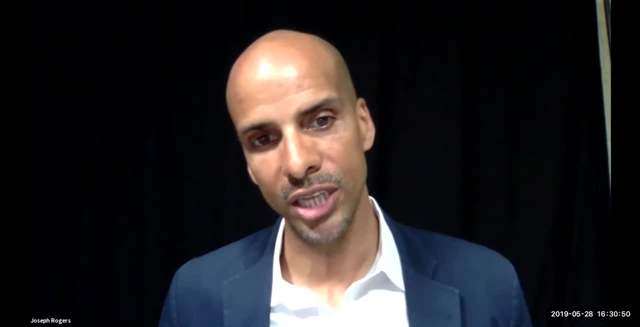 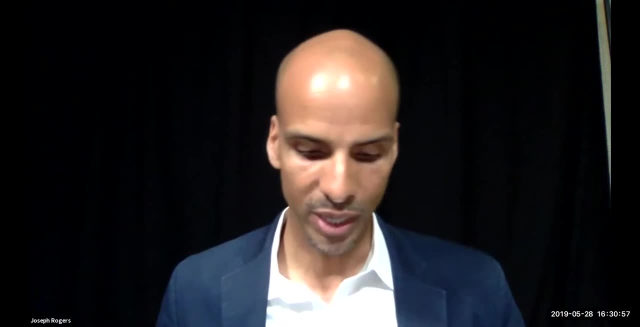 young people. the education of our children and making sure they're ready to shape and participate in our democracy is fundamental right. we shouldn't have to, we shouldn't, there shouldn't be any trade-offs in that endeavor. we need to uphold that and to fulfill our obligation. you also mentioned: 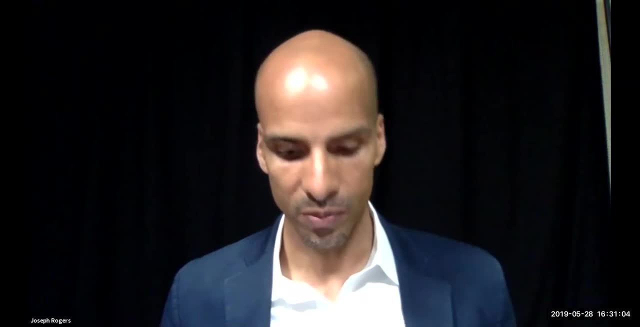 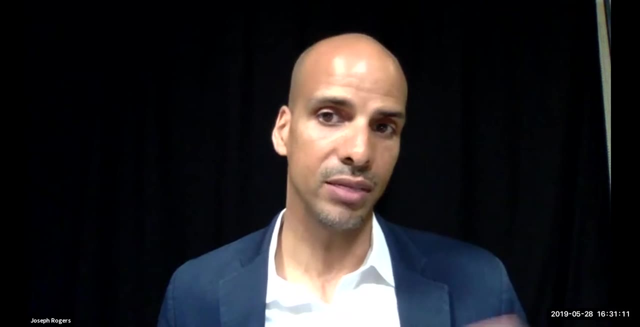 that we need to. we need to solve the problems that we're in and we need to state to figure out which resources are currently available in schools. Where are we? How close are we? And you know this is about. this conversation is about equity and some of the disparities that 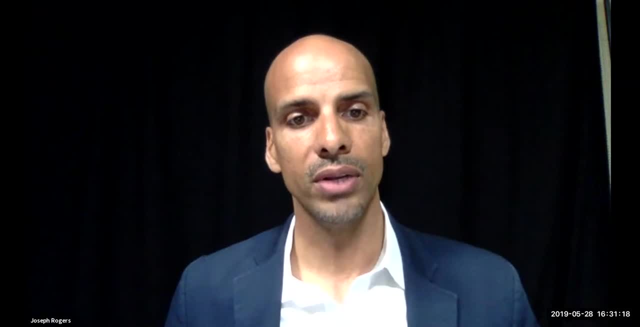 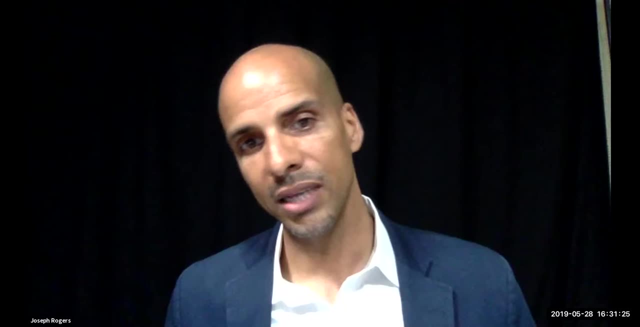 we noted in our research, and that some of you other folks out in the, among other stakeholders, are aware of, is that not all schools are able to provide this opportunity. So how can the state, our state elected officials, how can our policymakers, assess where we are? and then, 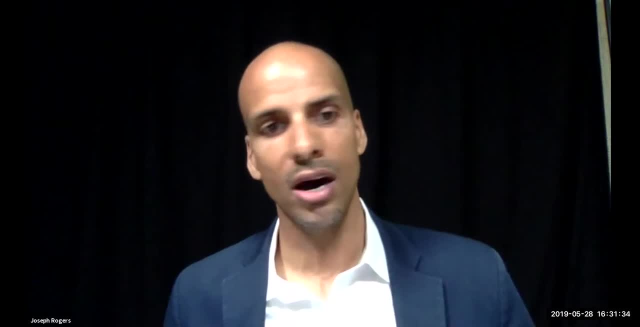 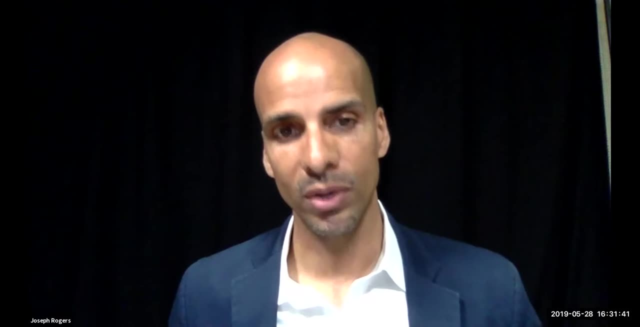 pinpoint and, as you said, I think, cost out right. How much does it cost to provide these opportunities to all young people in all schools at the appropriate level, at the adequate level to make sure they're truly ready by the time they graduate? But it doesn't start in high school. 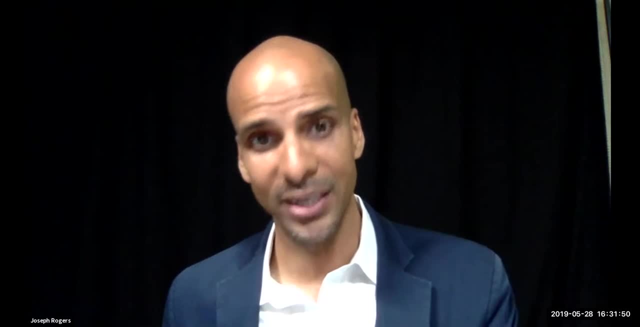 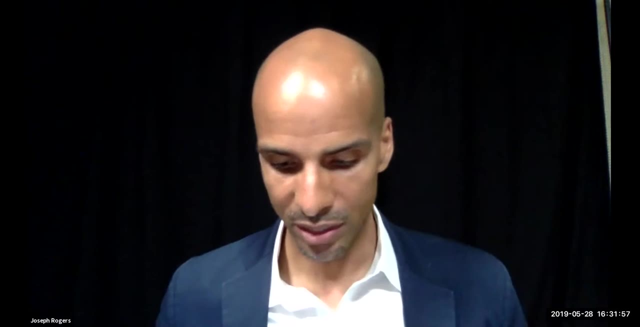 as you suggest, doesn't start when you're about to finish secondary education. It starts much earlier than that. So we need to figure out what are those essential opportunities along the way. We at the Center for Educational Equity have outlined some of them in our report, which you 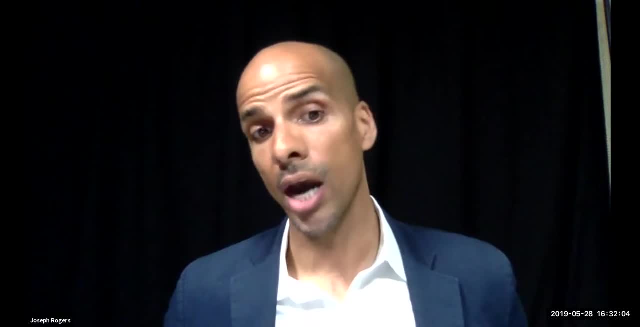 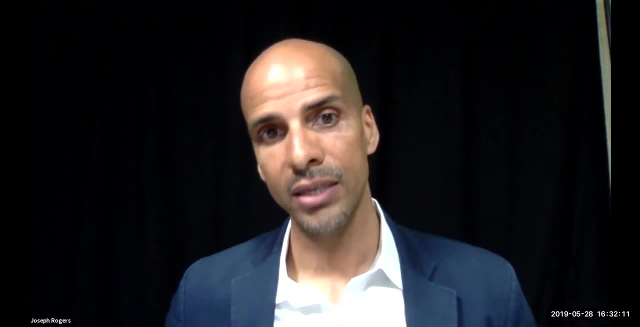 all will receive, But the state really has a responsibility and an opportunity and really an interest and a vision for doing that. I believe based on their commitment through that College Career and Civic Readiness Index and the Civic Readiness Task Force that they created to explore these, 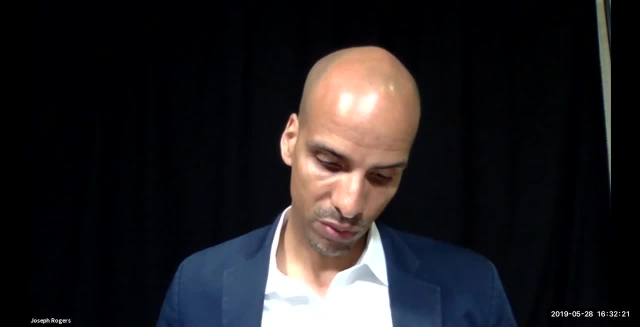 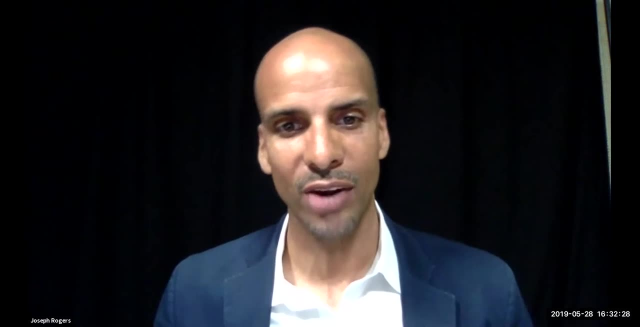 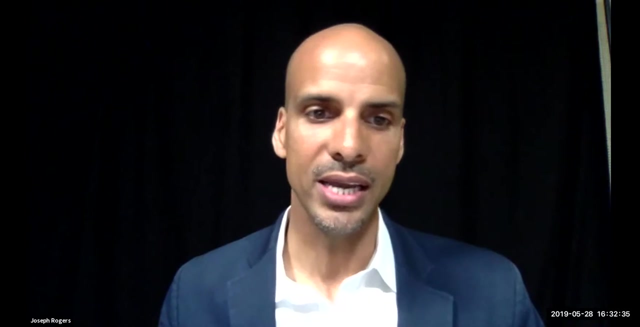 and related issues. So thank you, Jay. so much for your contributions, And so, with that, thank you everyone for your patience. I hope that this background information has been useful to you. I do, So I'm going to turn to you. Looks like we have a really good group here today. I'd love to hear a 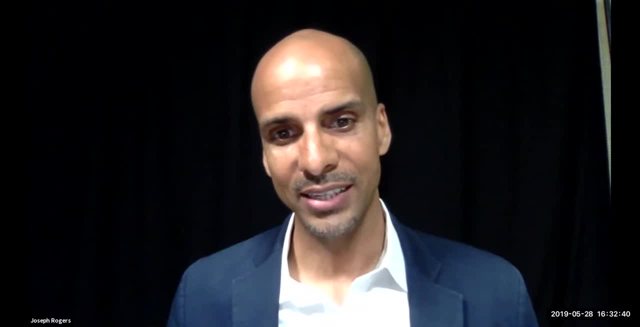 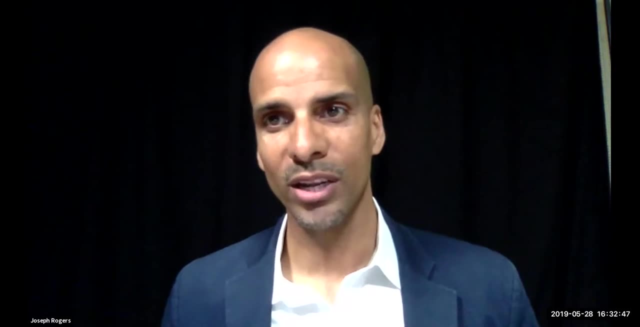 little bit about or actually see where you're from, And I didn't trigger this poll. You know we have these snap polls that we can do through this webinar platform, So I'd like to go ahead and quickly trigger, before we get to your questions, at least one of these polls here to. 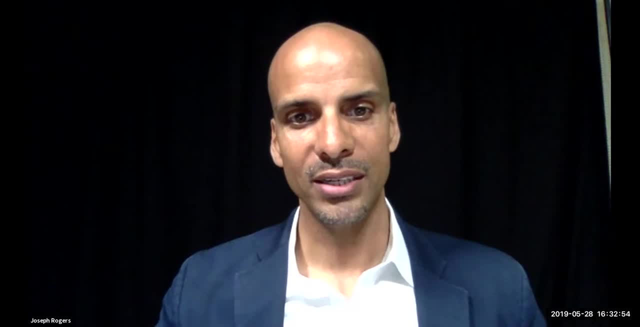 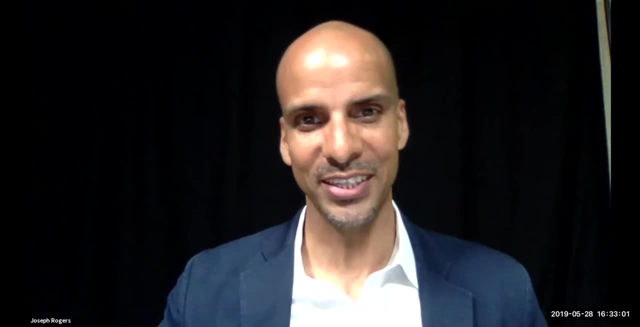 find out who's currently participating in the webinar, to better understand where you're coming from and which perspectives you share. So let's see if I can do this correctly and efficiently. I'm going to go ahead and launch this first poll, And the poll says which of the following stakeholder: 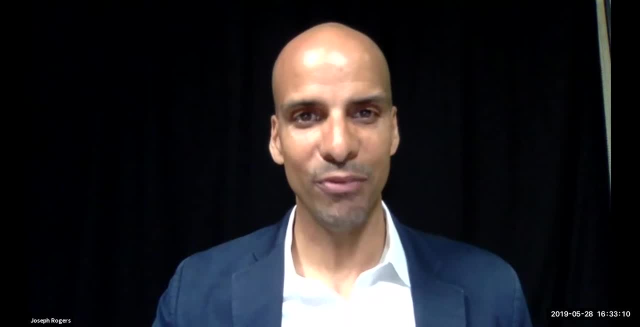 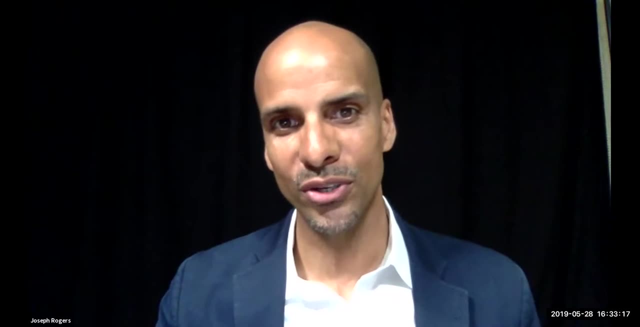 groups do you most identify with? And I know this is going to be difficult for some of you, because you're a student and a teacher, You're a parent and a school administrator, what have you? But if you could choose the one that you most identify with, just for today's conversation? So I'm going 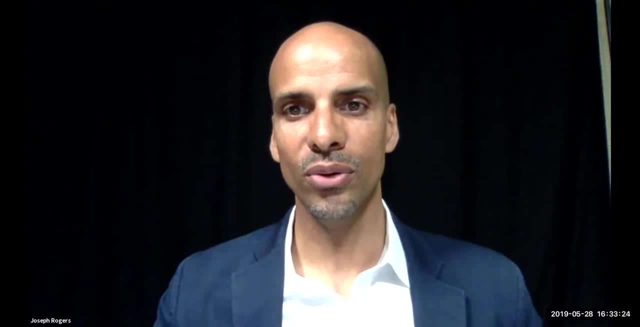 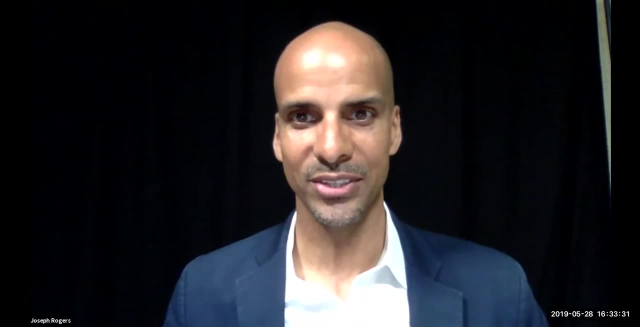 to launch that poll and then give you a few seconds to. if you would, you should see a field pop up. I see, Okay, great, The responses are coming in already. You all, you all, are going to be. it looks like you've done this before. Wow, this is exciting. All right, So let's see where. 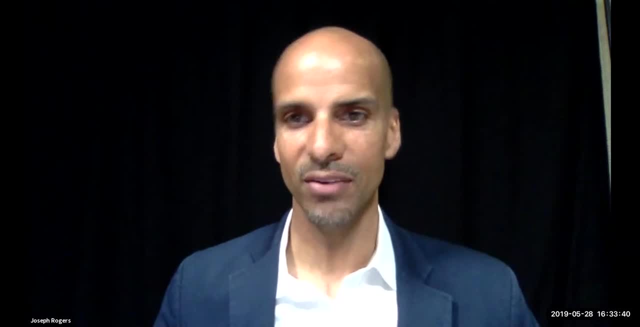 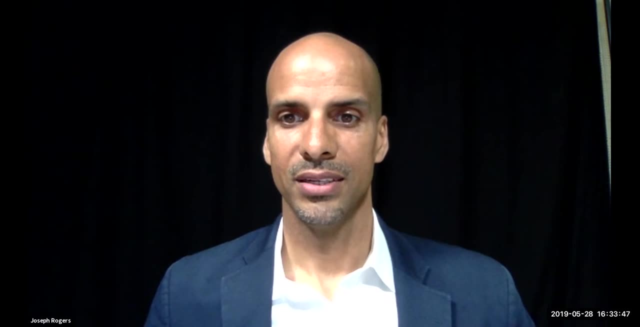 which groups you most identify with for the purposes of today's conversation? Okay, It looks like. okay, I'll give you a few more seconds here for you all to maybe to chime in here. It looks like I mean, one of the things I'm noticing here is: you know several of our featured stakeholders. 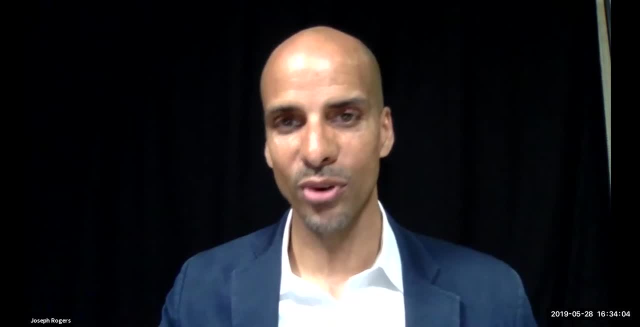 need to be at the table, need to be involved in these decision-making. Of course, Hamsa is here, but it would be great to see more young people involved in this particular conversation, And I think what we may need to do is have probably a youth-specific webinar. We'll invite other. 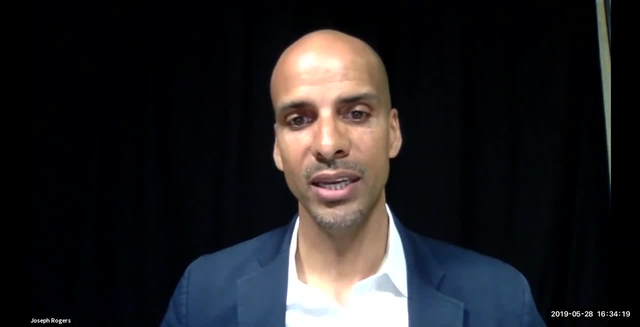 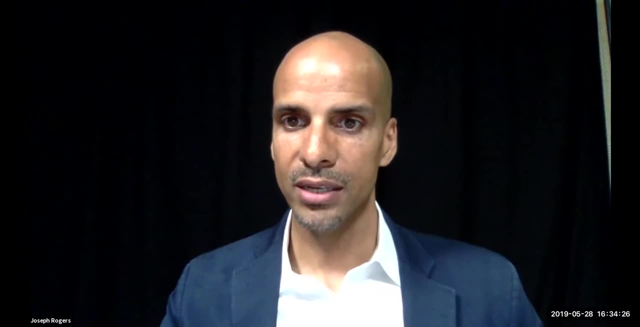 stakeholders, but really have one that's centered on youth involvement in this policy-related, research-related equity work. So it looks like we have a lot of nonprofit folks here. Not everyone has had a chance to vote, That's okay, But of those who did vote, 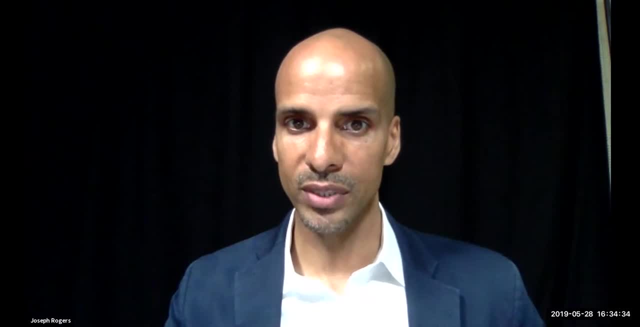 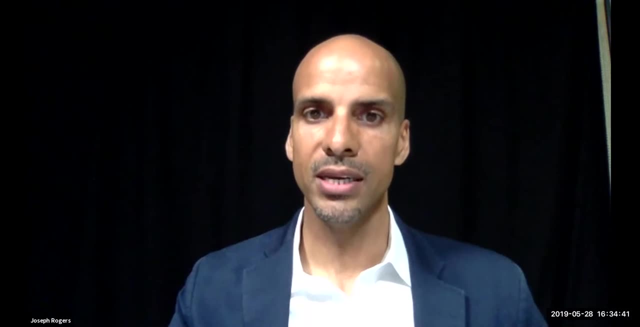 a lot of nonprofit people. We also have a few teachers, a few educators, a couple of parents, some college faculty members and otherwise a couple of school board members I see. So thank you all. I mean this is helpful for us as we look to plan additional opportunities. 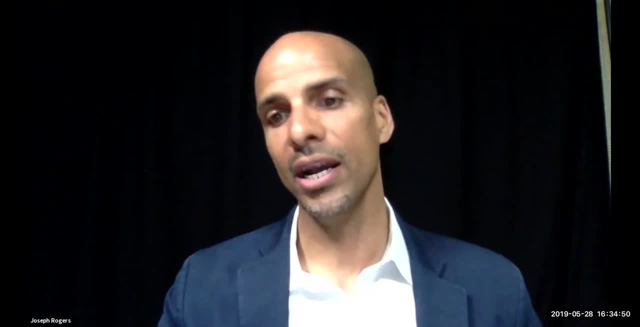 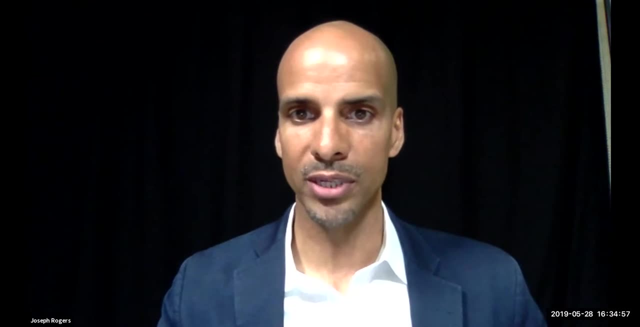 and figure out how we can best target and tailor the webinars and other opportunities to different stakeholders. So it looks like we have some work to do there. but thank you all for participating. So let me go ahead and close that poll out here, And then one. 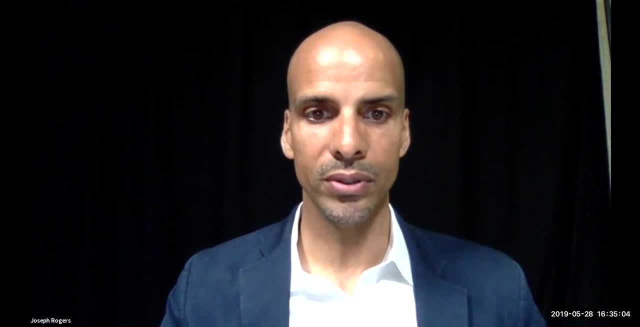 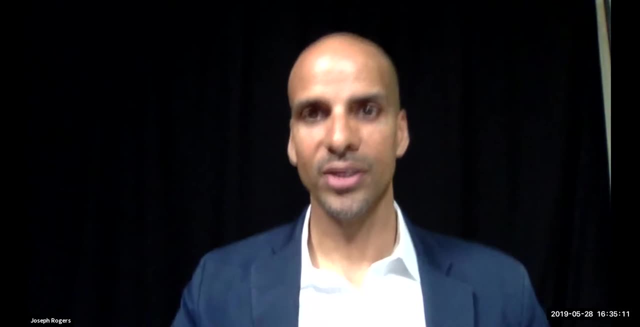 one more poll before we turn to your questions here. Let's see we'll end that poll. Let's see if we can do this. results: How do we launch the next poll? We're going to go here to the carrot and then we're going to select this. Okay, Everyone's learning here today And that. 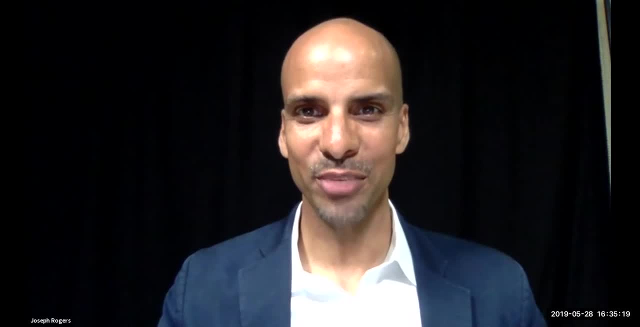 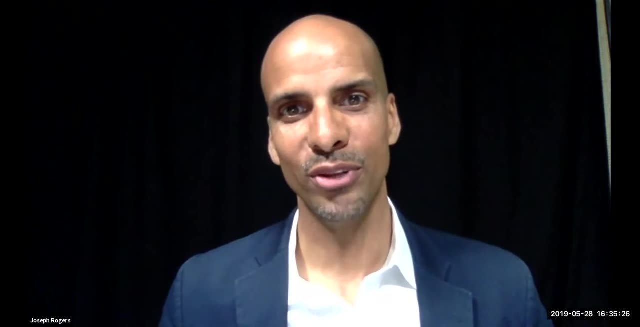 actually is a good segue to our next question, which you should be able to see now. in a moment, Let's see. You should see it now. How familiar were you speaking of learning with New York students' constitutional right to civic preparation before this conversation? 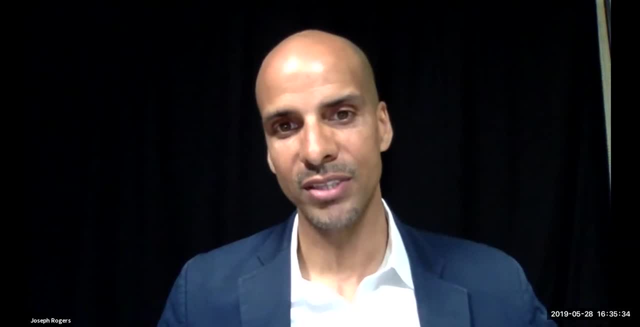 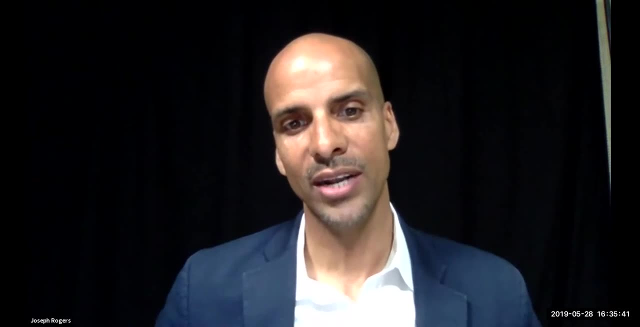 All right, We talked about a little bit at the very beginning of the conversation. You've heard some of our stakeholders today here refer to the lawsuit, the constitutional right and what it guarantees in terms of civic preparation. Let's see where you're coming from and what level of 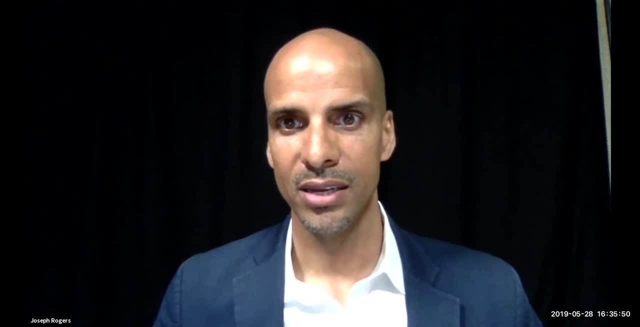 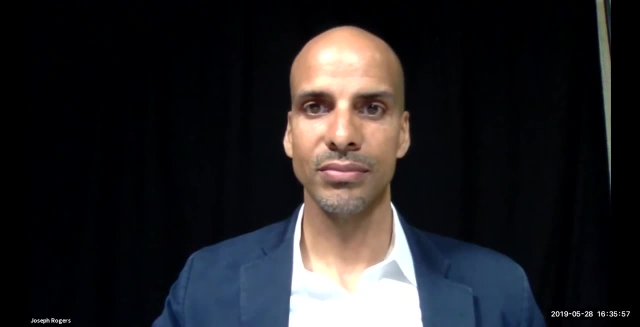 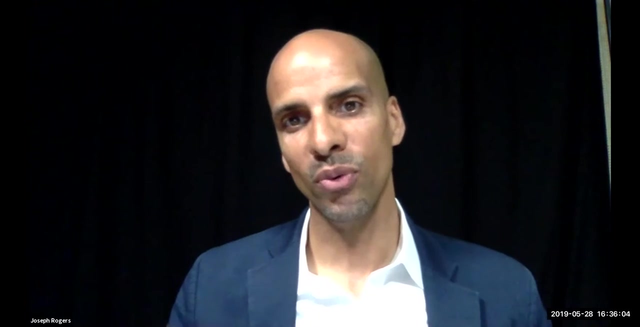 understanding you may have had before you joined us here today. So we still have a couple more seconds here, People who haven't had a chance to weigh in. Okay, Let's give you about five more seconds Again. how familiar were you with this constitutional right that all New York? 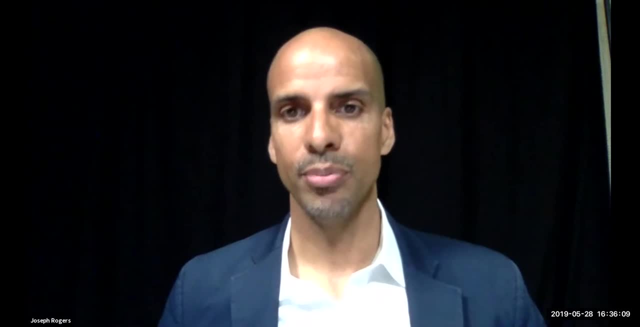 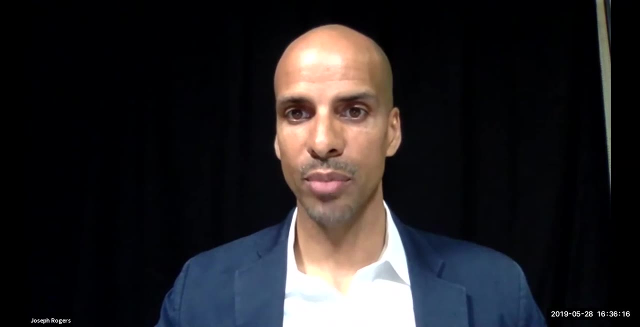 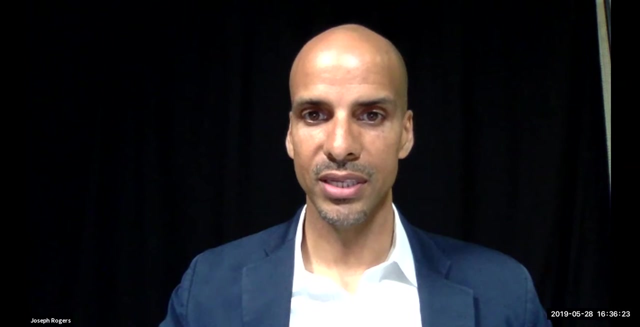 students have to be prepared for civic participation before this conversation. All right, So let's go ahead. I'm going to end the poll now. It looks like we have, and I'm going to- let's see. I'll share it with you so you can see. I think I could share it if. 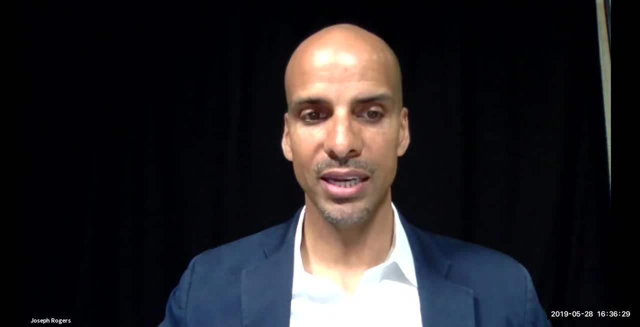 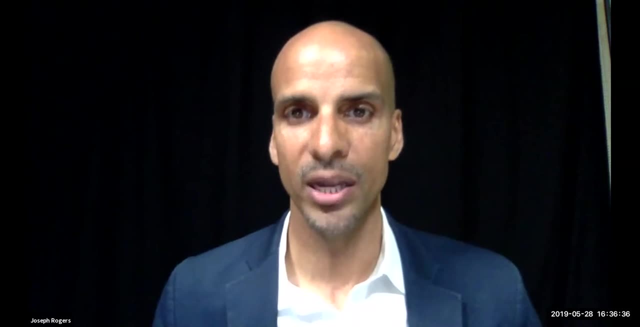 we share results here. You should be able to see Again not everyone who's on. looks like we have close to 60 people who are participating in the webinar, but of the folks who did participate in the poll you can see there's a decent spread there, But a large. 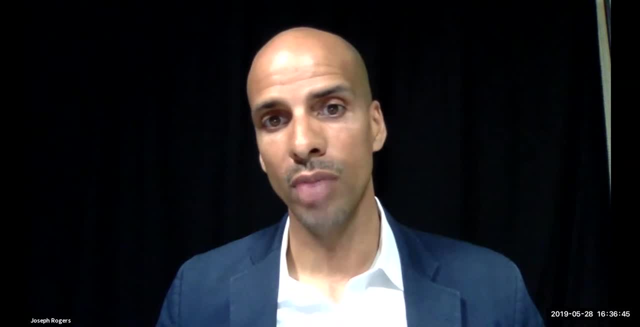 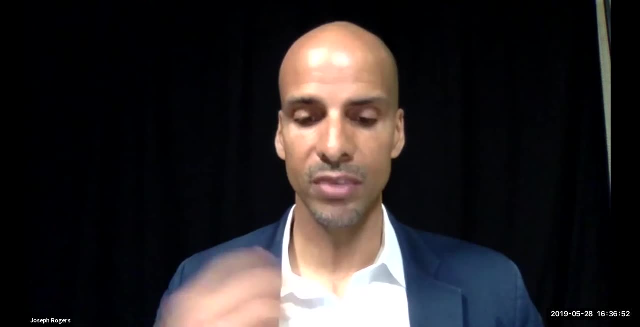 well, yeah, a large majority of you either didn't know much about the right or you hadn't heard of the right. It's brand new to you. So that's good, And that's why we're providing this conversation as the Democracy Ready New York Coalition: to raise awareness per our mission and to engage. 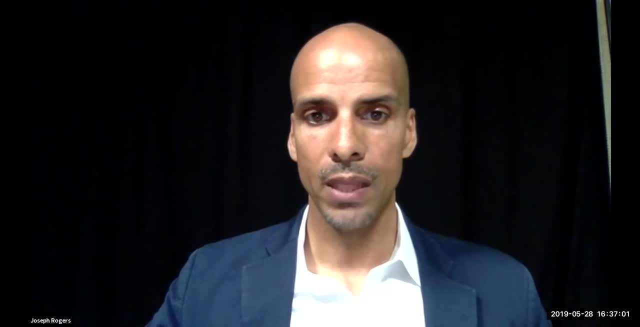 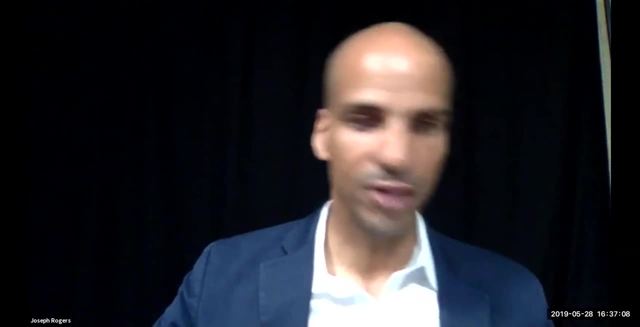 additional stakeholders. So let me stop that there, Okay, And we will close that poll out. So thank you for participating. Okay, So we do have a few minutes left. Why don't we go ahead and turn to the questions here? I'm going to turn to the Q&A. 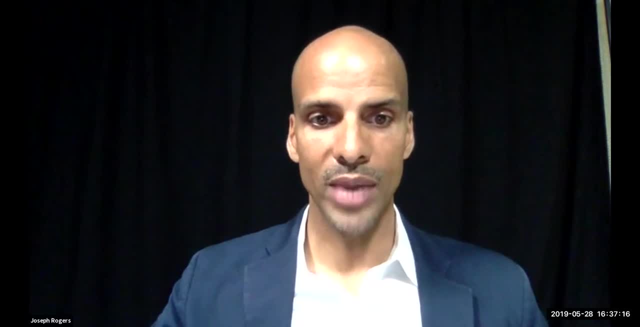 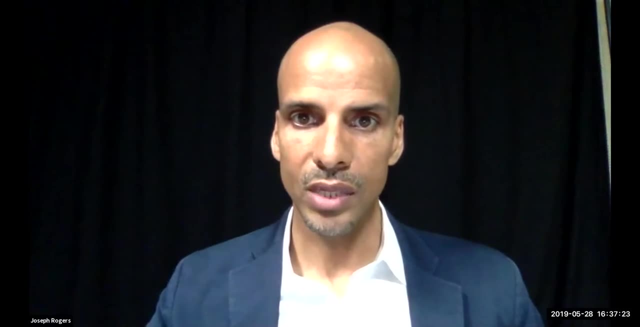 box here and see what we have here. Again, we're not going to be able to- I apologize- get to all of the questions, but let's see what we have here. All right, Let me move this up, All right. 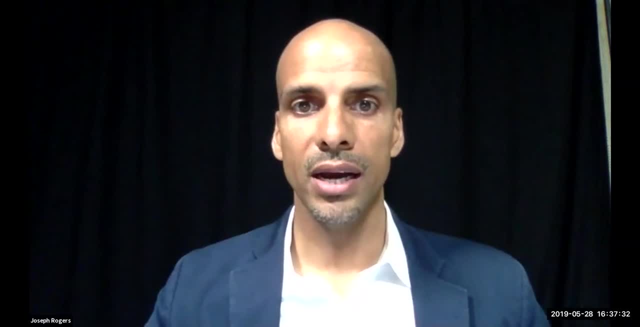 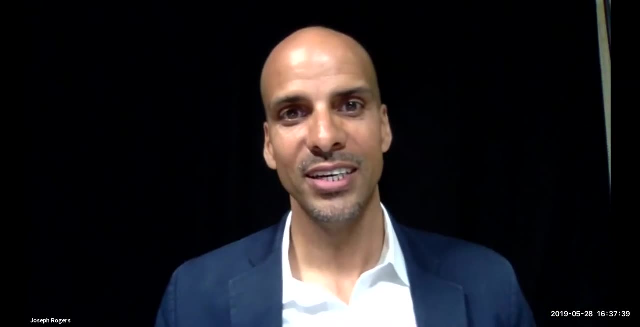 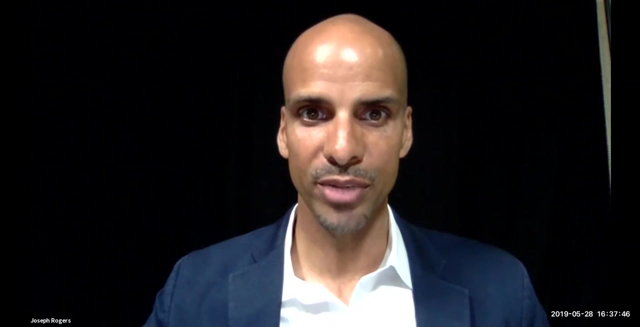 So it looks like Claire again. Claire is the other technical support person from the Office of Instructional Support here at Teachers College And she's also teaming up with Cassidy to field some of your questions. make sure we see them here. I see one here near the beginning: Claire documented. How do we best respond? 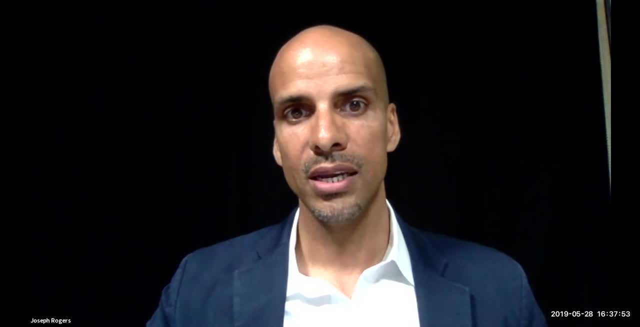 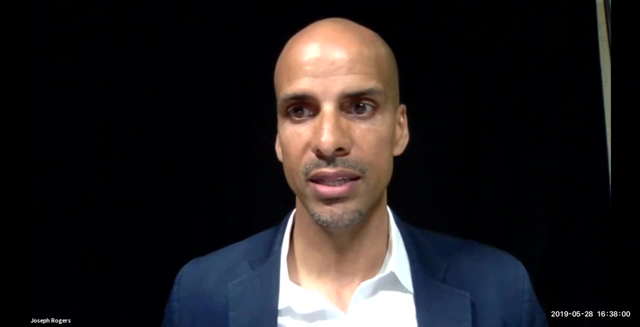 and support schools and educators, And I guess I'm going to paraphrase that a little bit. Hopefully I get to the heart of the question that I believe someone had posed in the chat box and we transferred over. So I want to target this specifically to maybe Tiffany, for example, but really any of our student panelists and anyone here is qualified and equipped to answer this question. 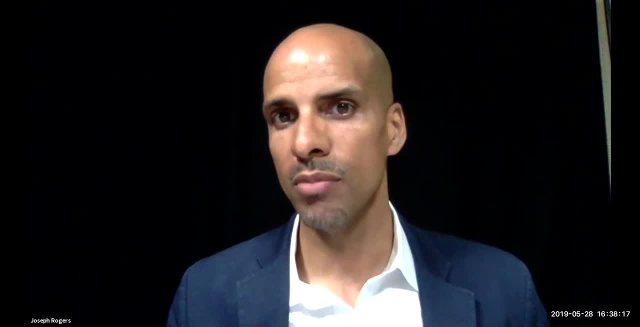 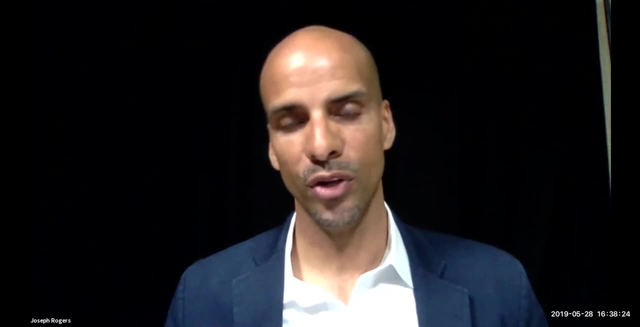 What do you need? Let me simplify this. We've heard some of some elements that you think are essential, some of the things that need to be available. What do you think we can do? And I'll let, if I can frame that a little bit: what can sort of the state do? and then, what can? 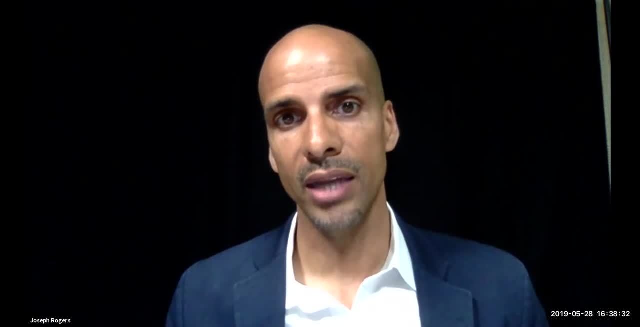 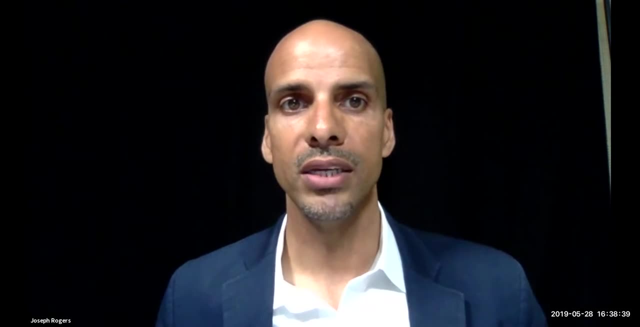 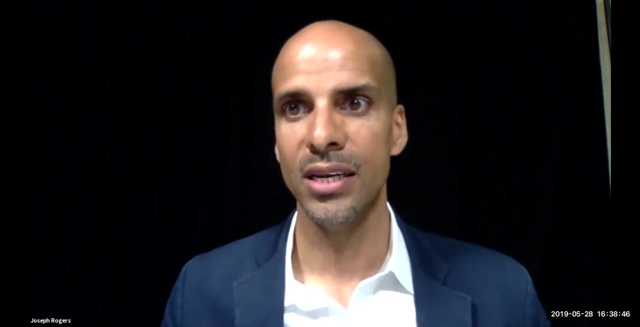 the Democracy Ready New York Coalition, do To make sure that schools and educators are supported to provide the civic readiness opportunities to our young people. Is there anything else- Again, we have touched on that, I know. Is there anything else that, because we've gone through the entire range of stakeholders that maybe you were in the beginning- that you'd like to comment on in terms of how we can best? 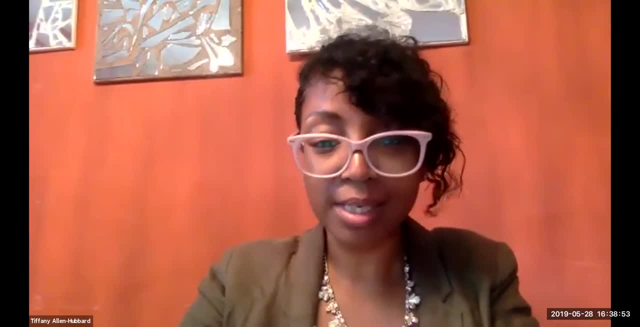 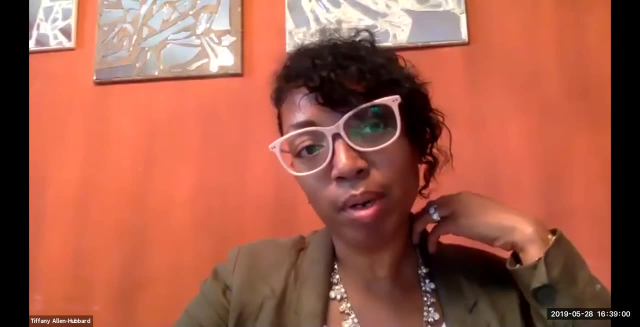 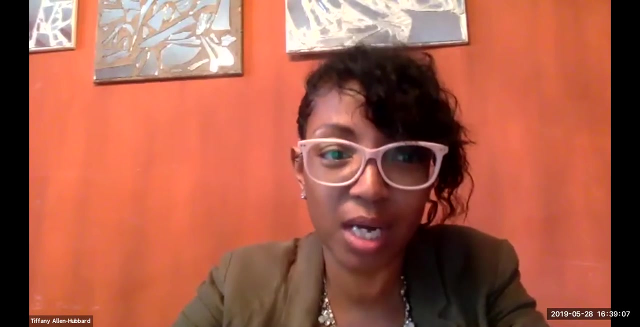 support schools and educators, Tiffany. So I've been in the chats and looking at the questions and kind of like seeing what the conversation is, And I am a member of the UFT AFT civics working group. So we're in the midst right now of like 50 educators all the way from K to 12. We have many elementary school educators, many. 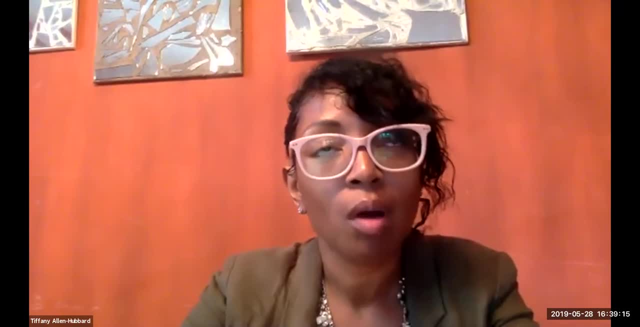 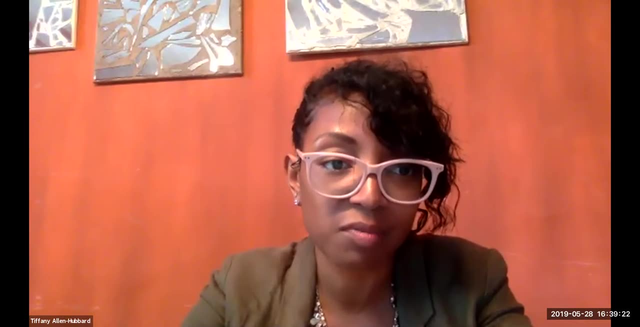 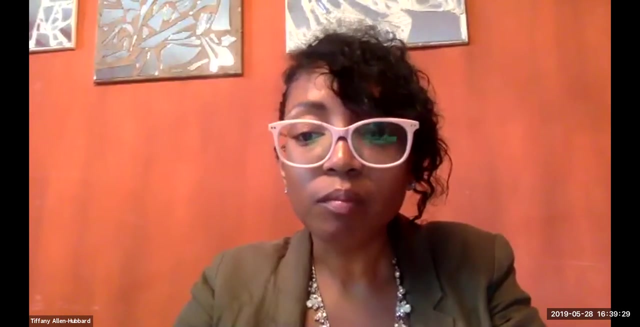 middle school educators talking about what civics looks like. So the idea here is that civics is not only something that is translatable to the social studies classroom, but to every classroom and outside of the classroom in all schools. A couple of things that I think are really important to me. 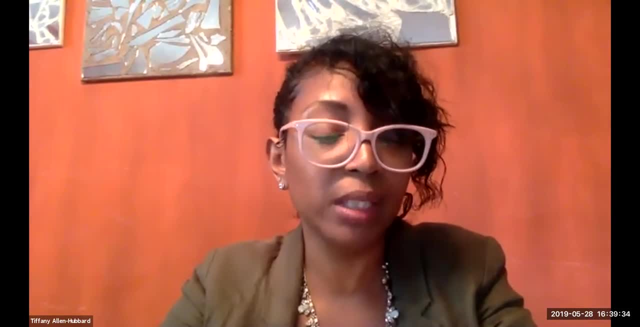 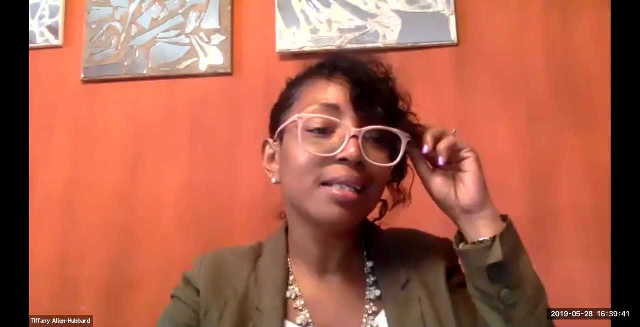 I think that we can really do to support schools, regardless as to the school's budget, is, of course, to have partnership with nonprofits like Deanna's organization and other organizations. I think they're really key to making sure students understand and have an education that's culturally relevant to them. 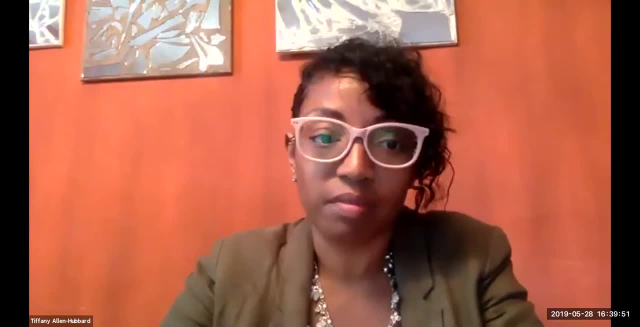 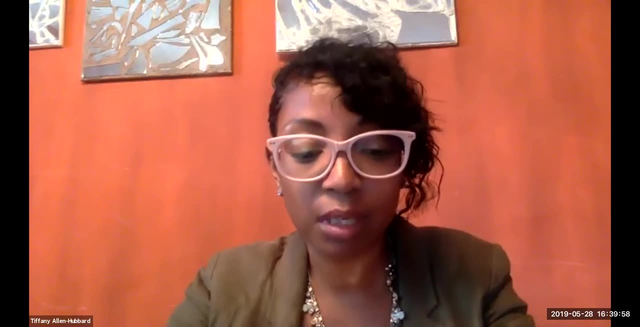 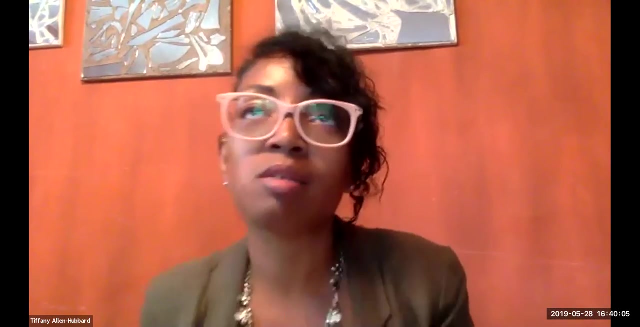 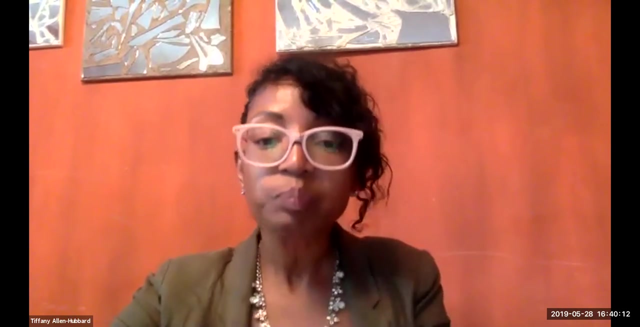 And a lot of our kids are screaming out for some cultural relevance. They're not seeing it. It's not in our history curriculum, And most recently in high school, the history curriculum has kind of been whittled away, And so I think it's really important for us to be able to go down into European history, So everything else doesn't really exist for the kids, and you have to see yourself in history in order to understand that you can also be a stakeholder and that you can change things, as Deanna said. 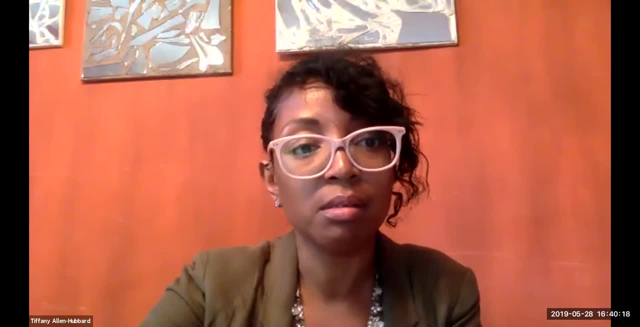 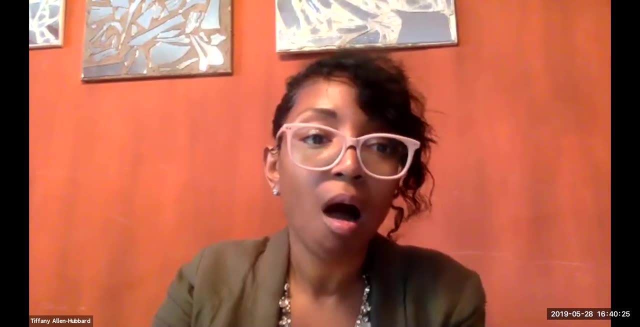 I think it's important also to have key partnerships with organizations that are willing to help Mentorship with the outside community. We have plenty of people in our communities who are vetted and or can be vetted and willing to help and work with students into different fields of. 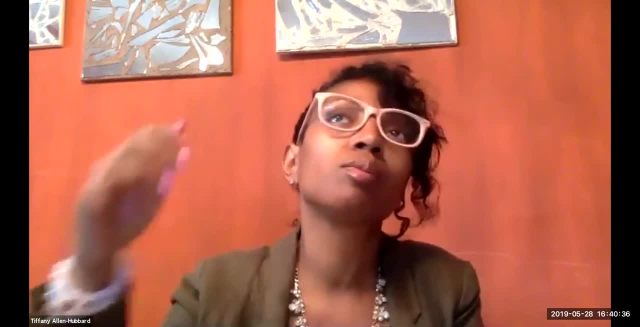 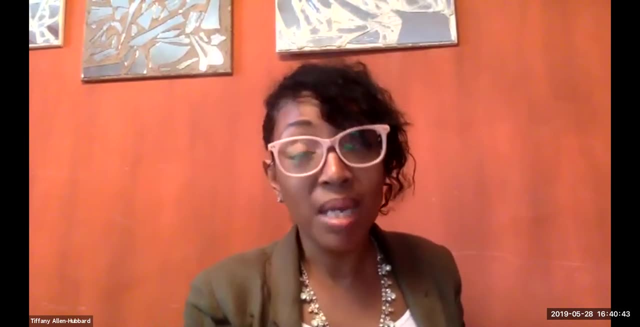 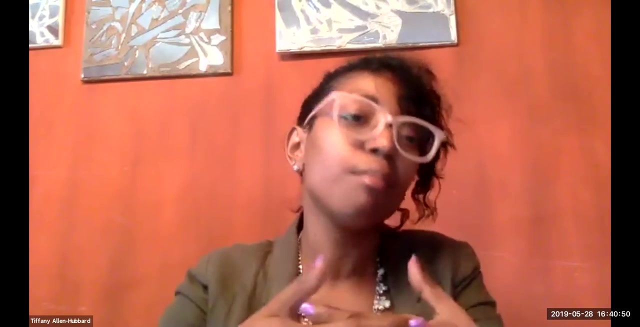 different fields of study, different ways to organize, etc. We're not taking advantage of this right now. Right now, schools exist in a bubble. They're just in the communities- many of them- but they're not really intricate parts of the community. There's not this real, this tight bond. We've kind of moved away from community schooling. 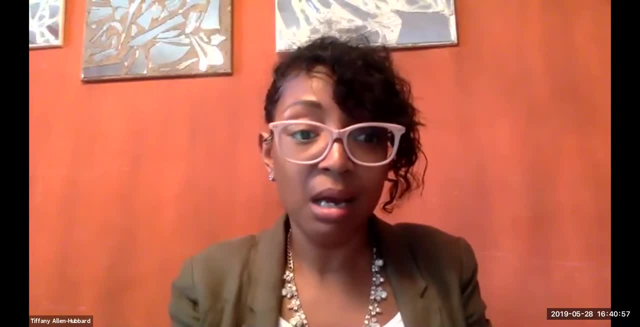 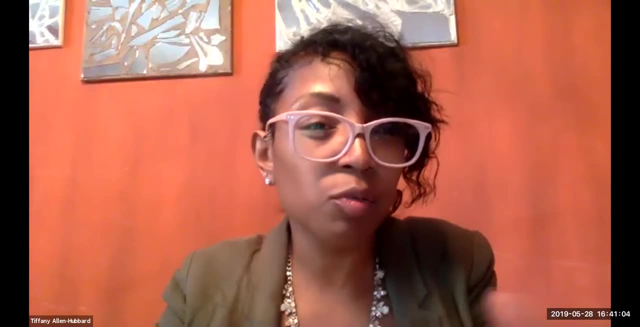 Where students, especially in New York City per se- probably not in Leah's district but in in our district- students come from all over the city to go to the schools and so we don't necessarily have this local connection and we need to make those local connections stronger. 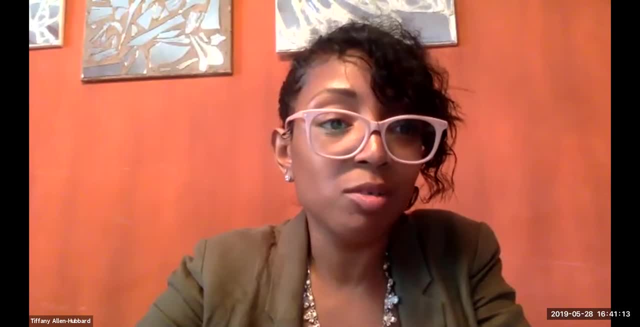 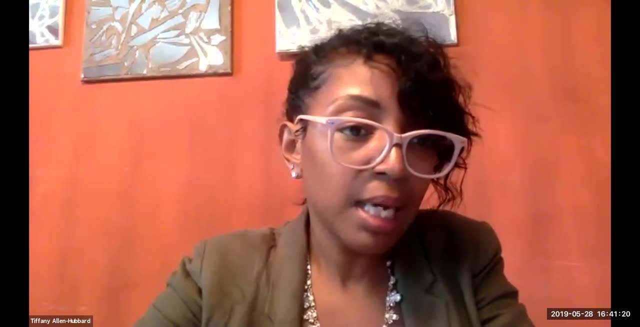 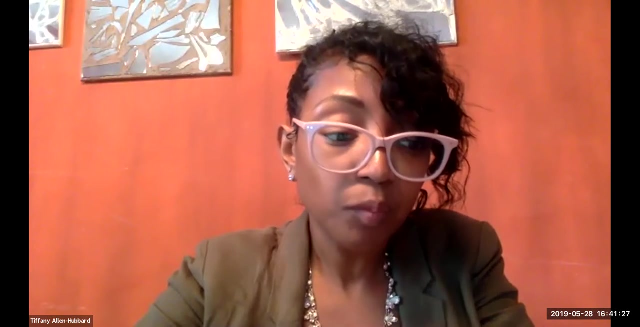 and I also think that schools creating internship opportunities for students. I think that that is key. That was one of the things that changed my life. My very first internship came through my experience in Benjamin Cardozo High School in Queens, where I interned in the district. 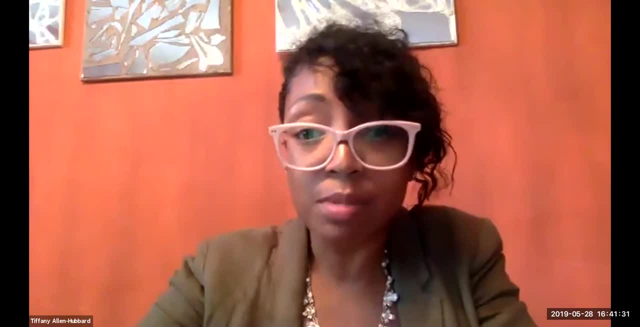 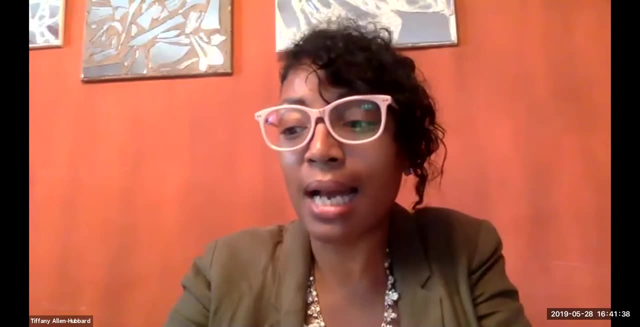 in the Queens District Attorney's Office for the summer and that was my first experience to see how like the District Attorney's Office works and what was happening there and to determine whether or not I did want to pursue the field of law or education or what really matters. and I 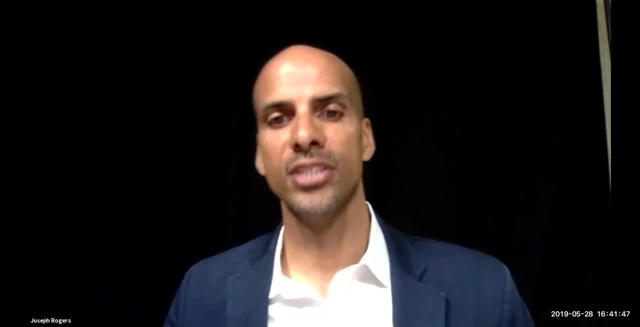 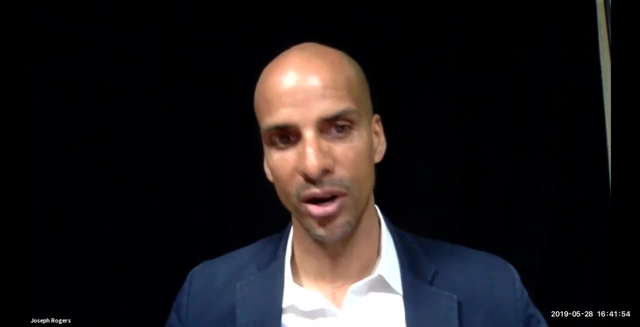 don't think our students see enough. How did you find that internship, Tiffany? if I may ask, Was that a school-based connection that was made where other students was it required? was it part of the school program to help connect these dots, for it to provide? 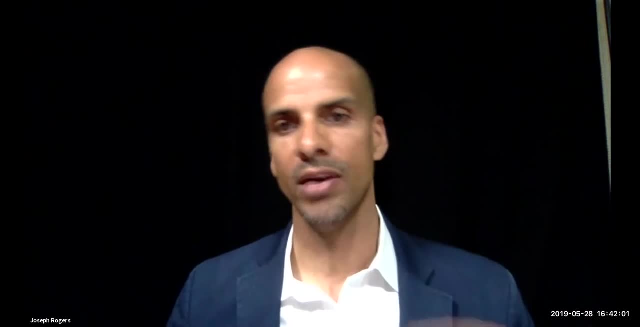 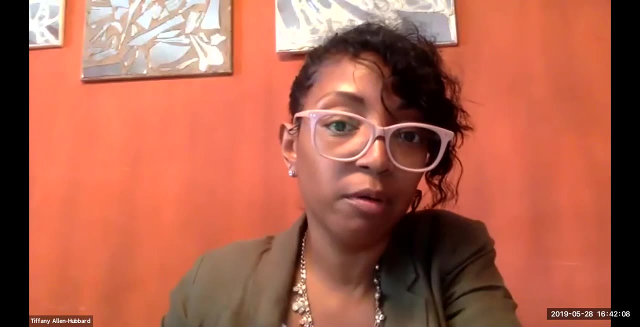 Internships, or was it something that you happened upon sort of outside of the school? Well, it was definitely a school organization and I was part of a program called the Public Service Program, and so they kind of courted students in the ninth grade to say, hey, do you? 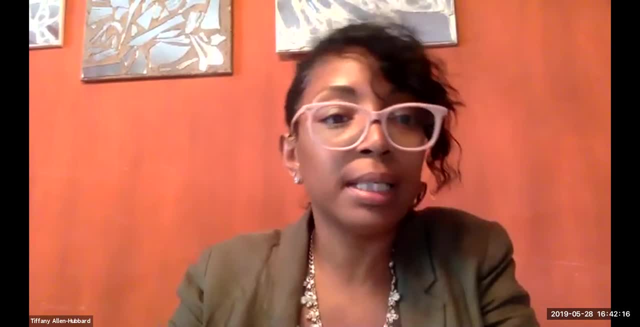 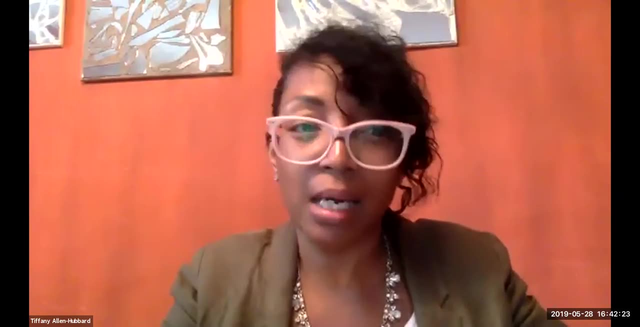 want to be a part of this. You know, if you're interested in law or anything in the public service, this might be interesting to you. and we took a bunch of classes and we went to things we personally- this was way back in the 90s- we personally, like- advocated for. 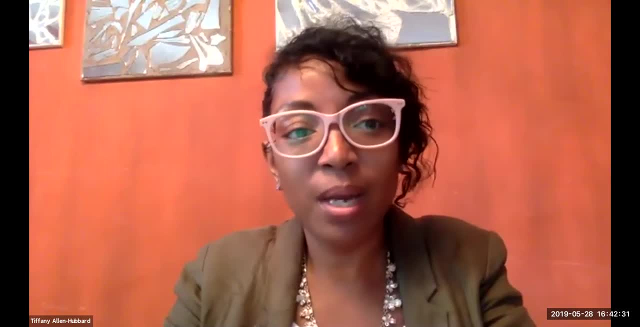 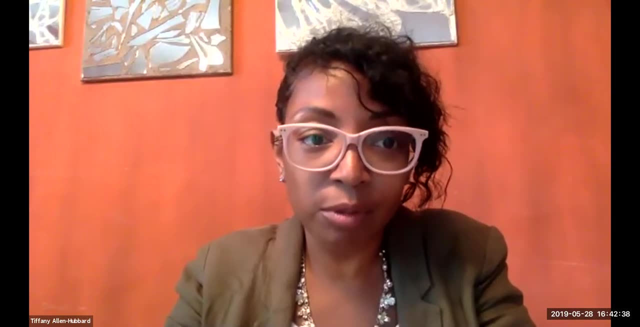 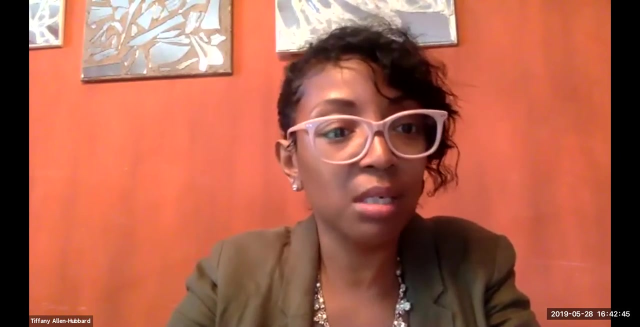 for different things. We we visited wards of AIDS patients. We we looked at some of the issues that were most like closely affecting our communities and our school at that particular time. and then you know, we had several like English classes and social studies classes that 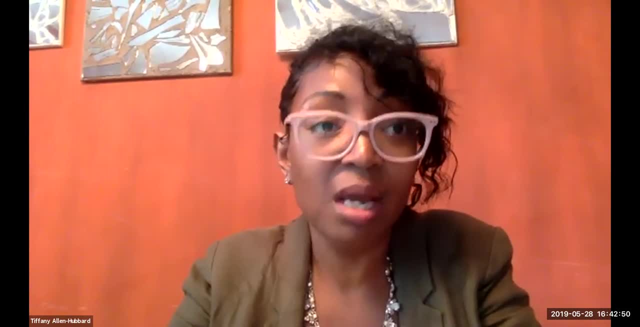 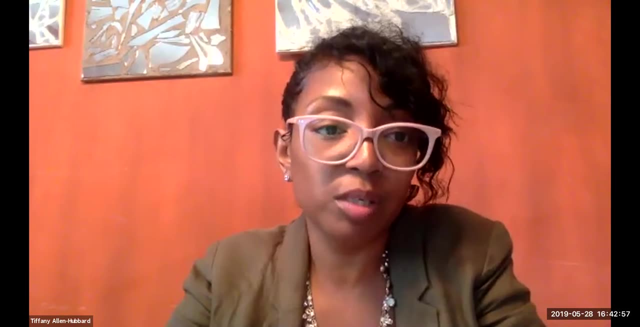 focused around this civic type of education and at the end of the 11th grade year we were all taught to interview and, and, and they had various partnerships with different areas, different organizations in the city. Like. I don't know if that program still exists, but like. 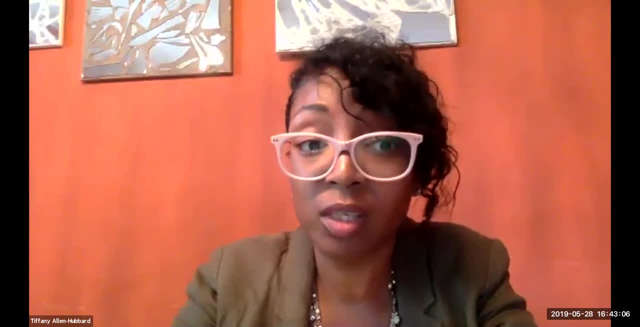 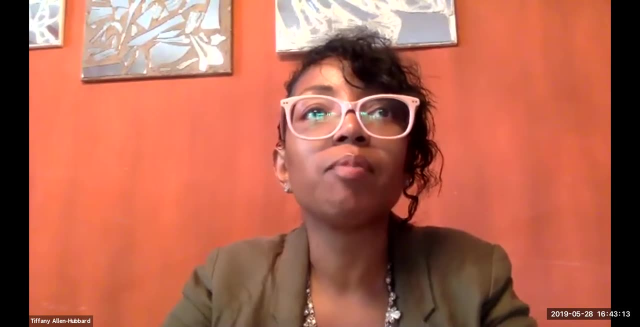 they had a partnership with the, the Department of Corrections, with the District Attorney's Office. There were so many different things. All the students did something different and- and I want to turn, if I can, just a minute, for a minute, Tiffany, because you're giving us a lot to chew on there- 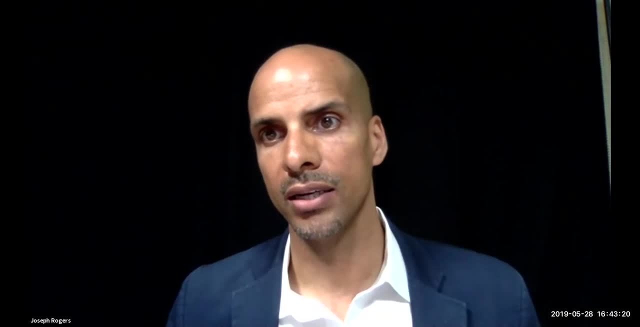 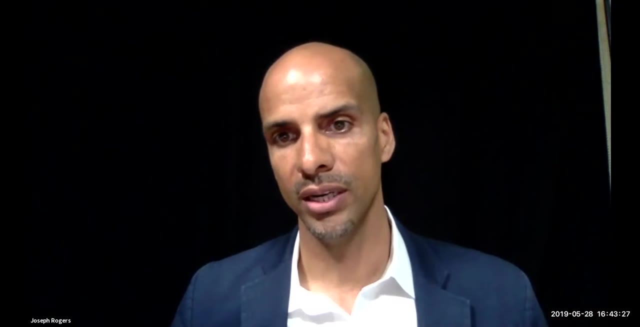 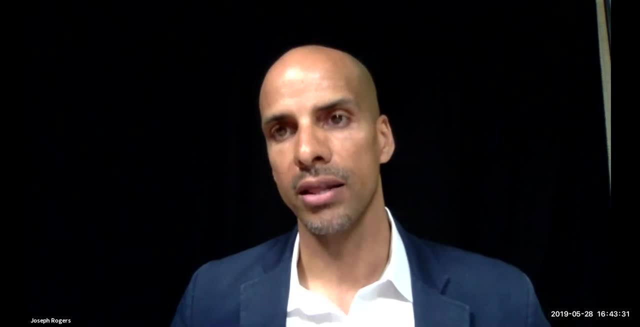 learning skills that were called out to her, So there were some things that she had that taught her about the law and about government through that program. We heard from the two of you. there are certain things that schools can do to better support students and each of you. 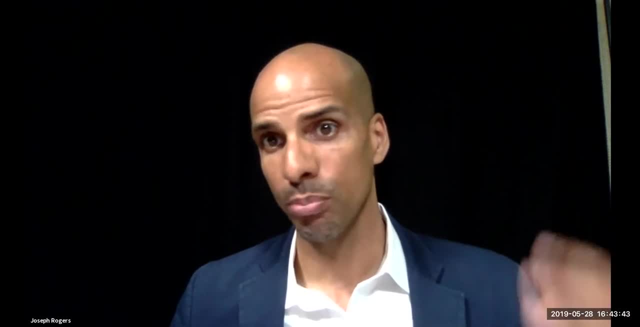 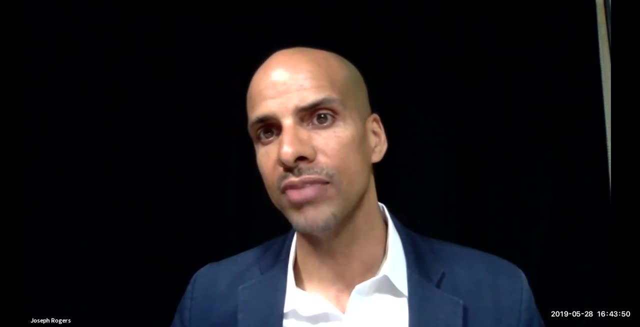 emphasized that experiential right, That hands-on practicing civic skills. Are there things that either that your schools have or that they don't have, that you think are essential? I'm thinking you know Leah was talking about, or I was asking her about. 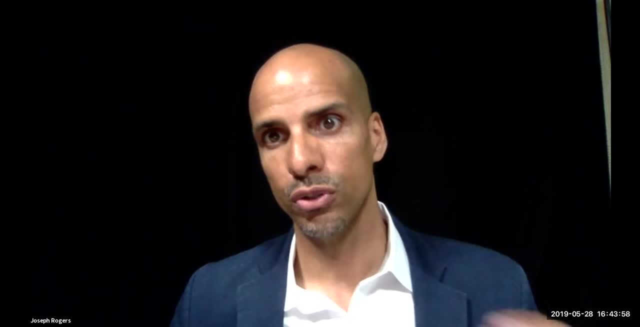 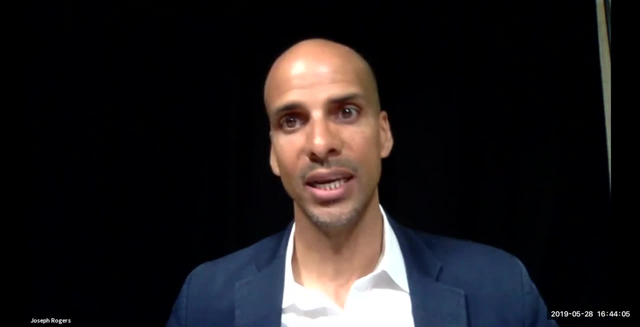 staffing right Is there? is there a person at the school who's用 a bunch of services, who's responsible for connecting all young people with- whether it's in the school or outside of the school- some kind of civic learning, internship or project based opportunity? because I know that. 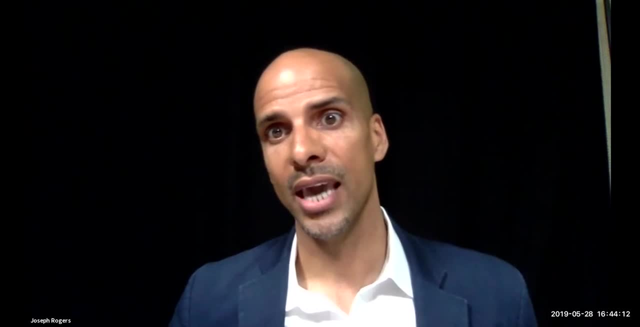 takes a lot of work and time and energy And if you know, if you're not set up to do that, it can be very difficult. So, Leah or Hamza, for this particular question, is there anything that in terms of staffing or other supports that schools need in order to provide those kinds of 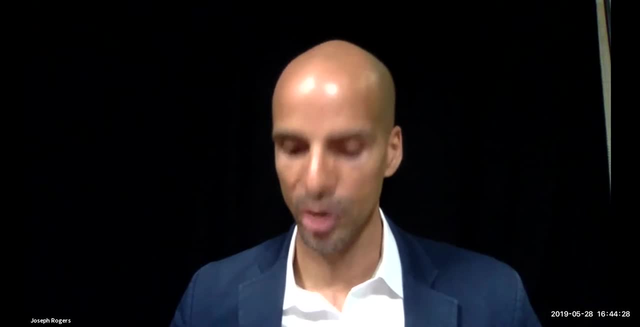 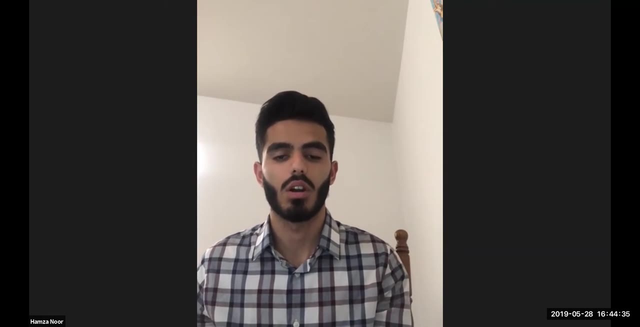 external project based opportunities beyond what you've shared perhaps. Um, yes, specifically in my school there, for me it started with our few clubs and you make contact with teachers there and they provide you with internships or opportunities that are. 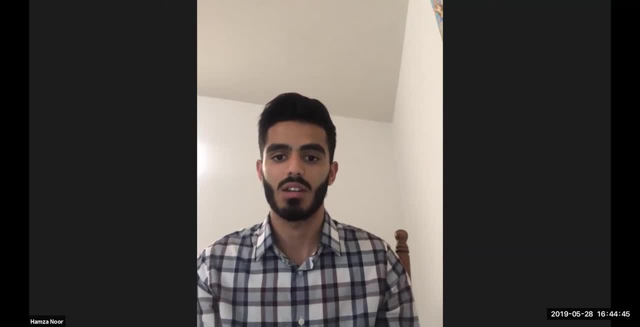 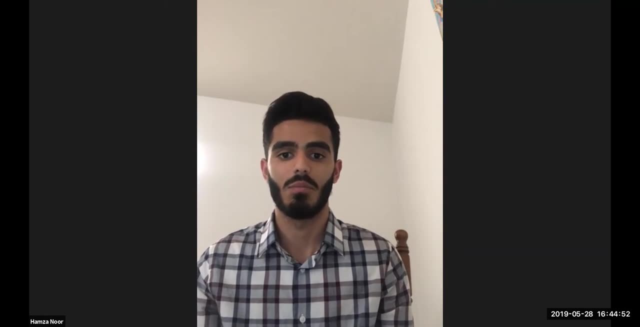 available in our community, But that's just specific teachers that dedicate their time to that. But now, like our schools, I realize how much those opportunities have, you know, benefited students like me and a lot of other students, And our school is working on this, this thing where it's, it's sort of like a like a. 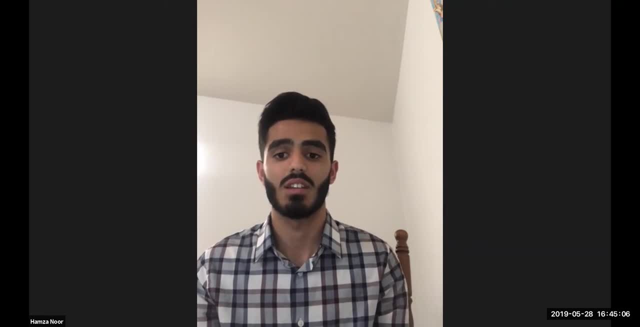 career fair, but like a community fair, where a lot of businesses and local politicians and a lot of firms that they're coming into our school over the summer and they're gonna see how they can provide opportunities for the students to have internships, work for them and in whatever way. 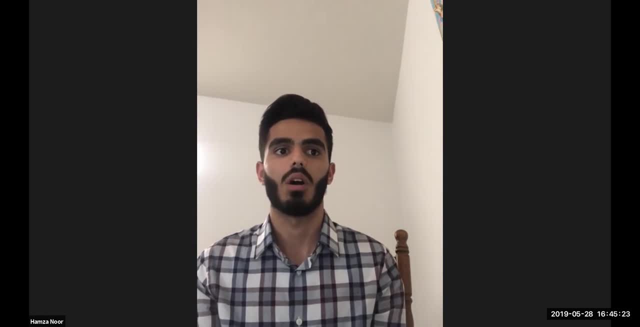 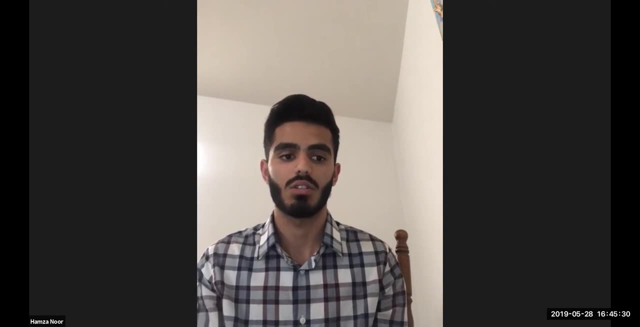 they can involve the students And our school has over 100, 100 community people or businesses coming in And it's just the our districts moving in the right direction And that that starts from the school And they have to reach out to these opportunities. 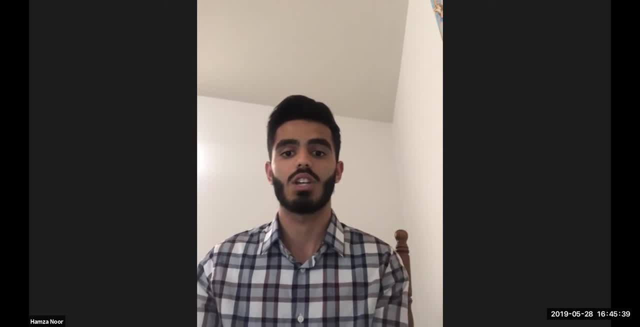 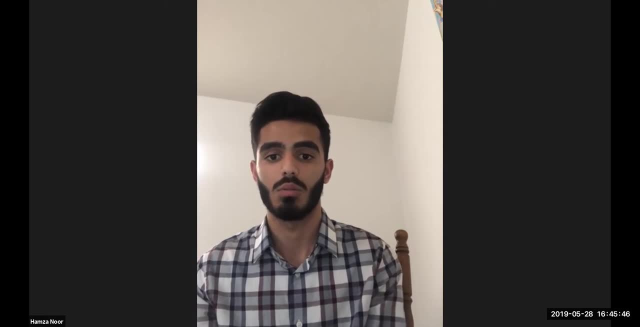 because they're. they're definitely out there in those communities And the school has to reach out to them and make them available for schools and communities, the businesses they want. they want their students to also get these skills by working with them, because they want better workers for. 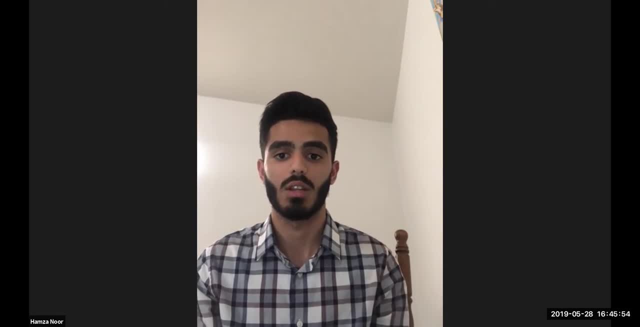 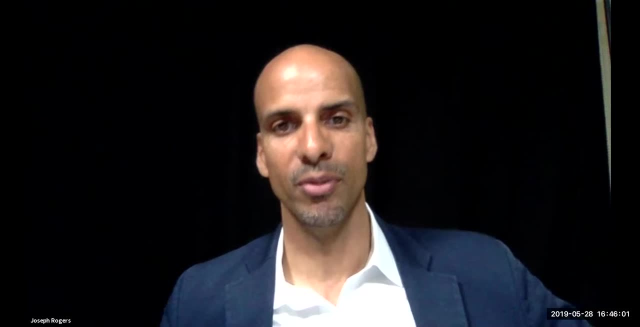 them as students come out of you know, come into the workforce and they want, you know, students to be able to be prepared with those skills. Emerick Bouch, You're connecting the dots. ہمزین, you know, as you mentioned, remember, from the very beginning of the presentation. 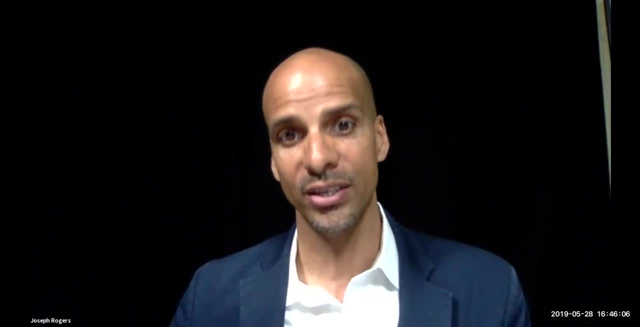 when we are outlining the constitutional rights, there's these two buckets right: preparation for civic participation and preparation for essentially a good job or competitive employment. You just connected those two dots here. But some of the skills that employers are looking for are similar, overlap with some of the skills. 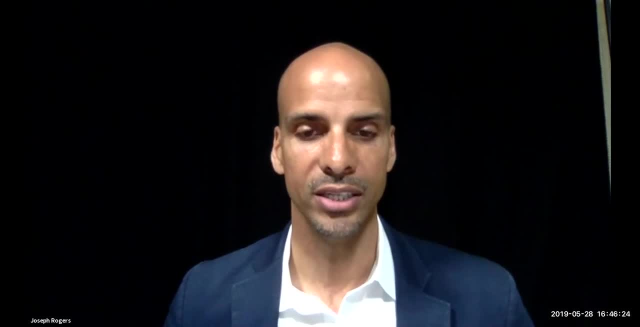 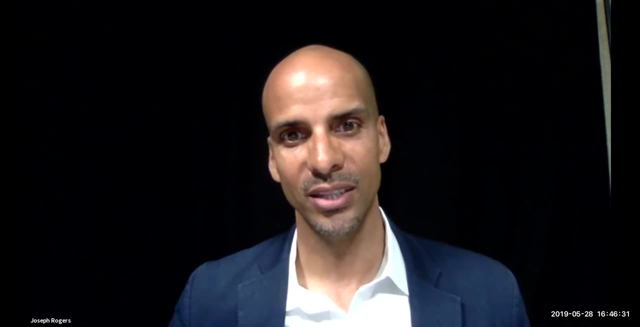 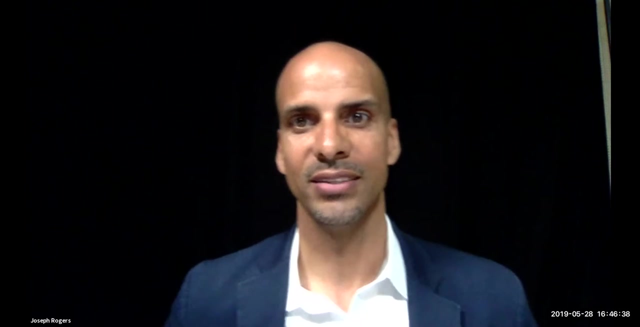 that are important and essential to participate in our and shape our democracy. A hundred businesses or a hundred organizations. who does that work in the school? Is there a specific person or is there a team? He just sort of catch-as-catch-can. you know, whoever has some free time they can fill in. 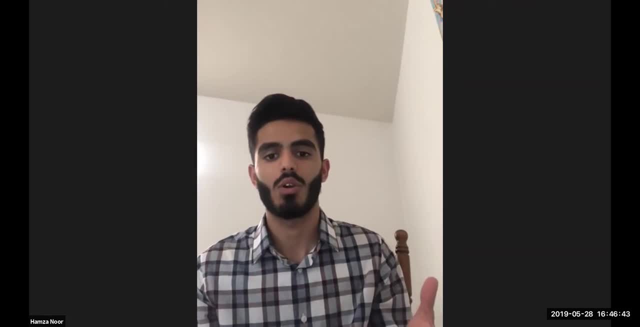 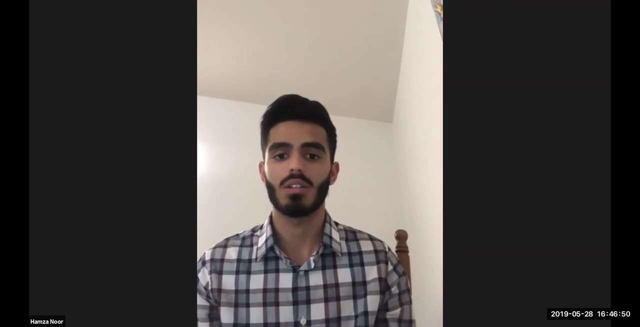 Well, our school has been doing this program. It's like a strategic planning committee that specifically has worked for, you know, months and has built plans and everything for how to make our school ready for 21st century learning. And this is a part of a subcommittee of that big committee and our 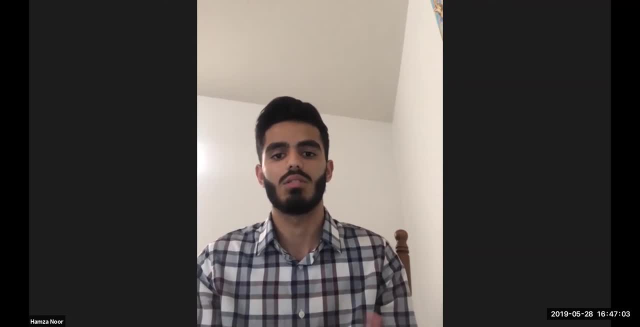 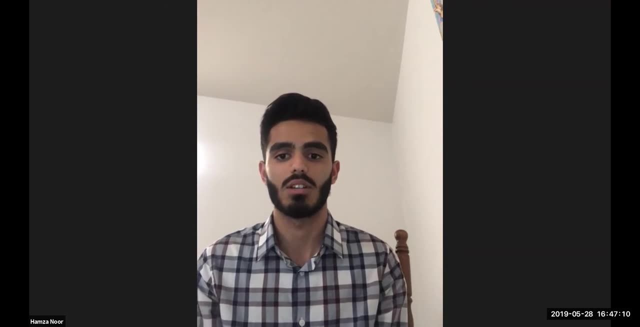 superintendent is leading it And there's, you know, different stakeholders and parents, teachers, and I'm one of the only students in those committees- but they reach out to whatever opportunity they see available And it's usually it's our superintendents leading the way, really. 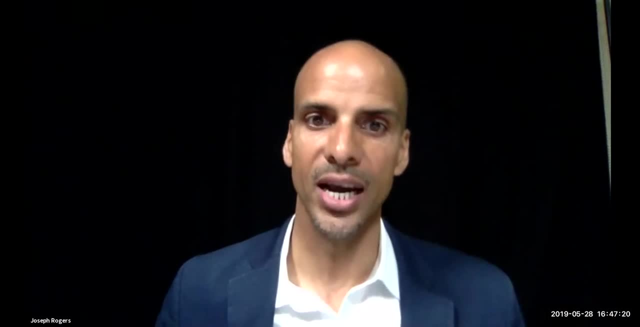 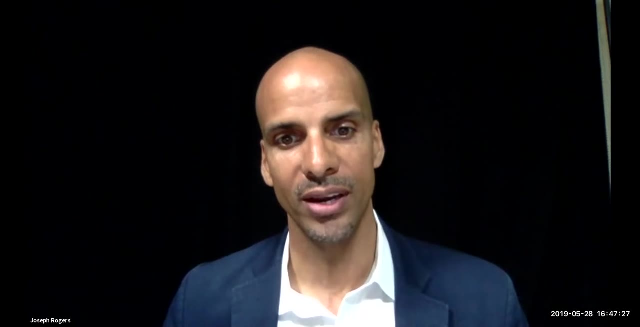 Leading the way, and it involves a wide range of people who are giving their time. So it's a question of: how do you, how do we research, how do we make sure that all schools, all districts are able to do that? So that's something worth. I think we can learn a lot from you. 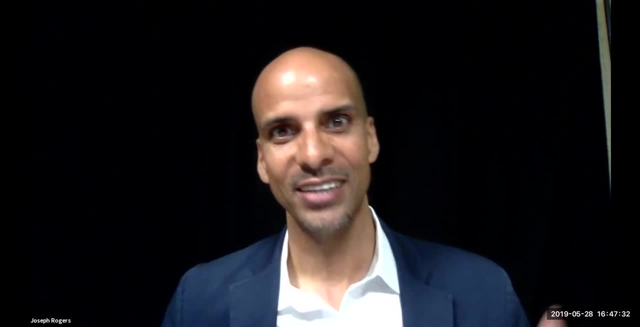 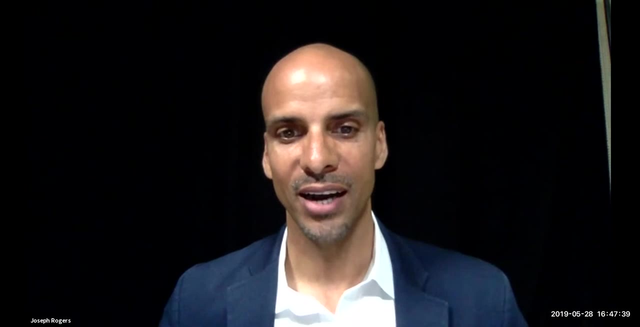 Like each of these, I wish we had a full hour really to delve into some of the opportunities and questions that each of our future stakeholders have raised, because it's so important and rich. So, but we'll have to do more webinars, How's? 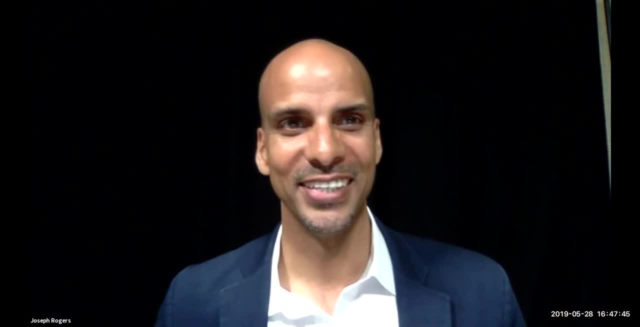 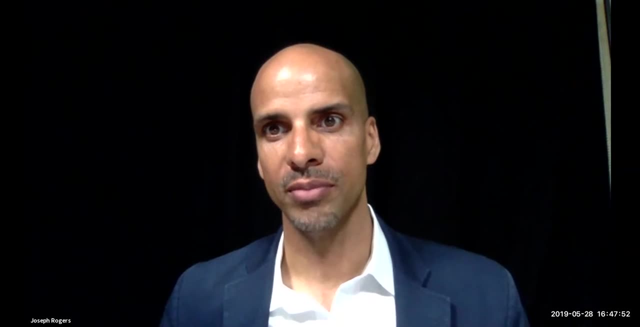 that Absolutely Daily webinars this summer, Anyone Okay? so again, I want to open it up for Aliyah. Did you also have something to comment? Thank you, Hamza. No, I was just going to say that we do similar. 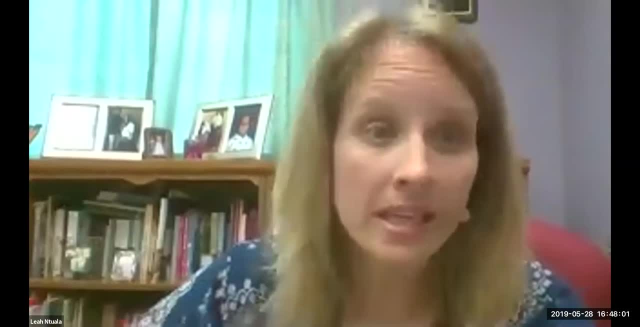 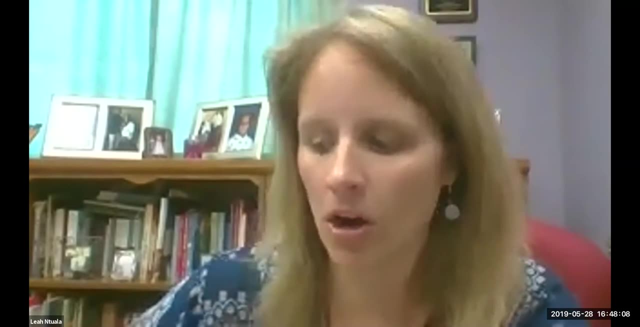 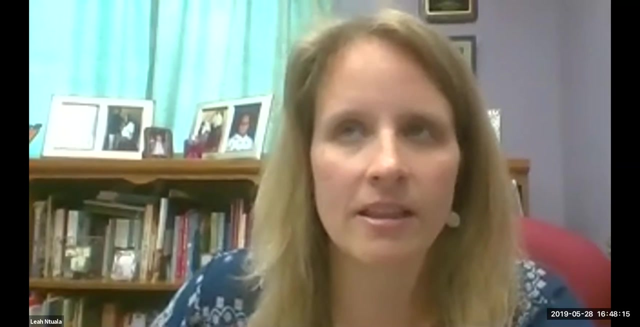 things in our district as children age up. but sitting here and being a part of this has made me realize that I know it's not something all schools do anymore, but our school district. they have character development, They have you know, they have school-wide assemblies and I think it could be easy if your 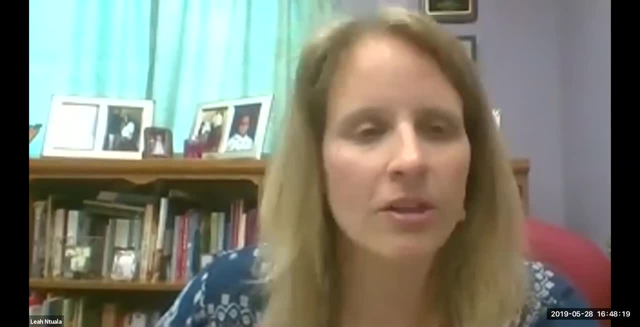 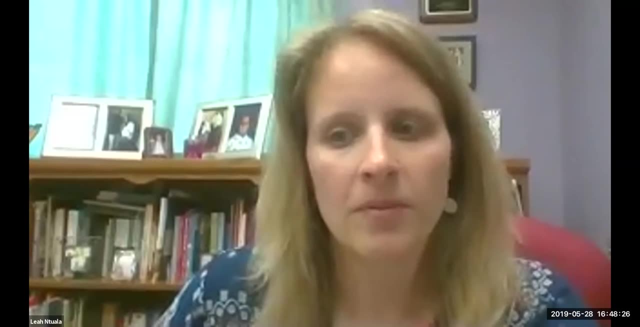 school already does that Sometimes. I think it's hard as a parent. you like the idea of something and you want to add it and you ask if it can be added, but the schools do so much that they have to do, But then it. 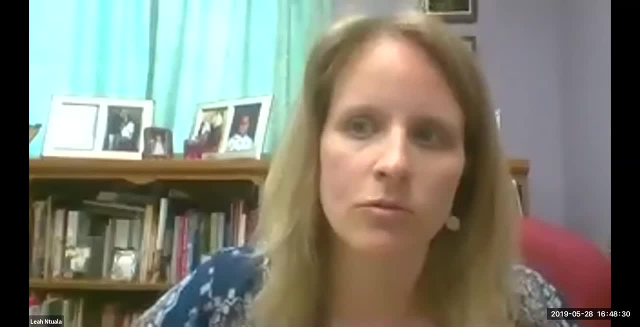 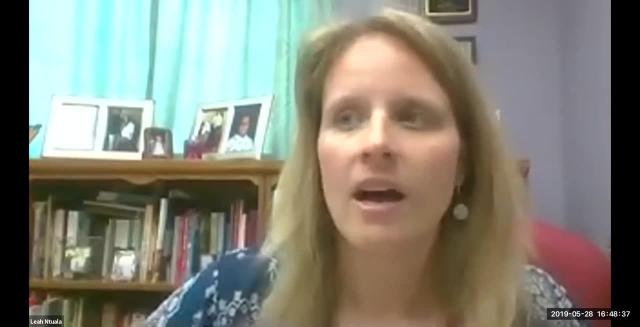 might be just asking the question: could one of those school assemblies that you do for the lower grades be focused more on some of these soft skills, job opportunities, things like that, so that you can just plug into something that already exists rather than adding on? 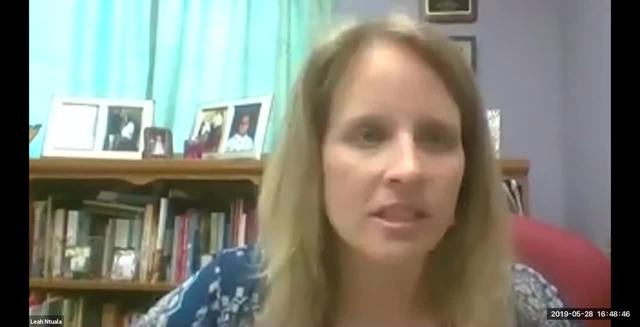 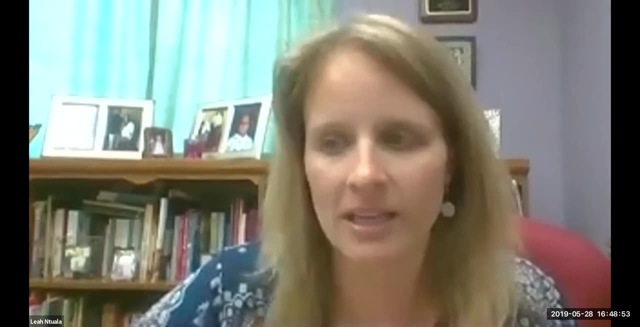 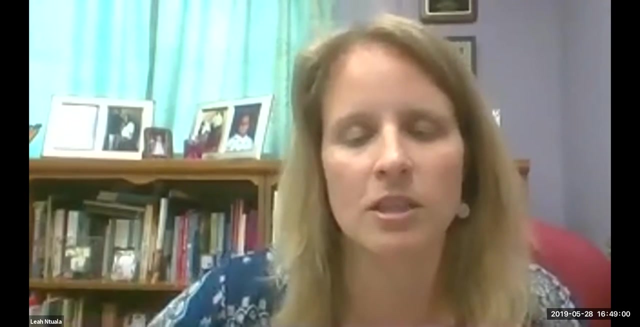 to the things that teachers are busy. volunteers are hard to find stuff like that, But a community member or some of the parents might be able to float 20 minutes to do an assembly presentation about the job they do or or do demonstrations on some of those soft skills, because I think the more you 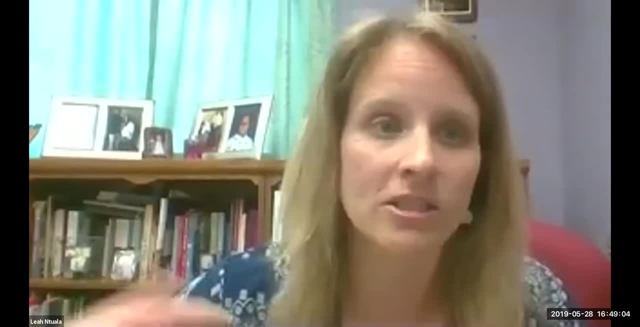 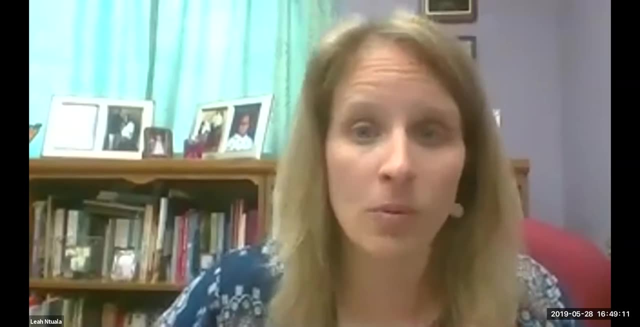 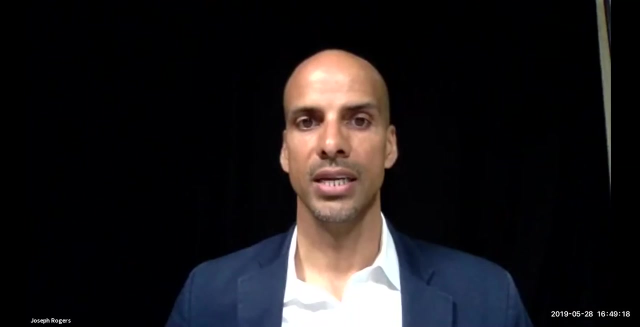 practice at a young age, the better you're going to be when you get to the place, where that's already plugged in to mentorships and internships. I think those are hugely important. Again, it's using your people as resources and not costing more money, Right, yeah, so it's always going to be a balance. What can you do with what you have for your school? Right, yeah, so it's always going to be a balance. What can you do with what you have for your school? Right, yeah, so it's always going to be a balance. What can you do with what you have for your school? 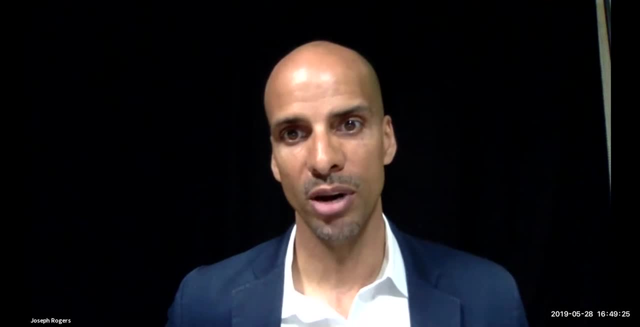 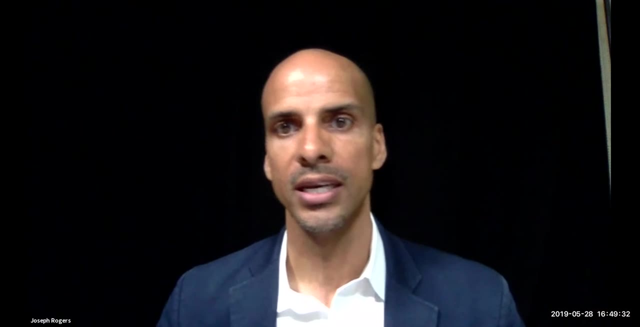 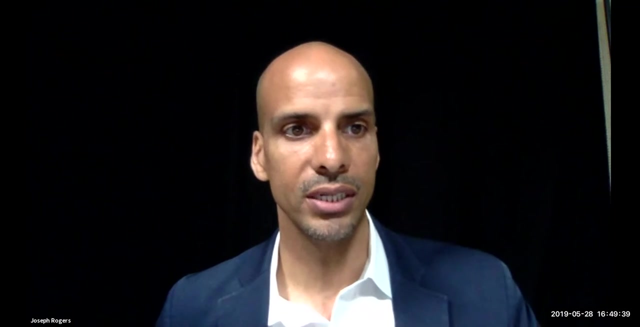 And then it's the extent that you need additional resources. how do you go about identifying what you need and then securing it from? you know whether it's the state, districts or what, or local communities? Thank you for adding that perspective. I want to also ask- and this is another question here, I think: 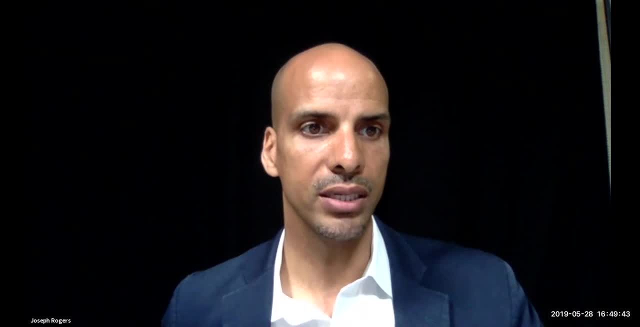 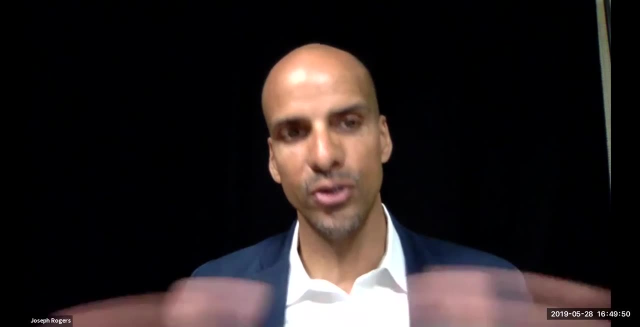 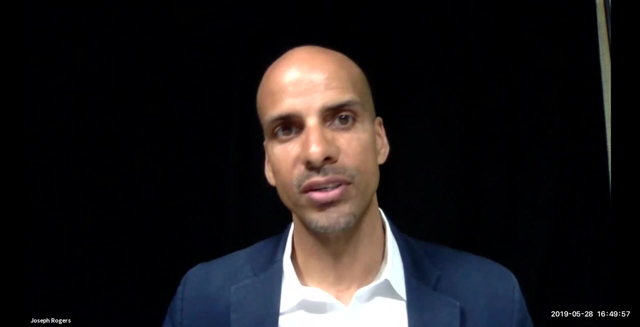 from in the Q&A box here that someone asked about, and Jay and Deanna, I'm thinking about you two because from four, two different reasons. The question is is, and I'm paraphrasing here a little bit: you know, not all young people are extroverts, Not. 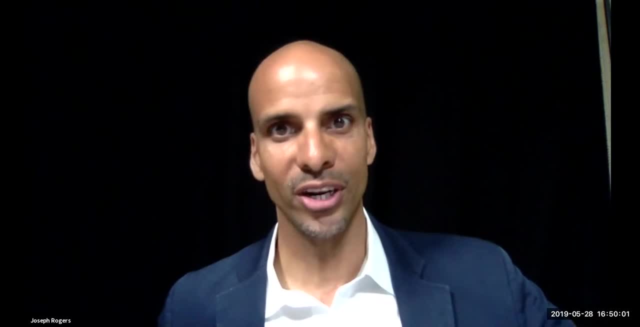 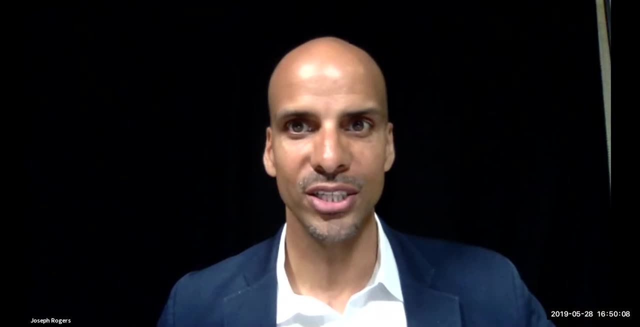 all young people are sort of going to be the ones who are going to go out there and petition or going to collect information from the community or, you know, advocate for an issue they're concerned about, or even just gather information, go around and talking to local community members. 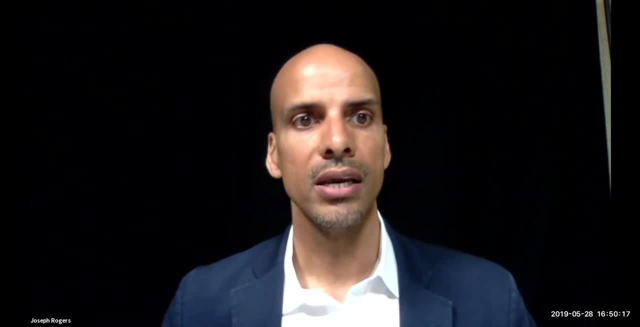 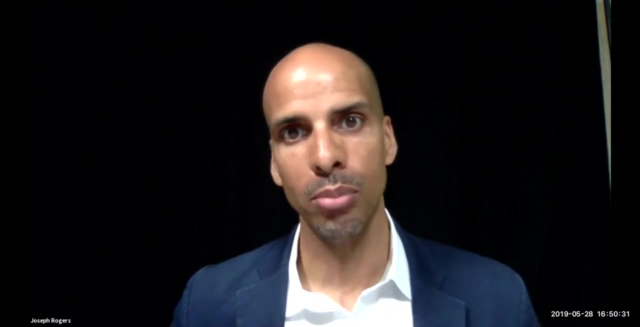 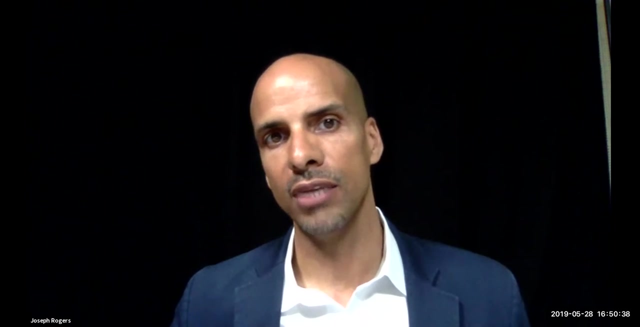 to better understand challenges and potential solutions. How do we help young people who maybe aren't as savvy, who aren't as maybe disposed to or don't feel as comfortable actively engaging in some of these more outward and public initiatives and projects? Is there a way for us, a way that schools can differentiate or really tailor these kinds of? 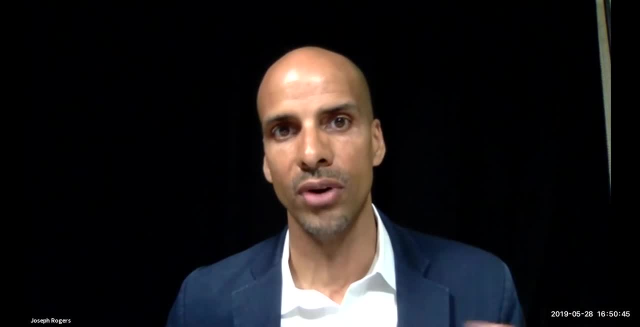 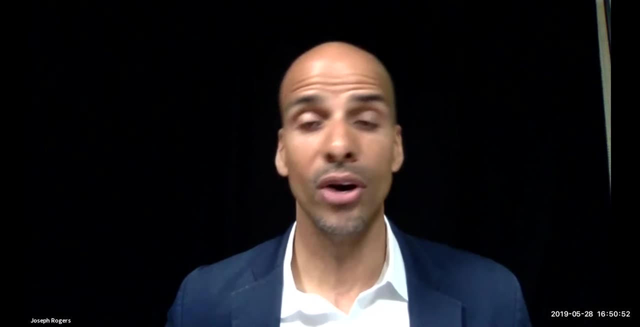 opportunities to different types of students, particularly with a lens toward social and emotional wellness and personality. I think that's I think that's a really good question, I think that's really, really important And I think we all have some- you know some- personality differences, Because we know that just. 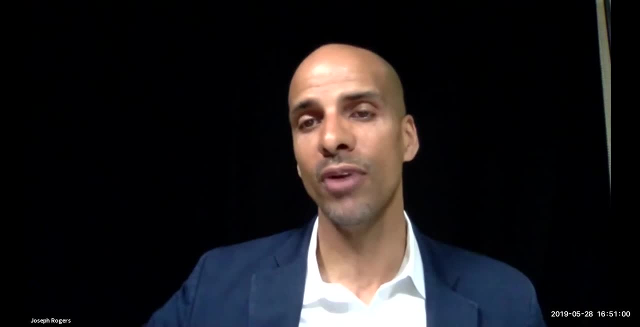 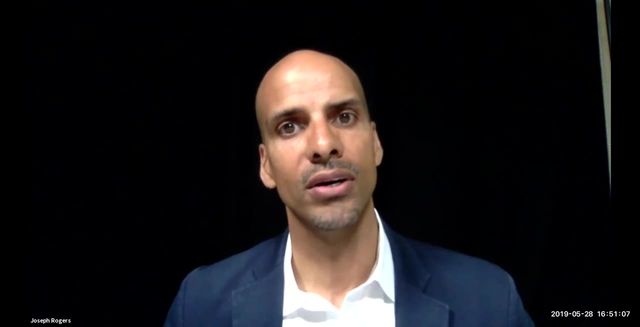 like we've heard here, at some projects and they work for a rural community or rural school district. we're preparing young people for civic readiness may be different in some ways, in some cases, from those in a really urban context or suburban context. So do you have any insights or 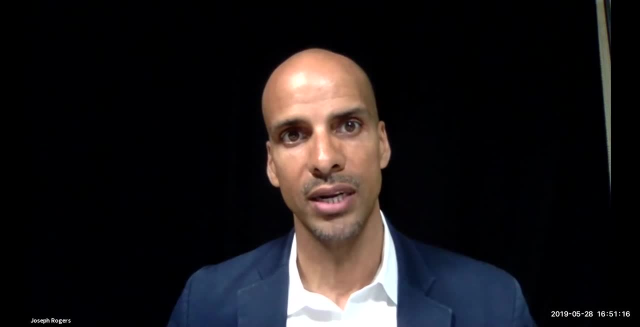 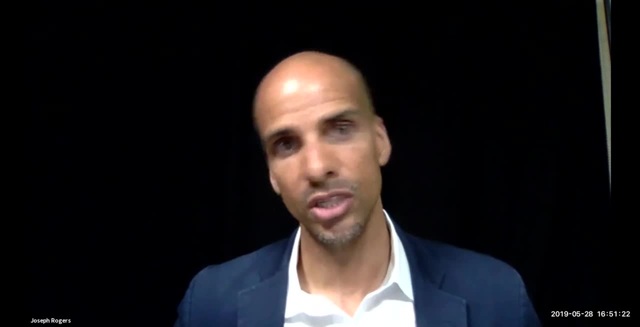 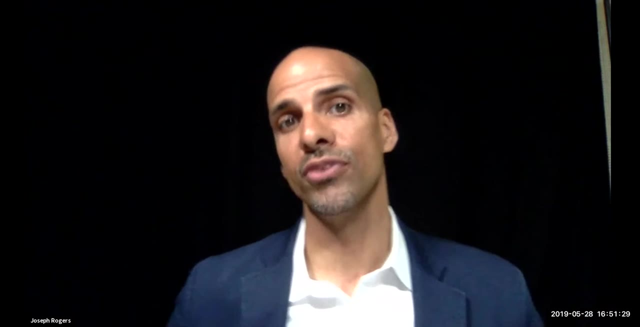 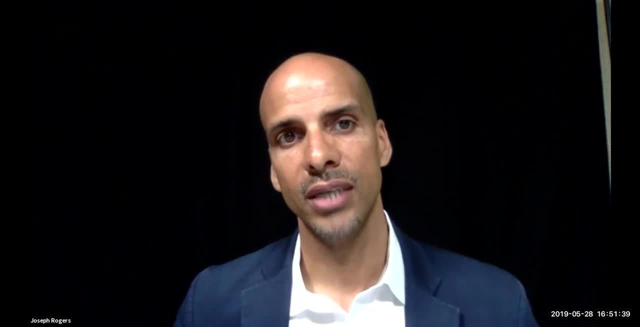 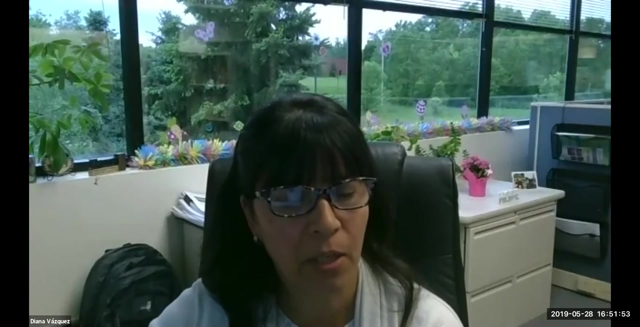 field. how do you- how do you cater to those individualized, personalized needs- recognize that young people access this work? this is learning in different ways. it comes to my mind that we have Hispanic students in our program that just arrived. their English is very limited. they get help for from the E&L. 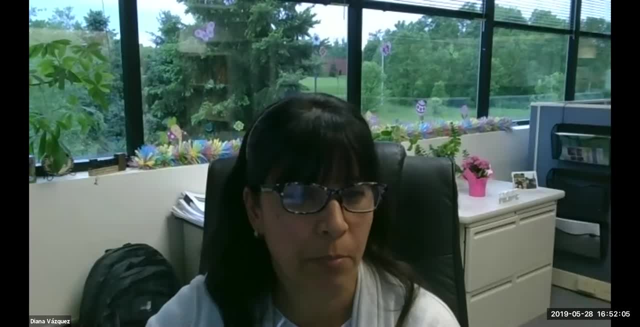 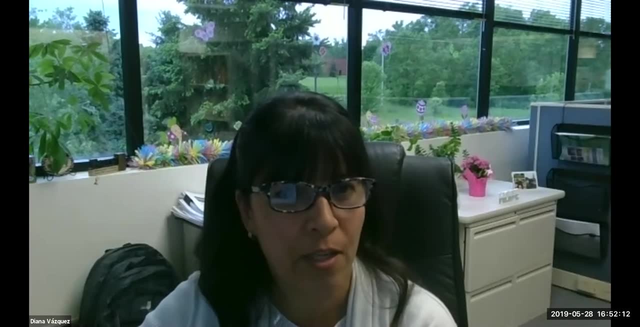 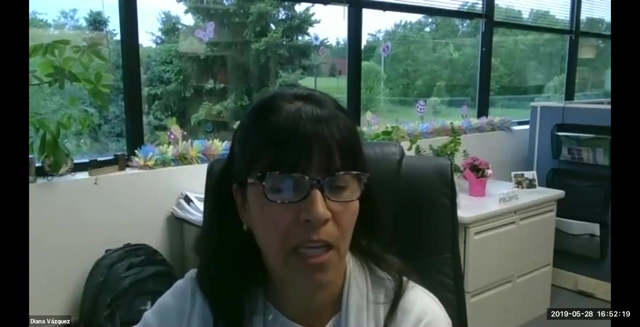 teachers and they are very close to us to the program because they recommend students to us. so these students are very shy at first. they can start the program in ninth grade and they just, you know, get a sense of what the program is about. they come up for the trainings, usually there. 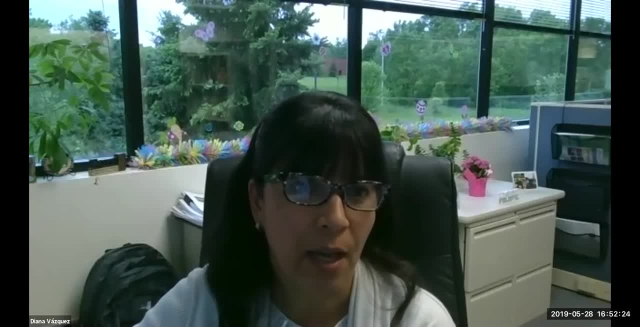 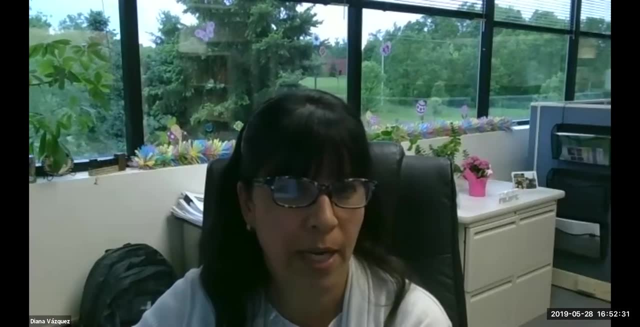 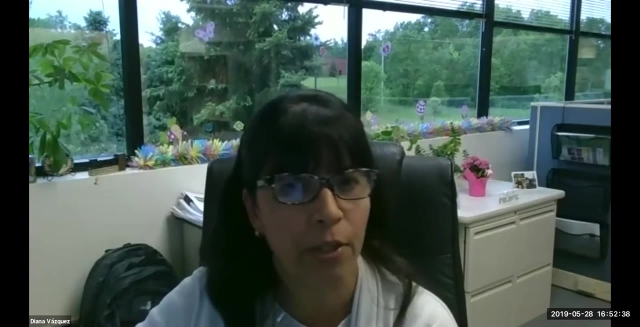 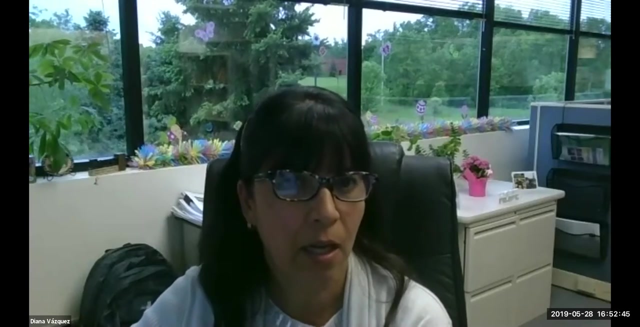 are Saturdays or after school and they start learning about the program and what we can do as a whole, as a community right. and by the end of the trainings that usually they start in November and go through March, they have, you know, become better at their public speaking and then 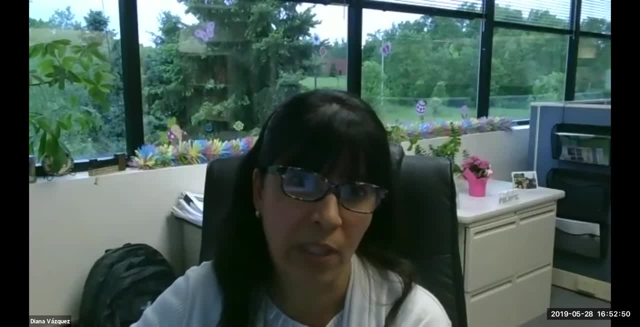 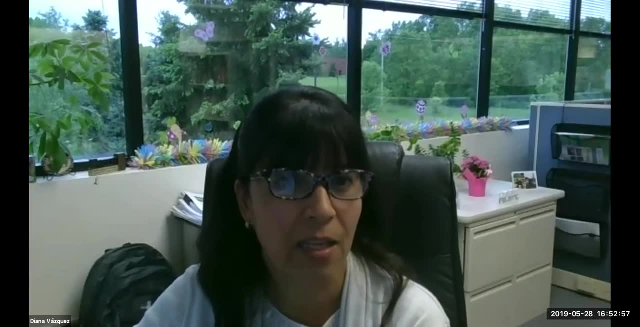 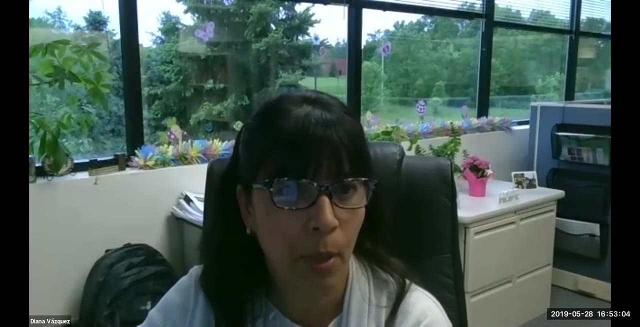 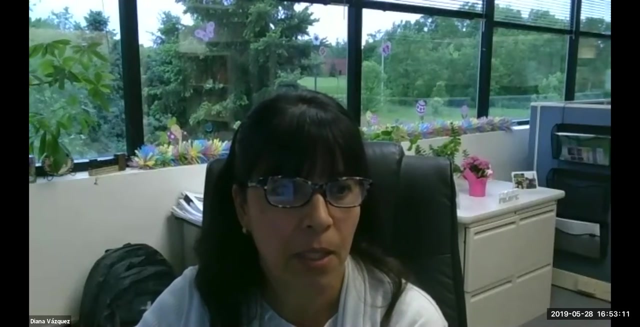 imagine them if they start in ninth grade, when they are seniors. oh my god. used to see them in the mock assembly debating for these bills, taking a stand, making their voice to be heard. so it's a process that takes time, but we give them the tools. we work with them through the trainings, the trainers and some of the 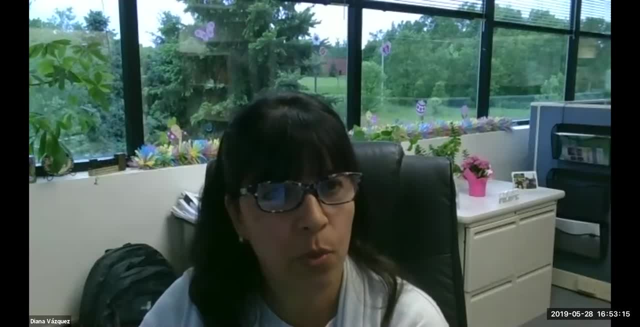 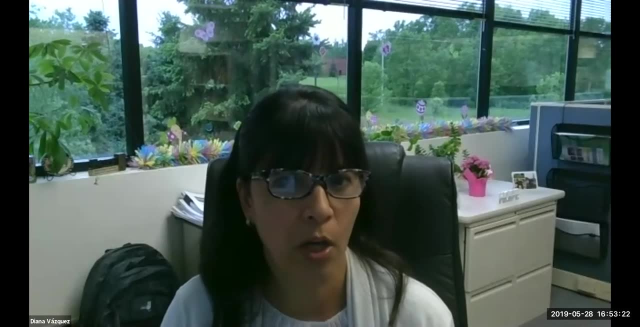 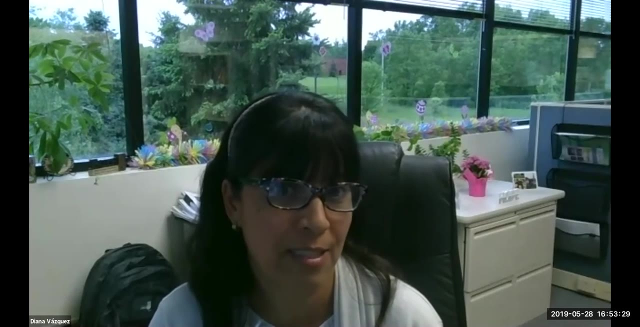 students that come back as volunteers. we really work with them and we give them the tools, we work with them. so it's it's like a little group here at the trainings and when we all get together in this private Institute in March we get. this year we had 255 students from across the state. we were all there at 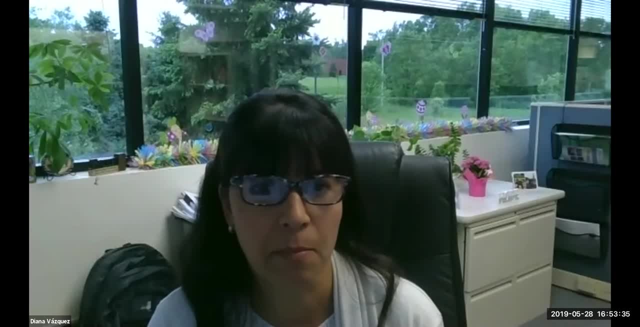 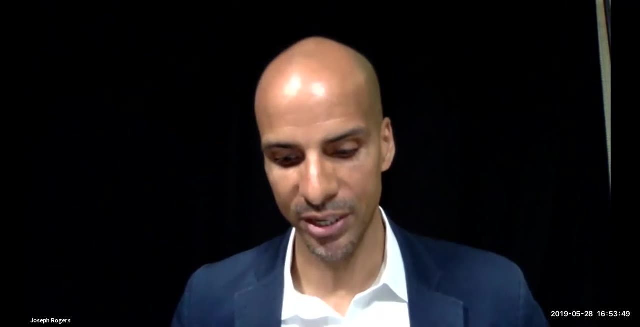 the assembly and they met people in and assembly men and congressmen. they were all there are senators and they were very impacted. so it's like you know, starting as little and ending as big, and it's really, it's really important you bring that perspective and you. 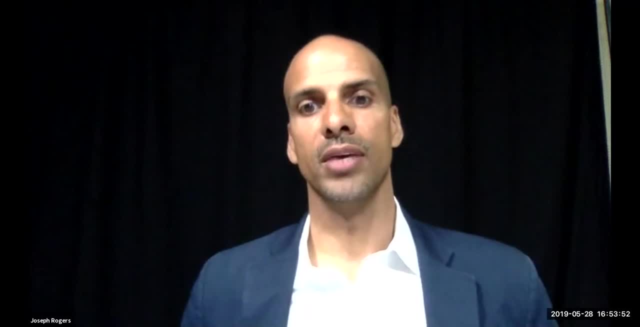 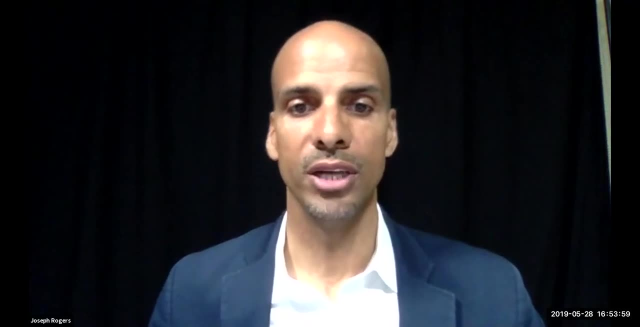 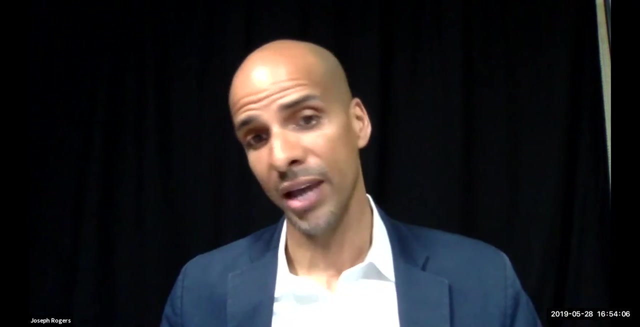 English language learners and English for for folks who are new to new to the language in some cases. I think you mentioned new to the country as well and you said you sort of start small right. you provide those supports. their schools select them knowing that they'll be supported and they're supported. 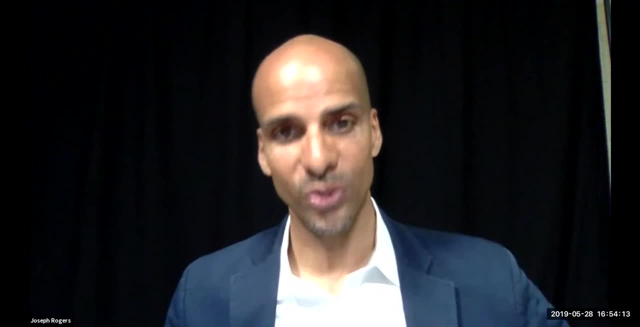 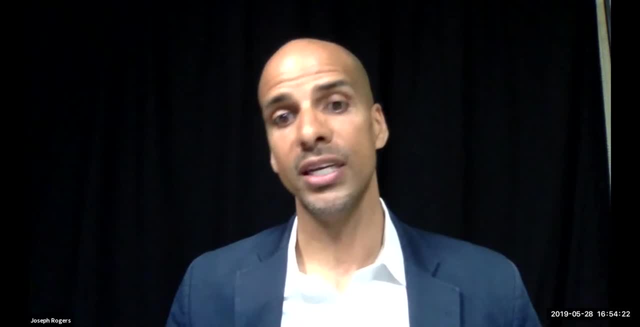 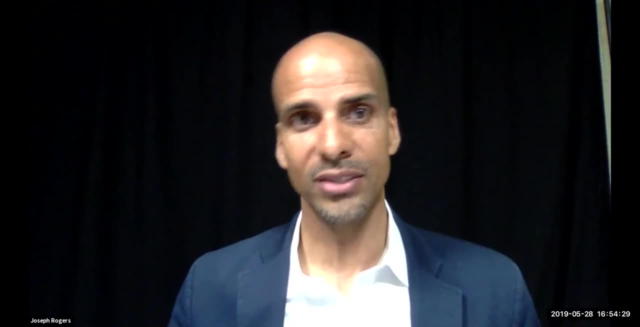 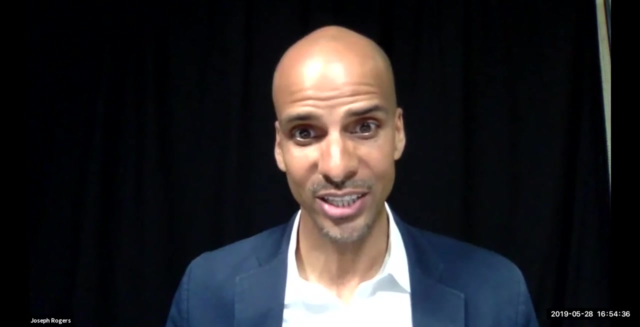 language skills, but it sounds like also in terms of their ability to participate as a civic participant. and that's really important to note is that the right, the constitutional right, doesn't only, isn't only guaranteeing these opportunities to students who, you know, grew up in the United States from an early age. this is 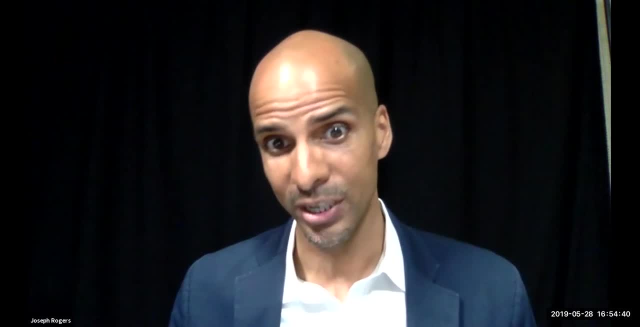 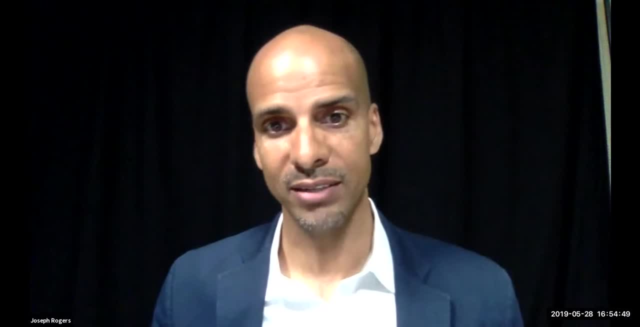 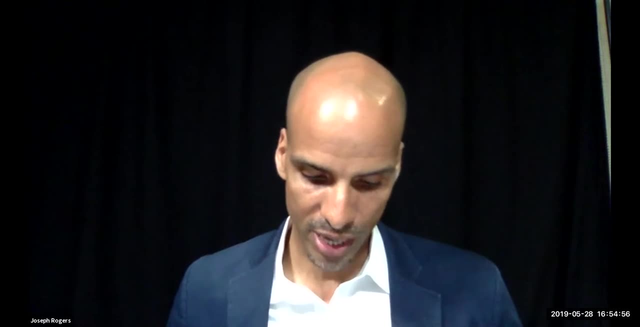 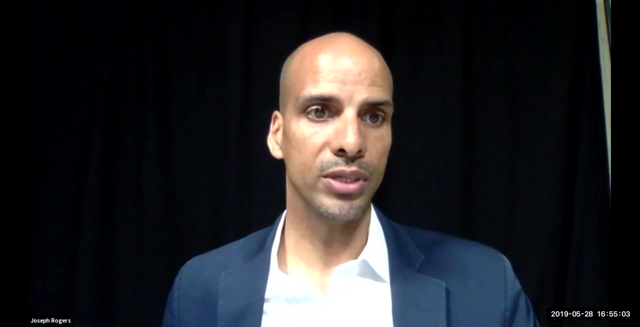 we can't stress that enough. so thank you for for that example from Pryla Jay. I'm gonna target it sort of a different question to you if I may, and that is it regarding. you talked a little bit, you talked to earlier about mandates and I see one of the questions in the question box here pertains to, they say, you know. 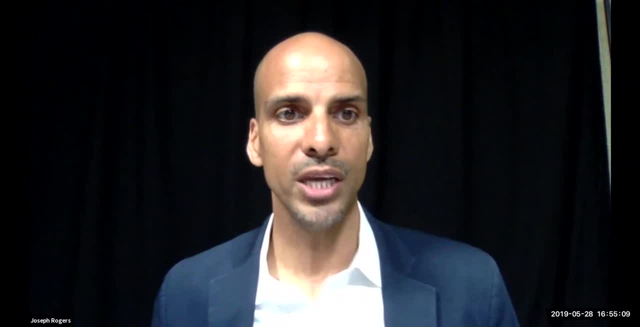 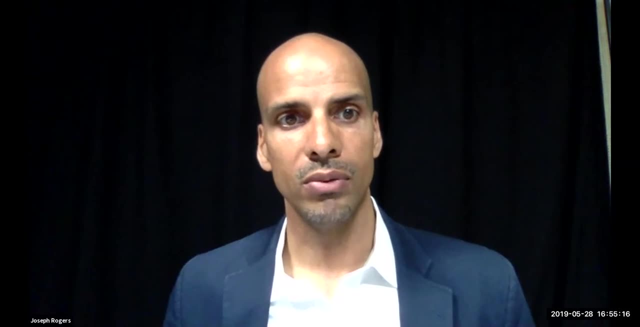 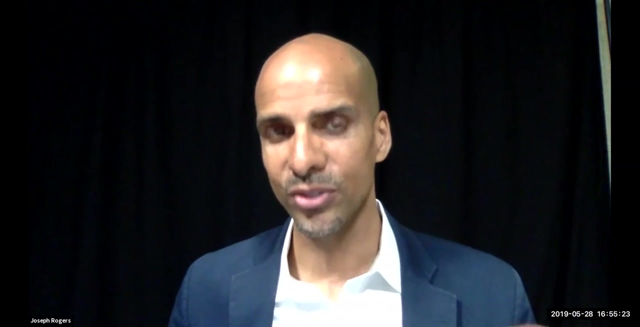 it's great, great to increase opportunities for community participation, but there's no guarantee in that, and what I think the this commenter or inquirer or was getting at is how it looks like there's some, some language about accountability. how do we make sure? I mean your school boards, I know school. 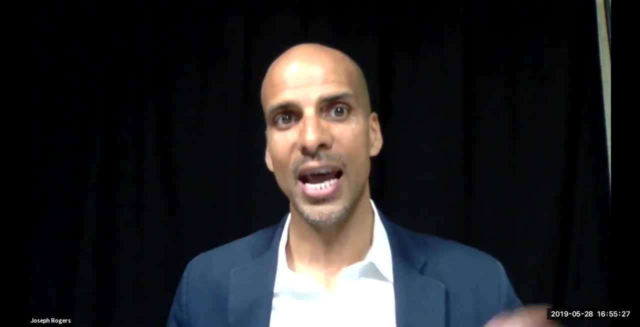 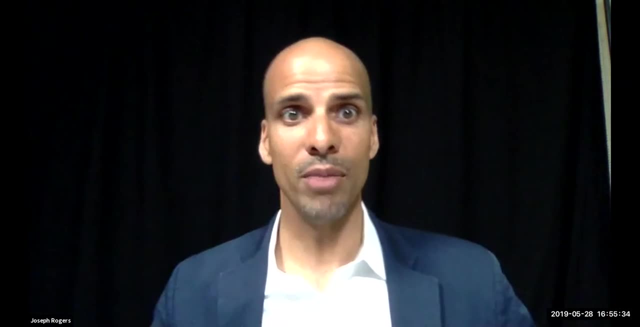 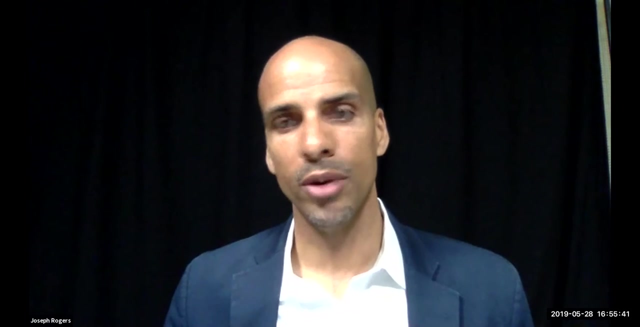 boards often aren't fond of mandates and you mentioned, if you're gonna add something, require our districts to do certain things or school boards to do certain things. you could help us figure out what we might have to reduce or shift a little bit or do differently what? what talk to us for a moment, if you. 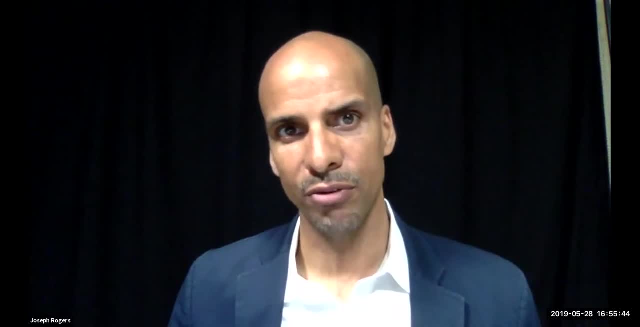 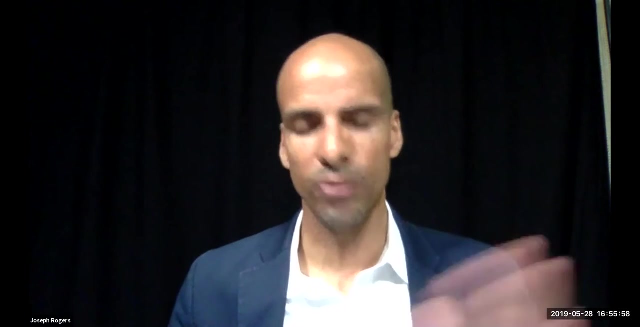 would about accountability and how it sort of at the state level. how can the state implement an accountability system for civic learning that it accomplishes the goal of making sure all students are fully are civic ready? but that doesn't get into some of the sort of avoid some of the snafus, some of the challenges. 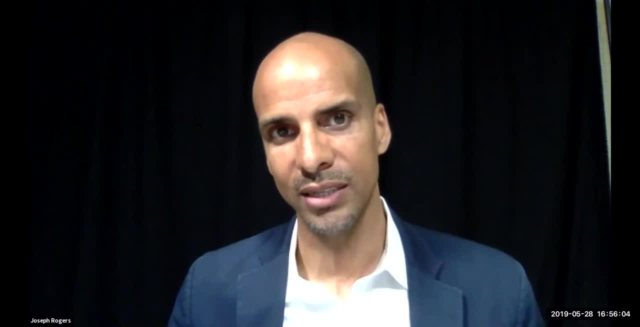 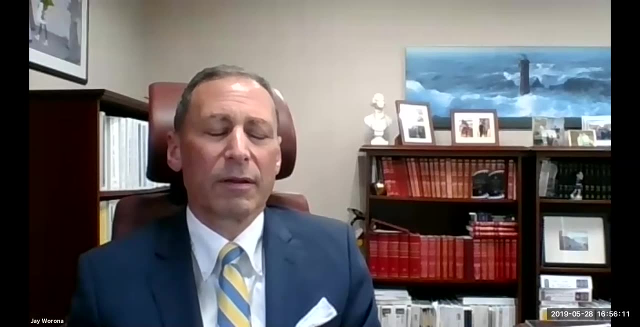 that may be unnecessary in the process. what does, what is the ideal accountability system for this look like for you right To start with, I think, Joe, accountability, you know, would be best determined by the local school districts. I mean, if they're not doing their work, then I think they would be in a bad position if they were to step out of school. 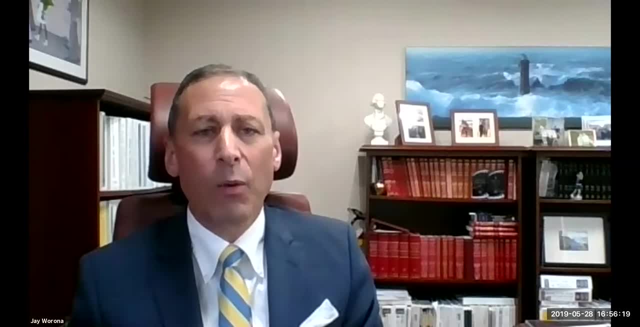 their job, then perhaps the state needs to step in, But I wouldn't presuppose that. you know, a local district would not be able, if they had the right resources, right, would not be able to make appropriate determinations as to whether they have accomplished their goal of getting. 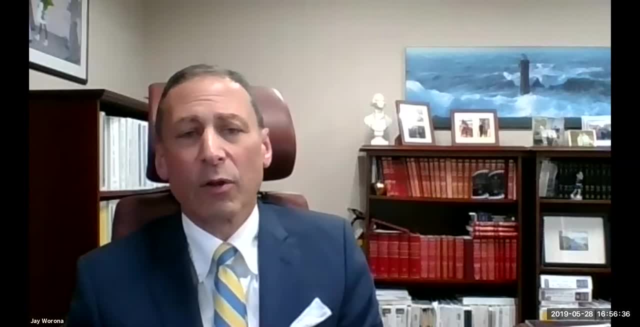 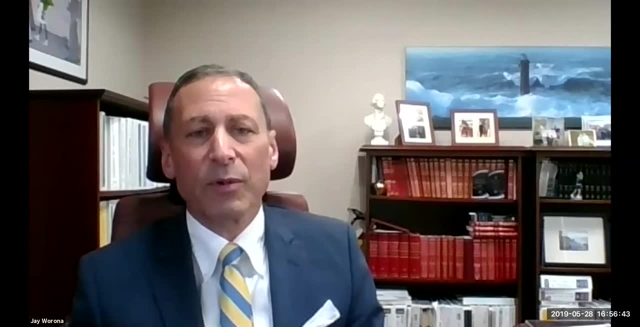 these kids proficient in civics, learning right. So I think the local districts would be able to make that determination. But again back to what I said before, that all becomes impossible if the resources aren't there to provide the opportunity to start with. So you know, obviously I, you. 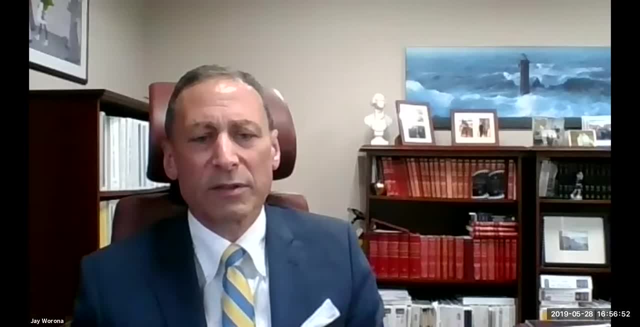 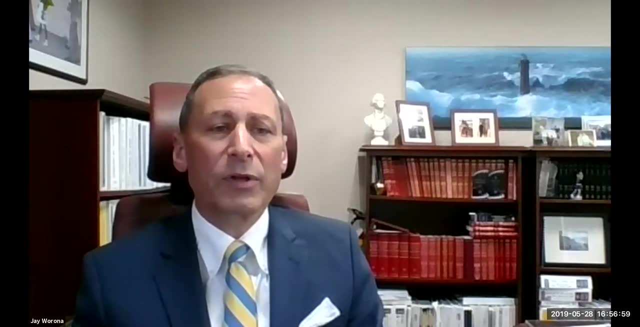 know I would leave up to the educators who are on this webinar the best way to make those opportunities available. but the opportunity has to start with money and resources to be able to make sure educators can go off and do what they need to do. 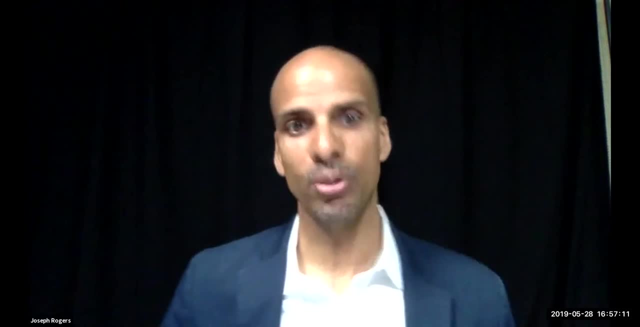 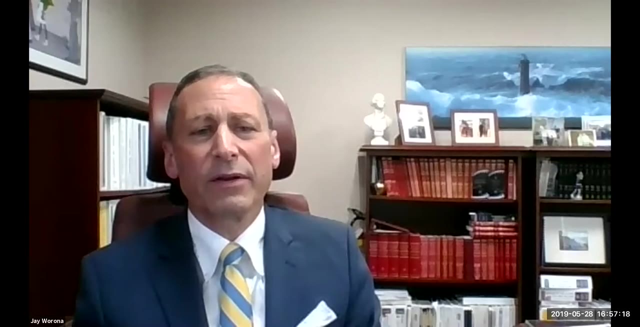 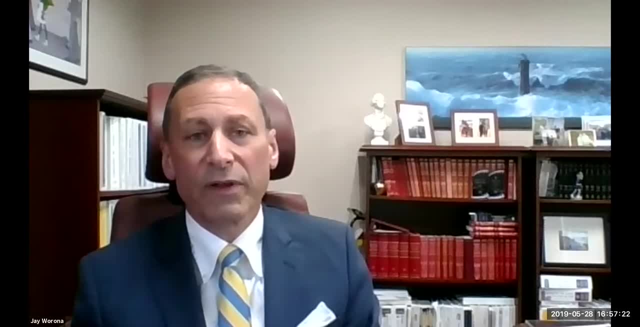 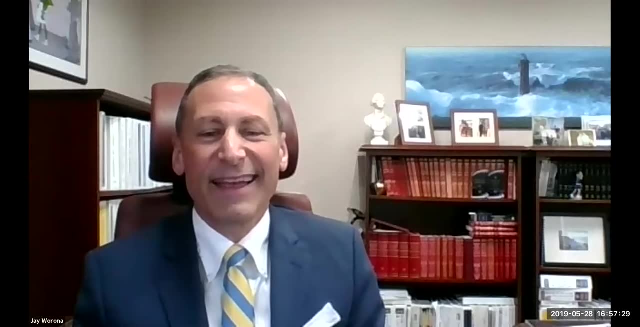 and I think everyone on this on this webinar would agree, hopefully, that when you define the word oh, you are our. it's not just the school district, it's societal right. This is an important aspect of what kids need to be able to achieve in order to be productive citizens, for 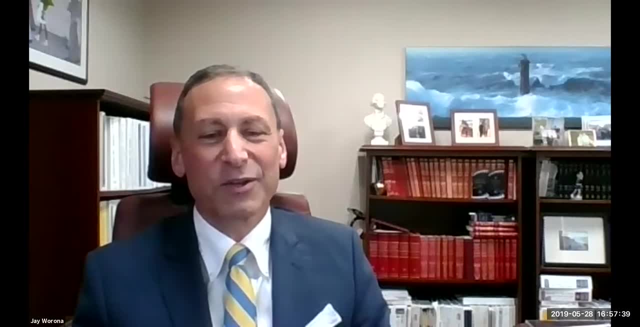 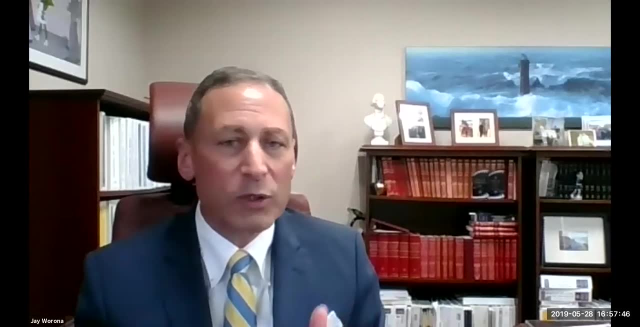 all of us, because they're going to leave school at some point. So this is not just about what schools want, And I think that's what the state uh, misunderstands. They think we're money grubbers. We want just more resources. No, 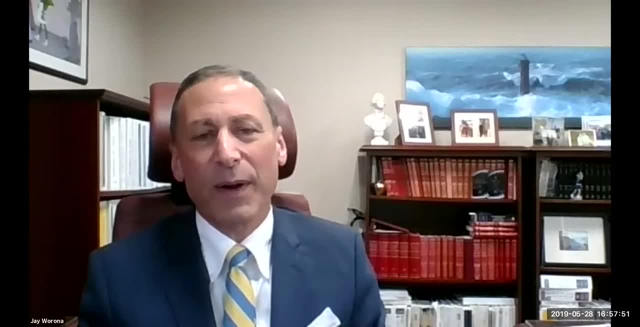 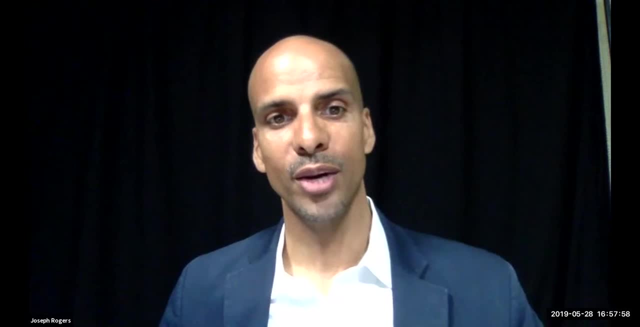 we want to make sure that our kids are able to be as productive as they possibly can. That really is what this is all about. You heard it here first: Um uh, um, it's really about the young people. Uh, one one, one little wrinkle, and then we're going to have to close. It's such 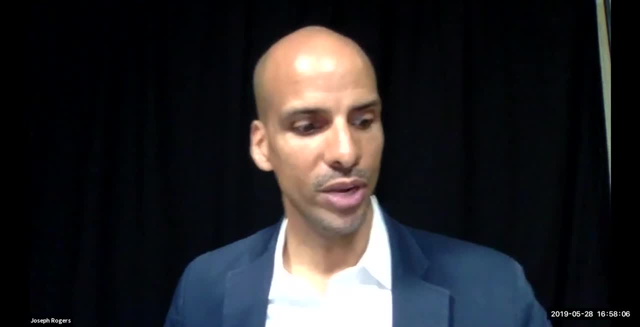 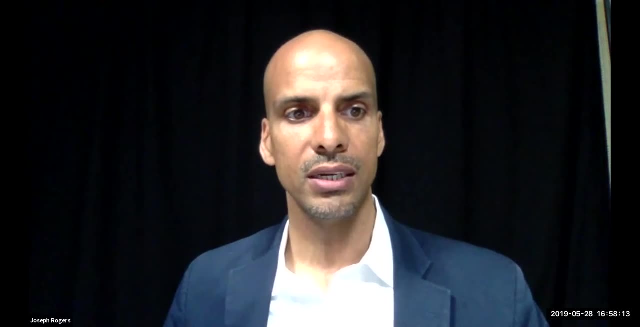 a rich again. I'd love to be able to extend the conversation, Uh, but we are almost at our witching hour, almost at five o'clock, So has just quick question again, Jay. uh, school boards, has school boards done any work? 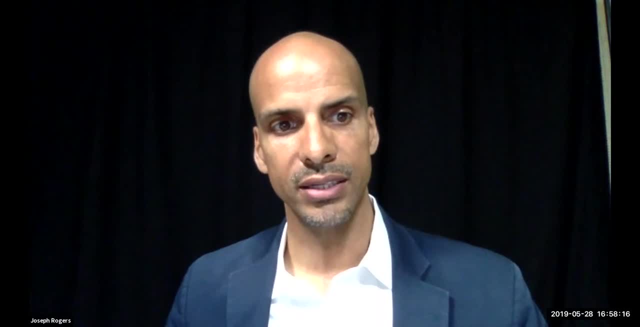 A survey or any research to find out, uh, to the extent to which this these opportunities are already being provided and what the barriers are. Have you all published any reports? And, of course, with the center for educational equity we do some of this research, So we hope this informs. 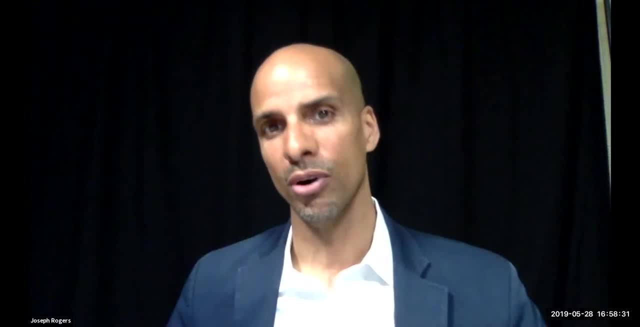 uh, the work, and we certainly like to expand it, but has school boards done any, any, any studies or surveys to understand from its members? uh, you know how, how we're doing in preparing on people. We haven't done that yet, Joe, and you're making me feel guilty. 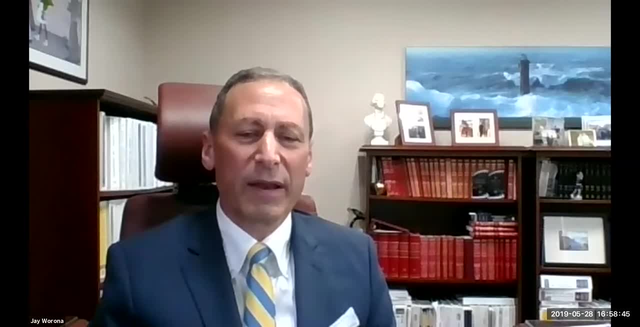 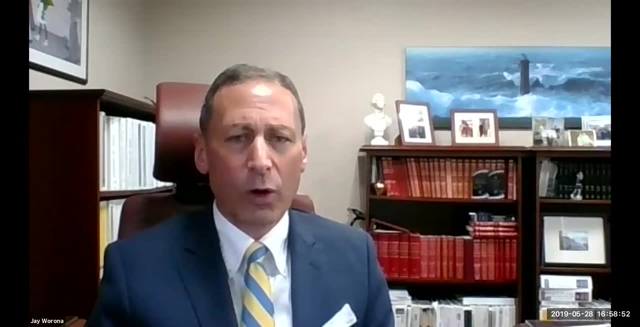 because we need to And we need to work with, along with you and the researchers who have, um, all of this stuff at their fingertips. What we have done is we've attempted to, to, to work with school districts, um, with respect to the opportunities that are out there, but, unfortunately, to acquire those. 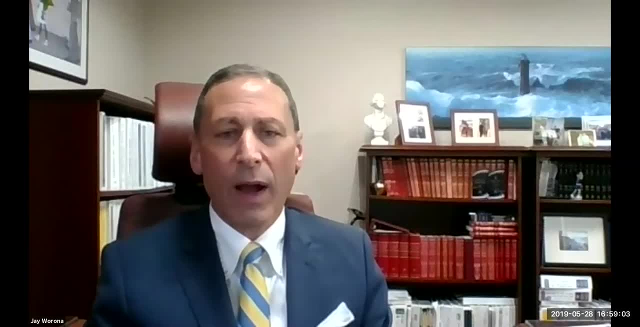 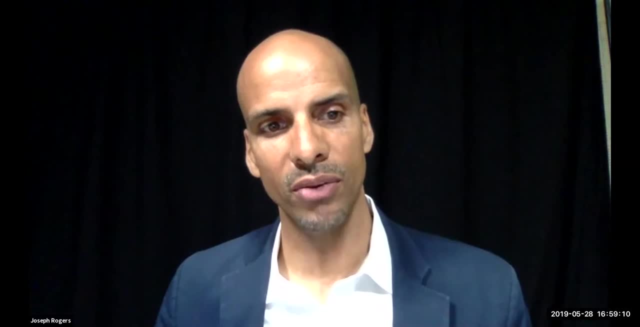 opportunities like moot court, competitions, et cetera. it requires districts to have the resources to be able to provide those opportunities. Okay, good Thanks, Jay. And then just finally, I just want to make sure we underscore here This: 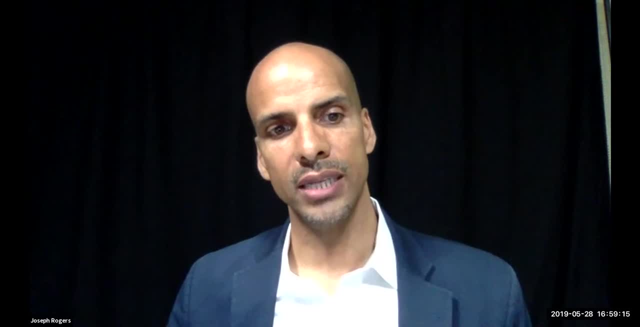 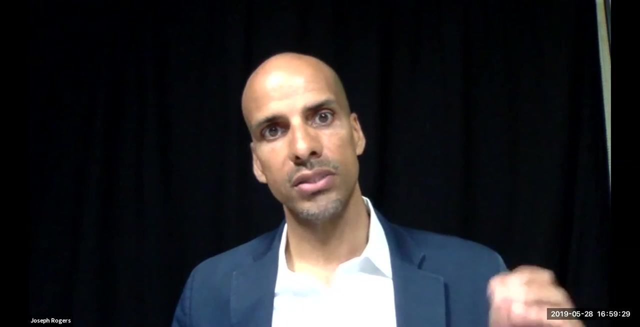 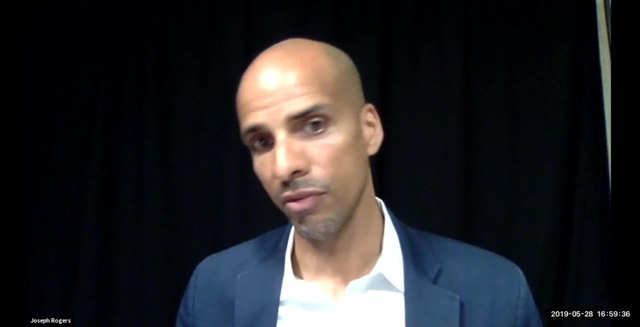 is a constitutional responsibility- Okay, That is really. it's incumbent upon, It's a responsibility of our state government to make sure that these, uh, all, all young people have access to a sufficient, adequate level of civic learning opportunities. So you know, school boards, educator, teachers, students are nonprofit partners. youth development specialists, superintendents, parents and other sort of stakeholders all have a role to play. 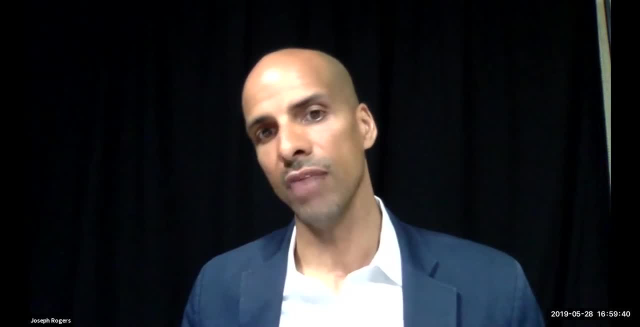 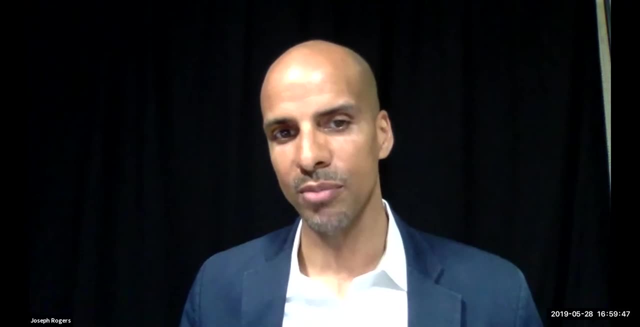 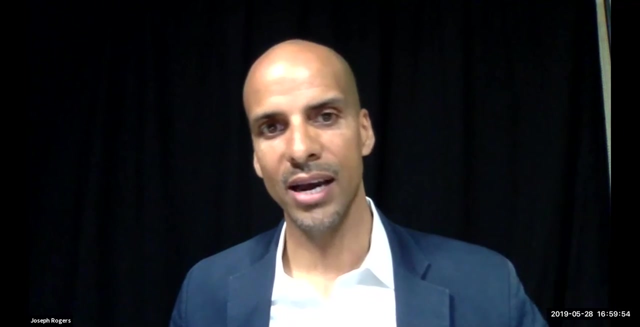 But that constitutional responsibility is really the responsibility of our state government. that includes our state policymakers. So we of course have to be successful And we have to work hard in our state. that includes the legislature and includes the governor and, uh, collectively, we have to make sure that we're all doing Our parts. 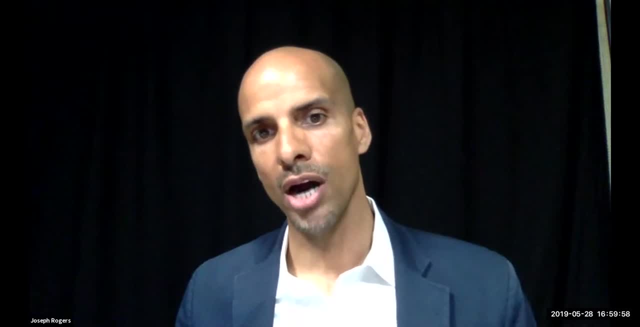 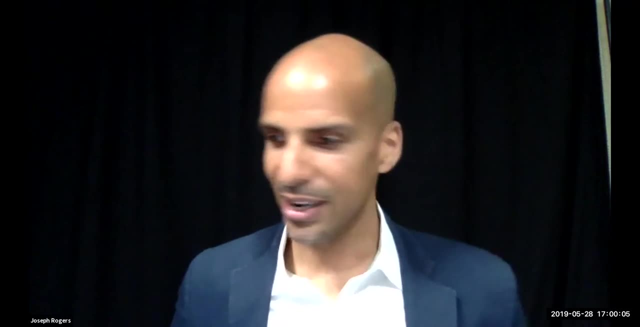 And, uh, we'll come back to this issue of accountability and figure out what it looks like, not to chastise and punish folks, but really to make sure that we're tracking, We're monitoring access, these opportunities and ultimately, they're being delivered to all students per the state constitution. 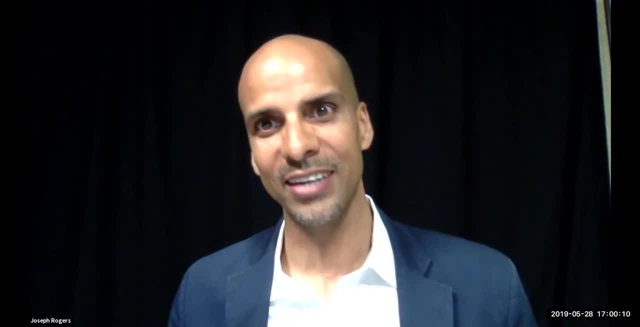 I want to thank, uh, as we close, our panelists again for, uh, their phenomenal contributions here, for enlightening us and raising questions here. Uh, we'll be back in a couple of minutes. if there's any further questions, let's get to that. 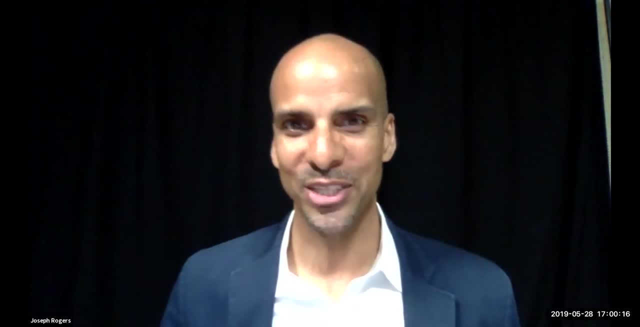 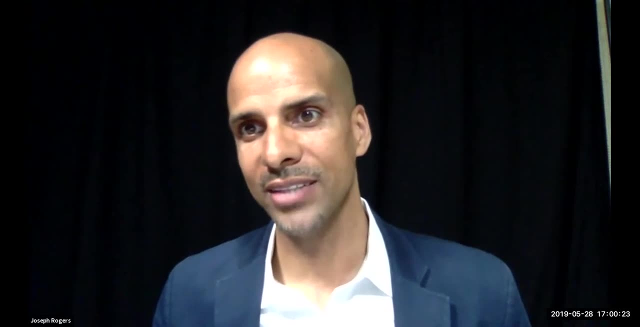 Please join me everyone. I know we can't hear you, but join me in thanking anyway Jay Warrona, Diana Vasquez, Leah Antwala, Hamza Noor and Tiffany Allen Hubbard. Thank you so much for taking your time to inform the discussion and inform the decision making.